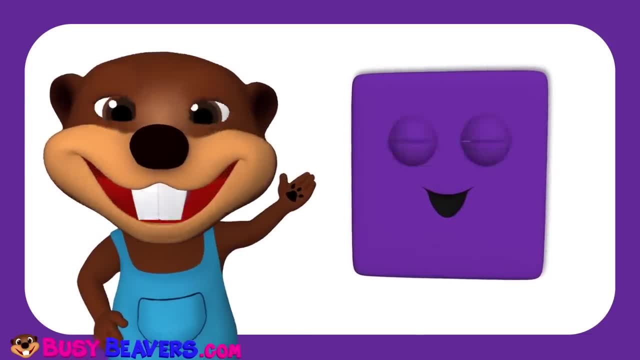 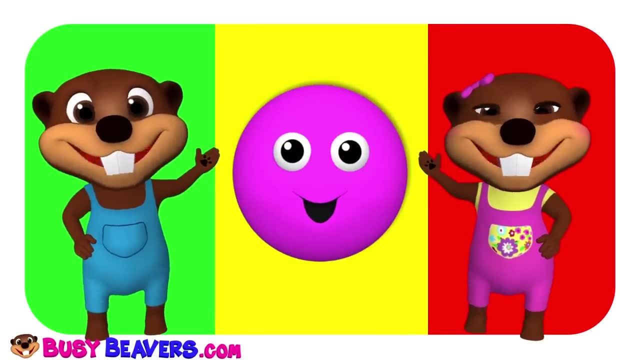 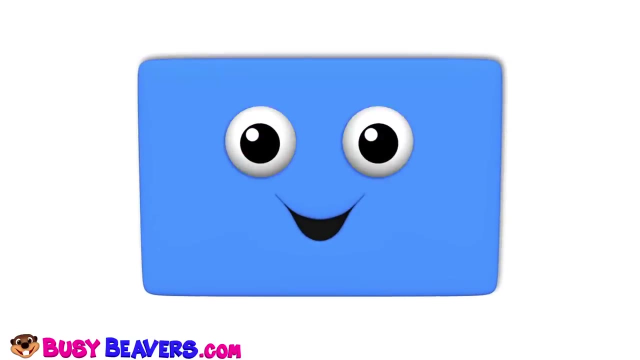 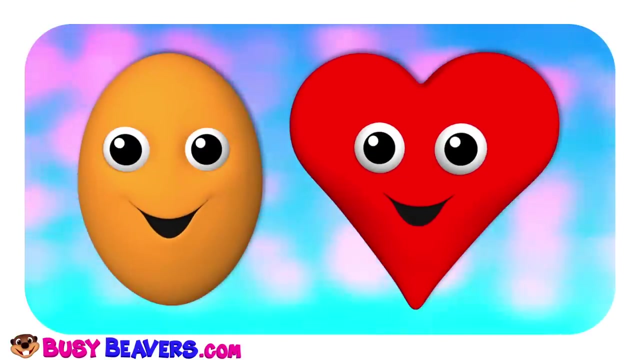 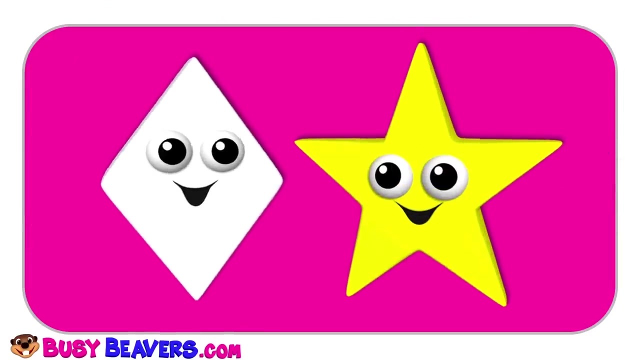 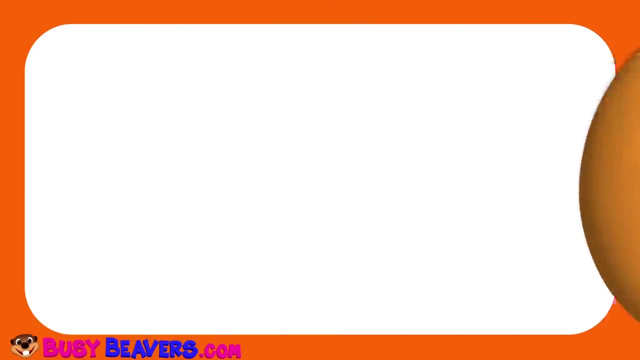 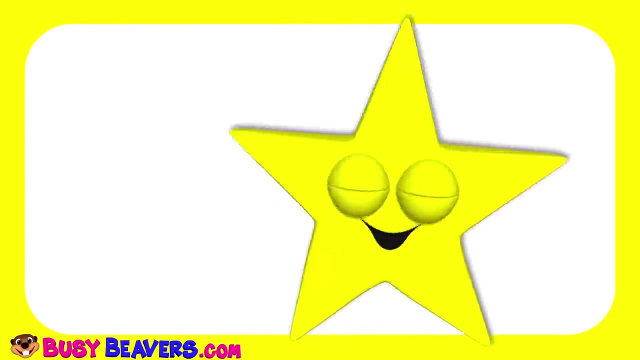 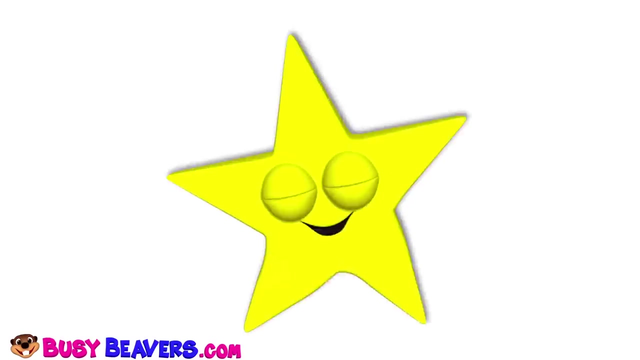 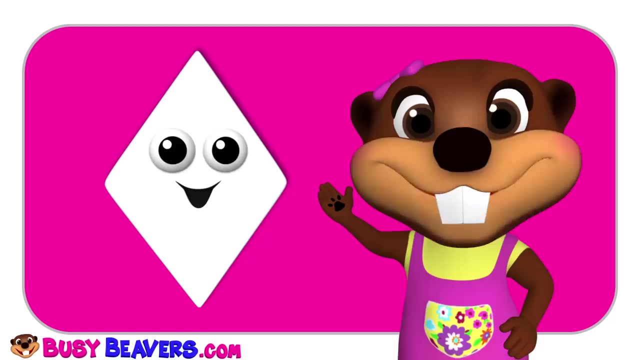 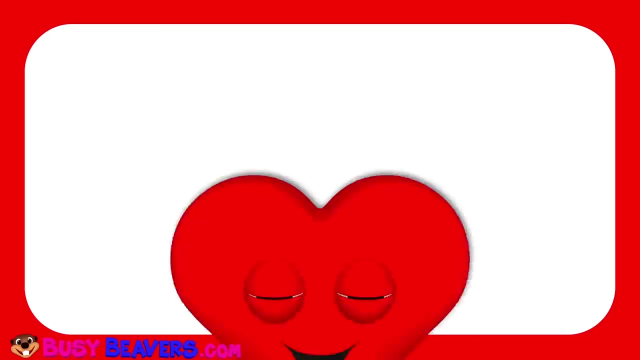 Circle Square, Triangle, Rectangle- rectangle. circle square, triangle, rectangle. Oval heart- diamond star. Oval heart- diamond star. Oval heart- diamond star Star. Oval oval heart heart- diamond, diamond star. 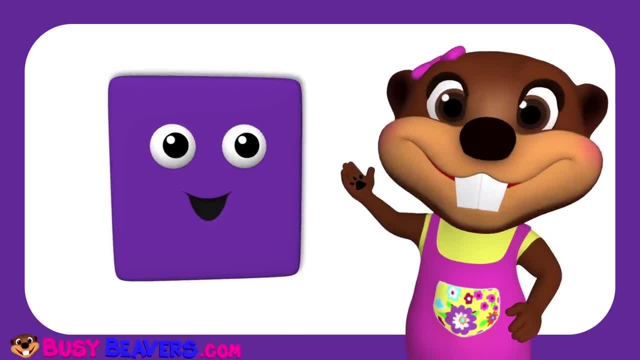 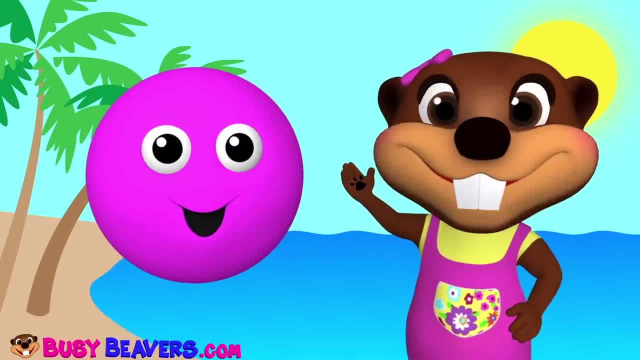 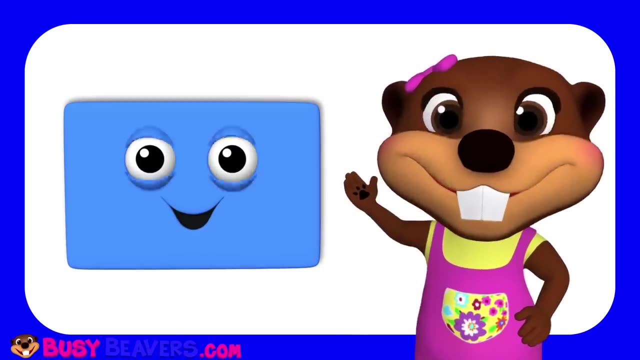 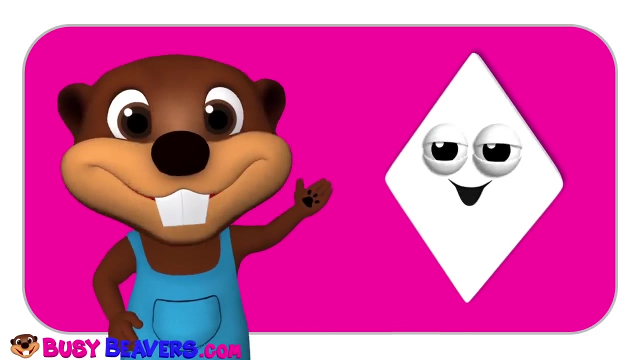 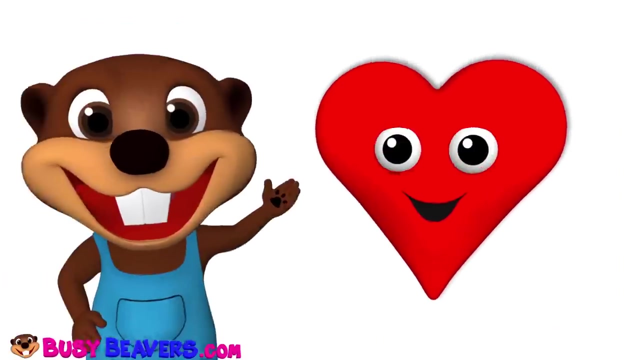 Circle Square, triangle, rectangle, circle, circle square, square, triangle, triangle, rectangle. Oval heart, diamond star. Oval oval heart. Rectangle round. diamond, Oval round. diamond, Oval thing. oval, oval. 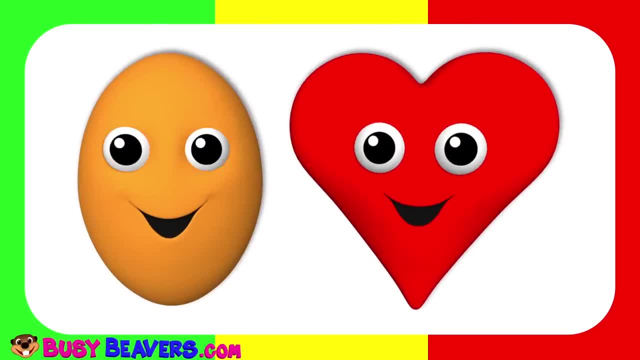 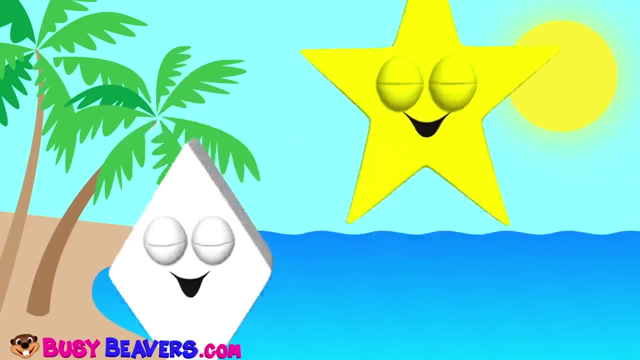 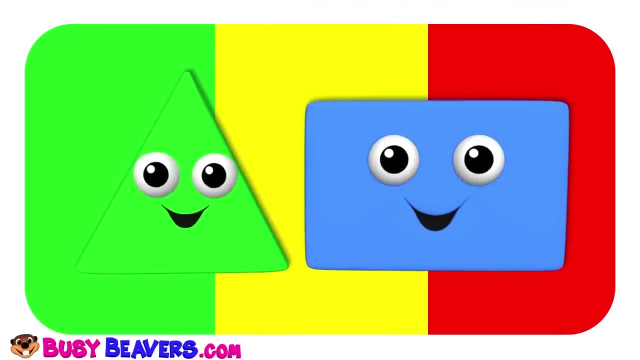 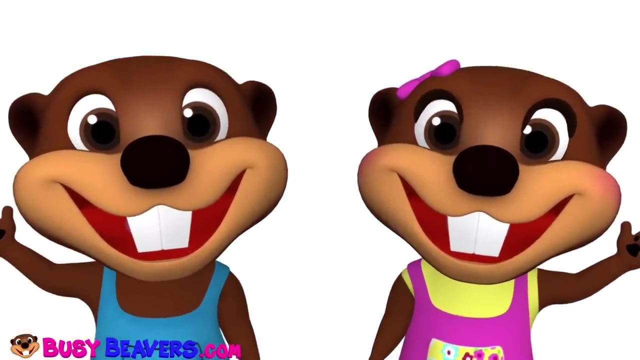 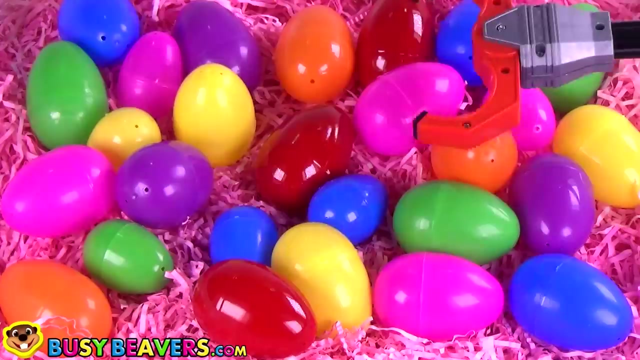 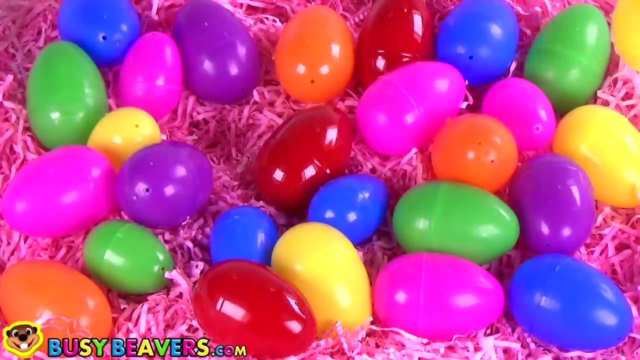 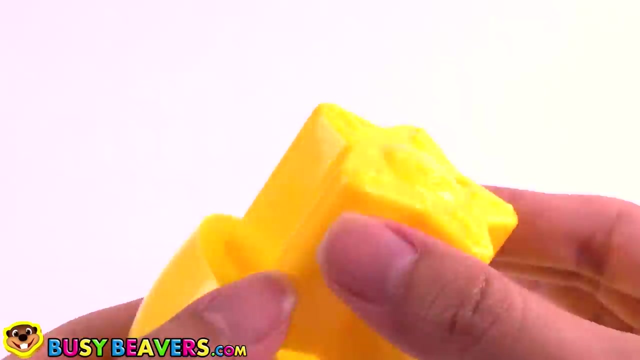 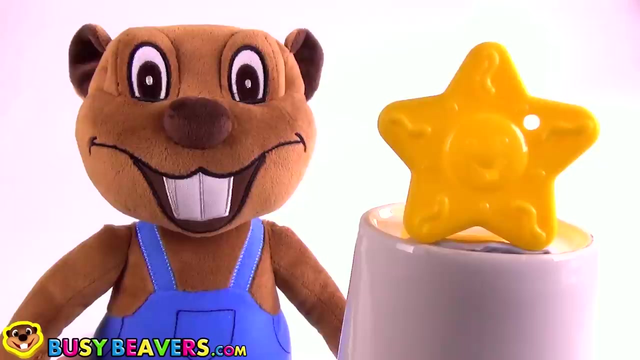 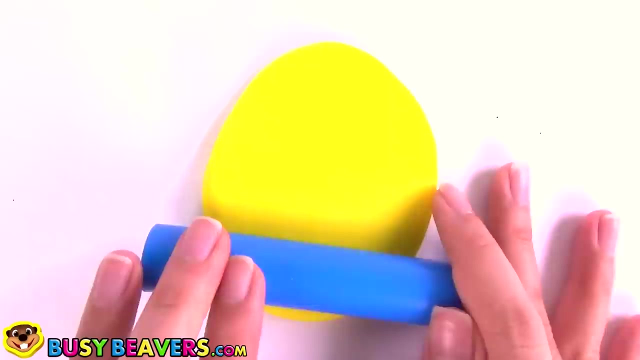 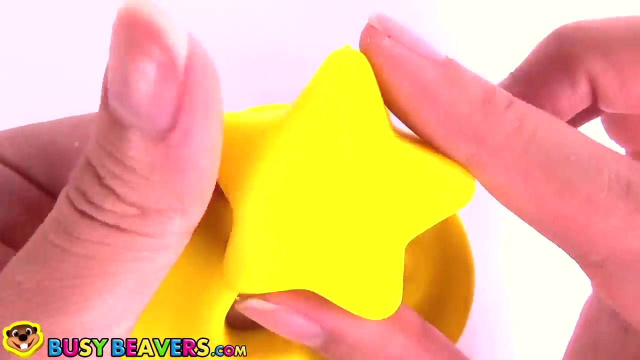 Rectangle, rectangle, triangle, diamond, diamond star. square triangle, circle, space, space, space c. square circle circle, square rectangle, Tomato Shapes, Surprise, Yellow Sky, Yellow Star, Yellow star. 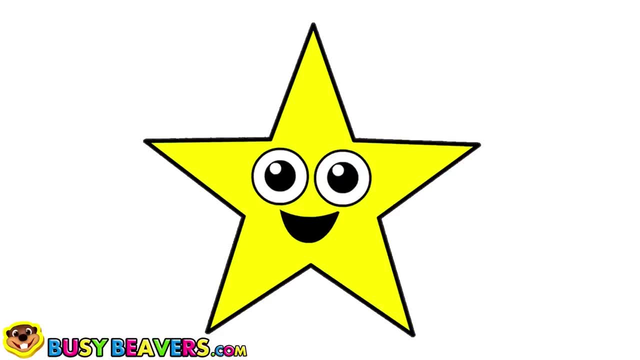 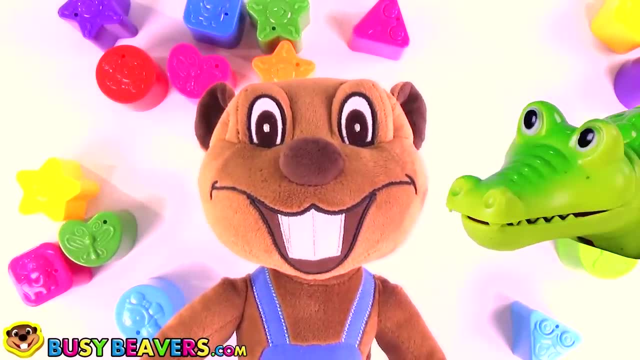 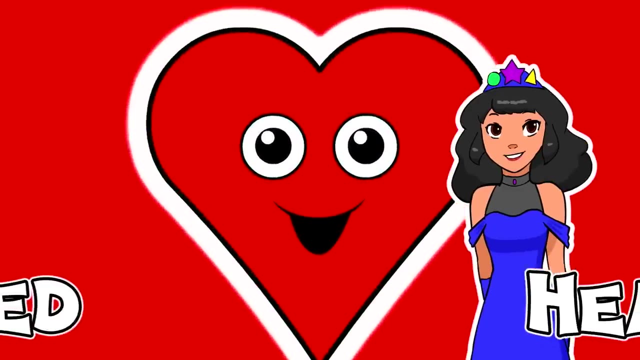 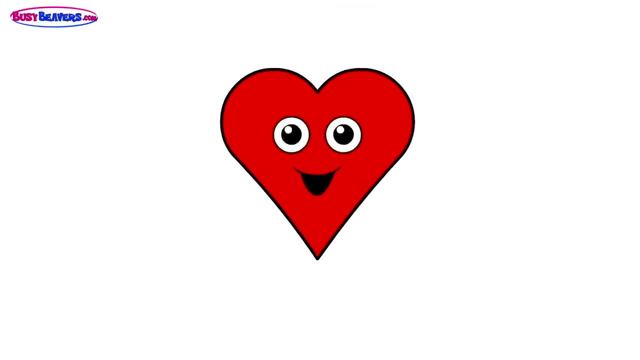 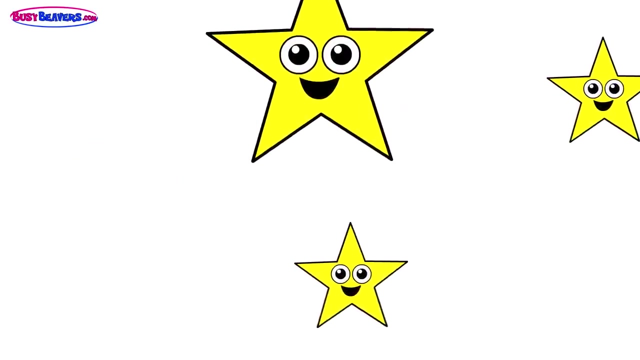 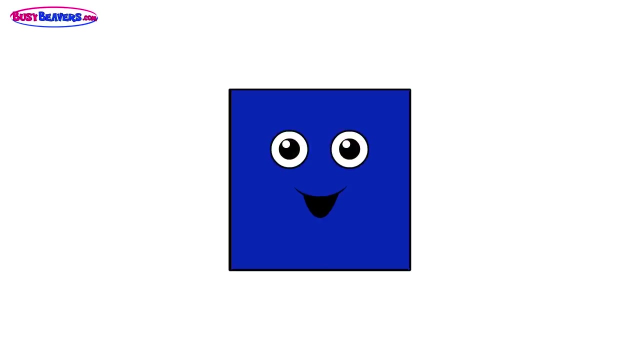 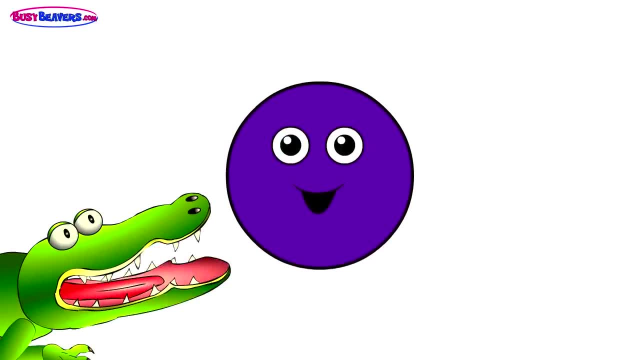 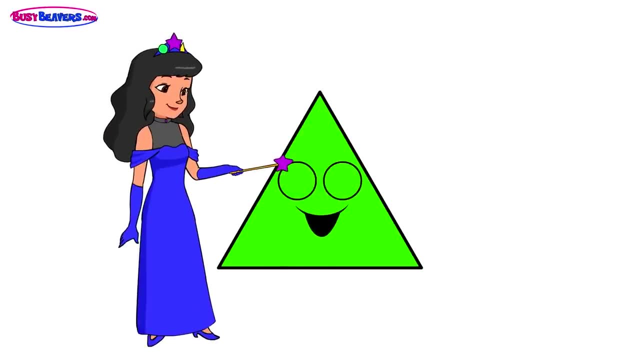 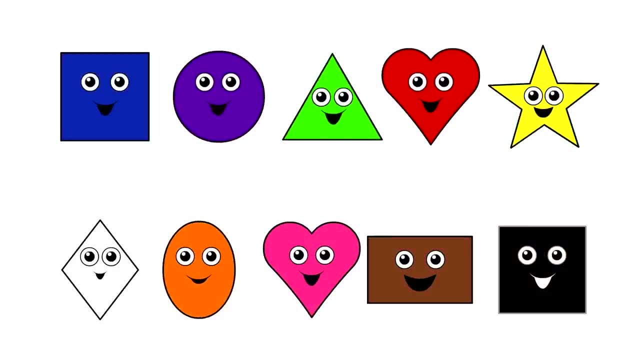 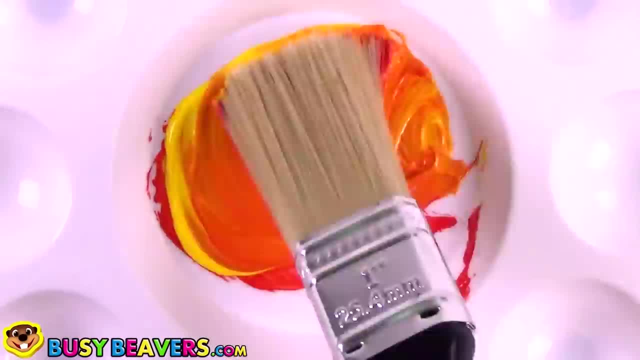 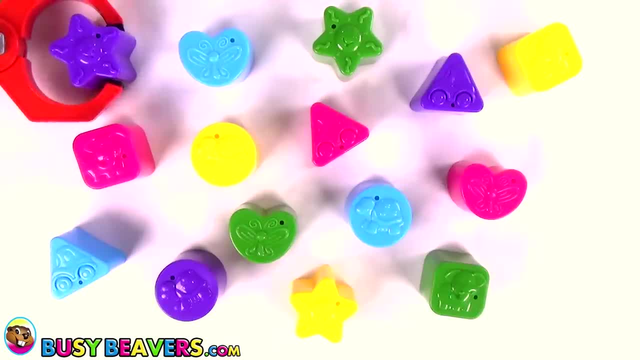 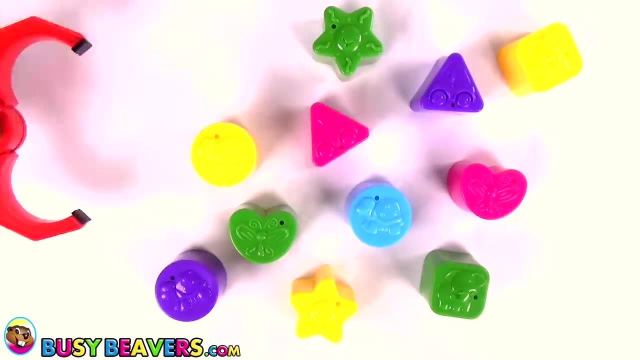 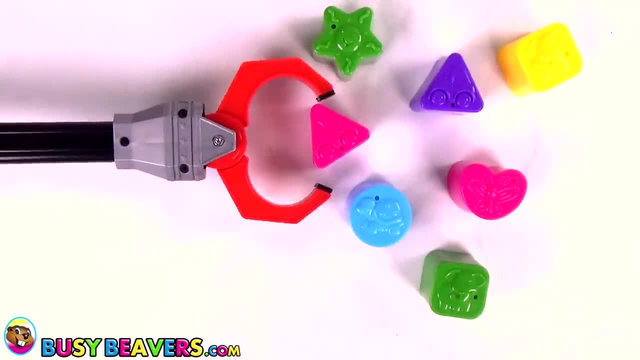 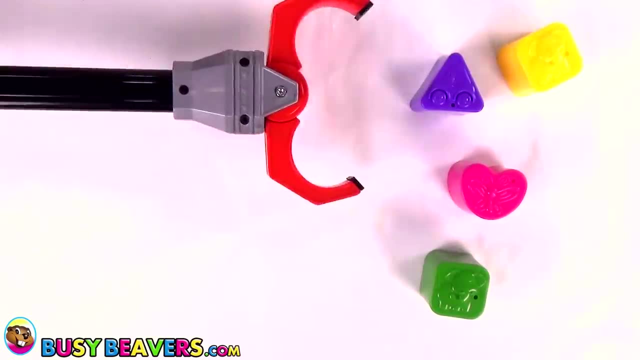 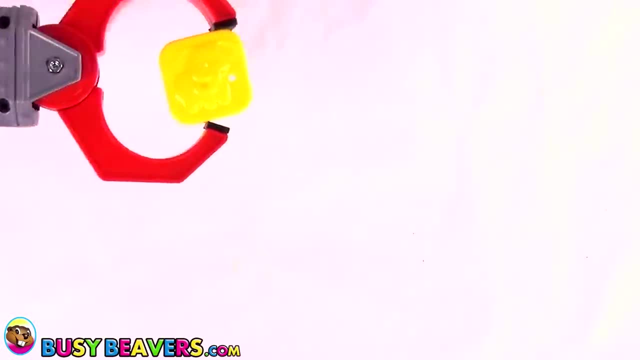 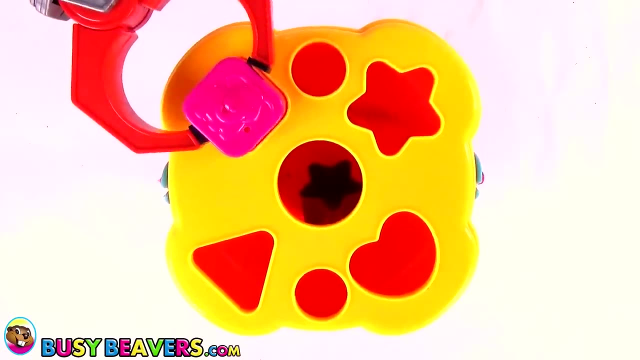 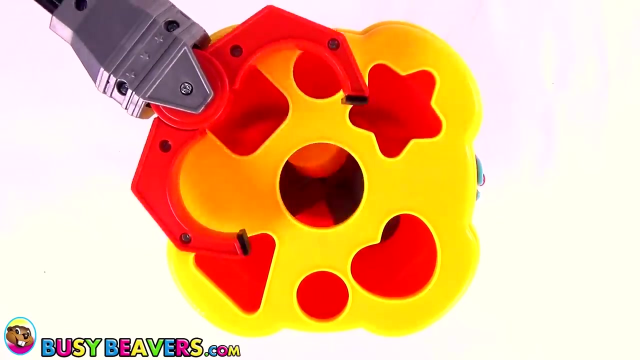 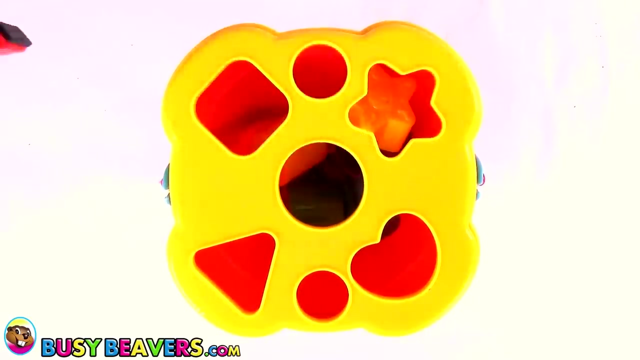 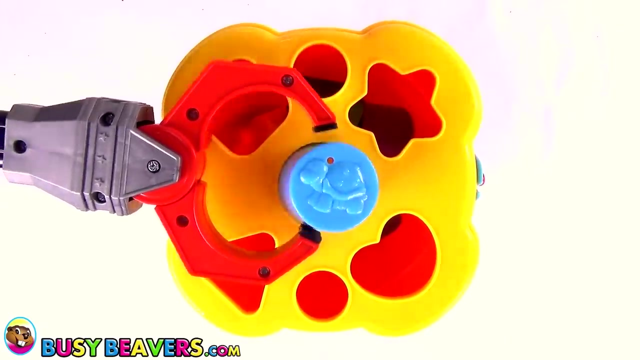 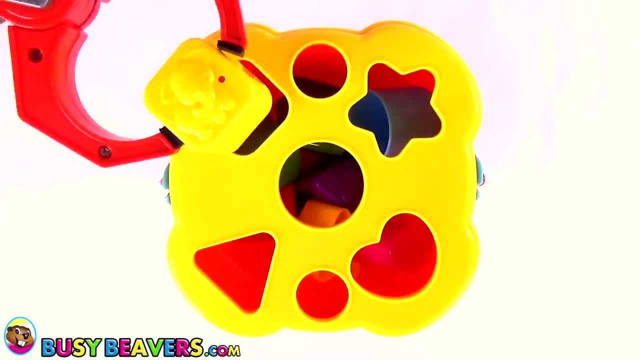 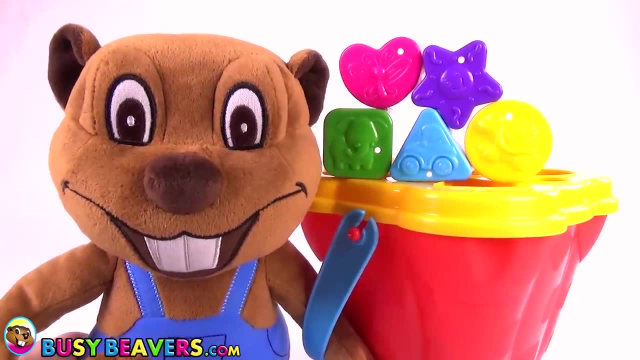 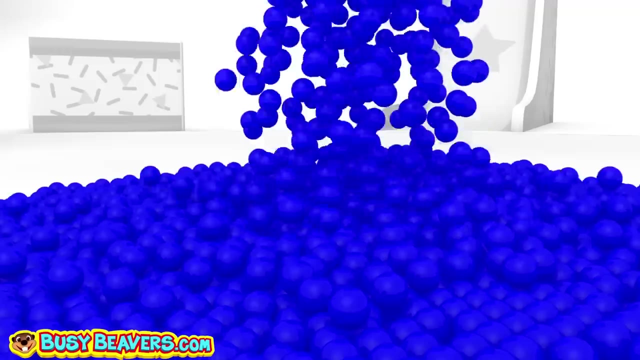 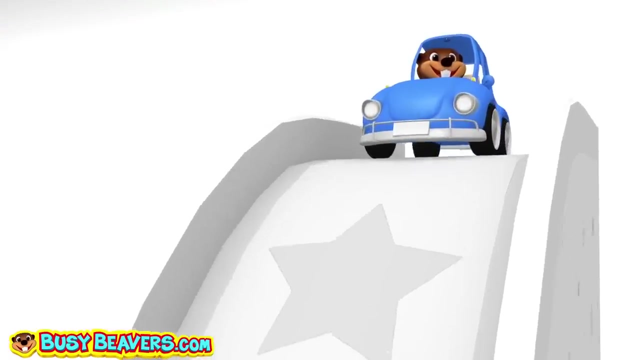 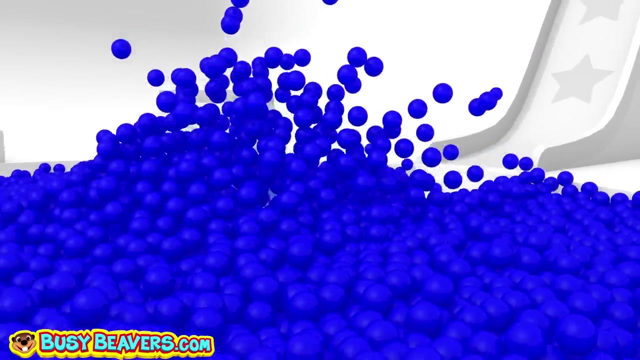 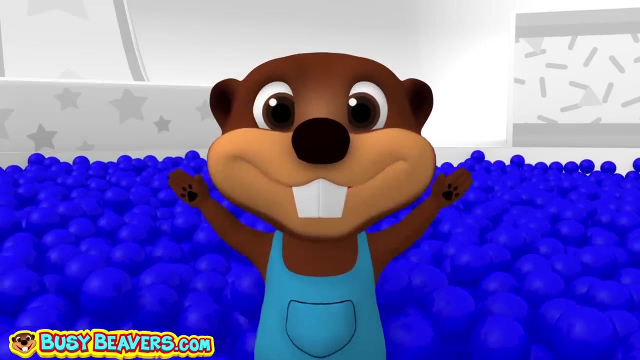 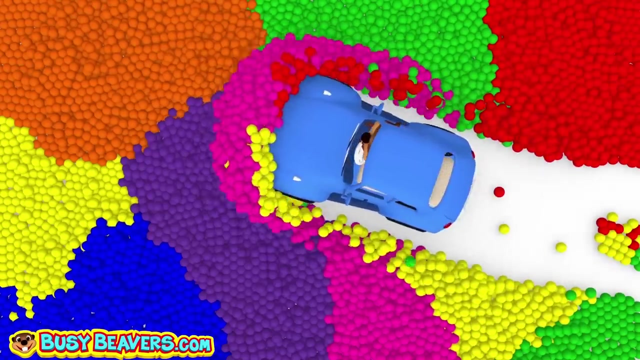 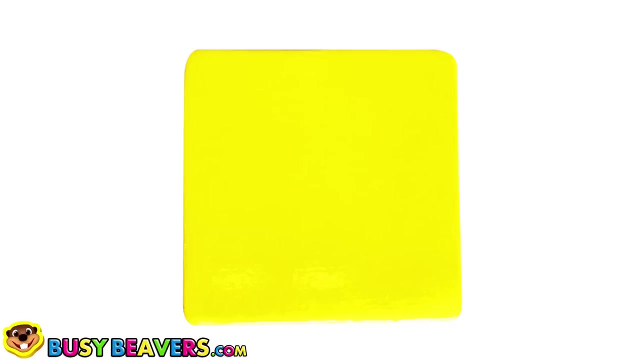 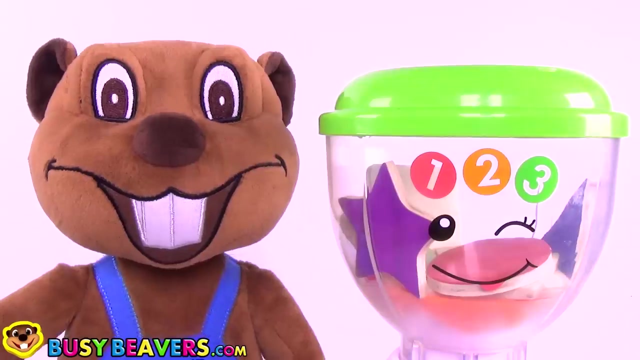 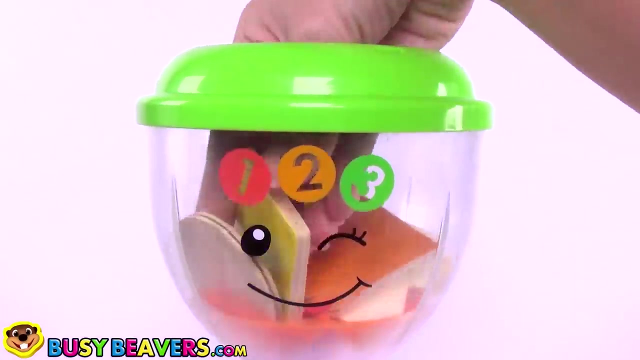 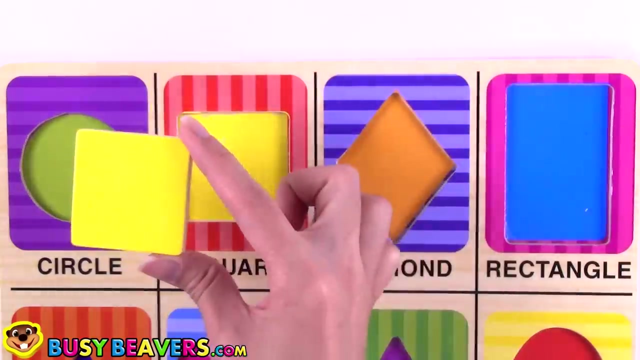 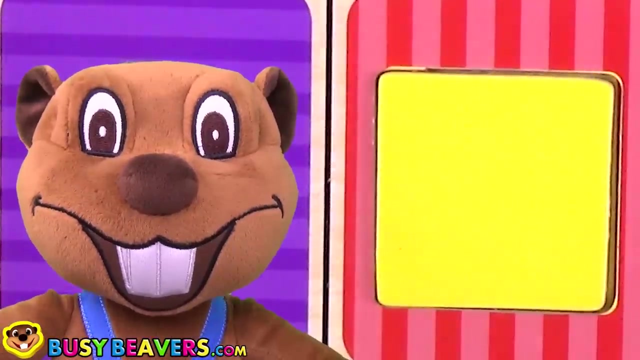 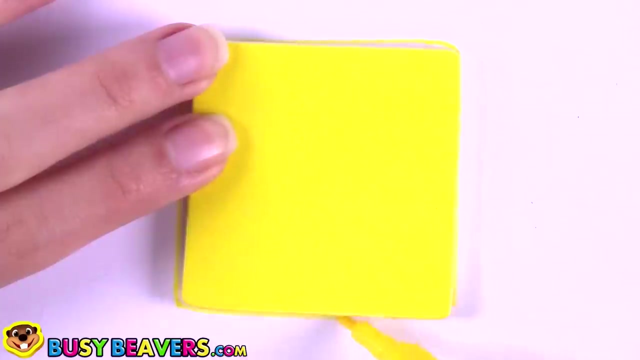 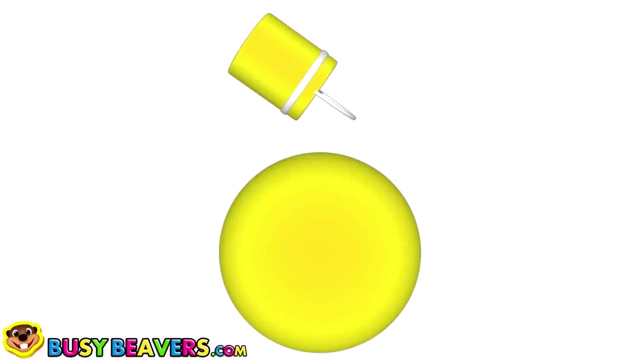 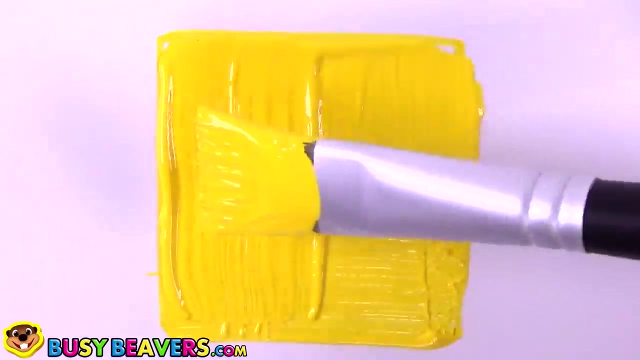 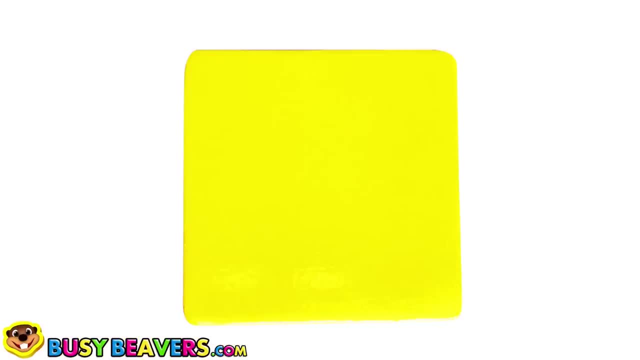 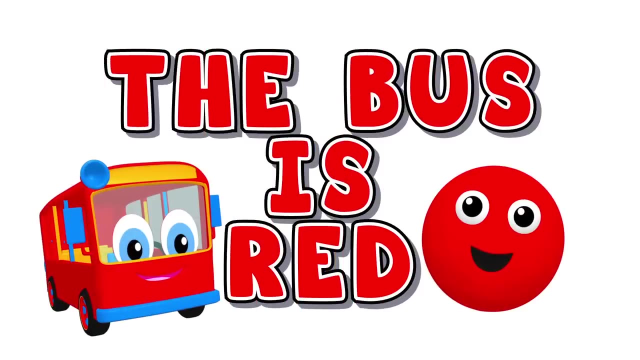 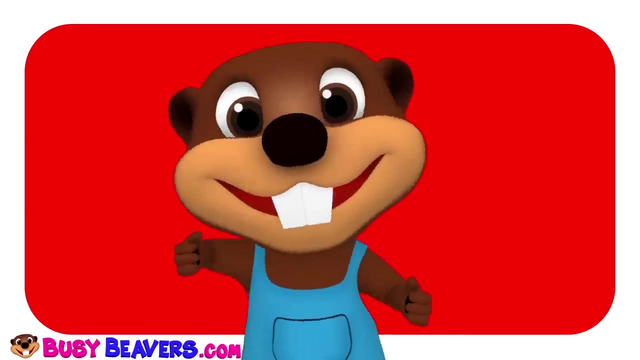 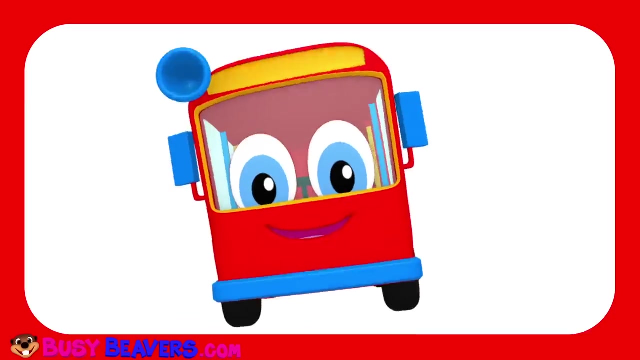 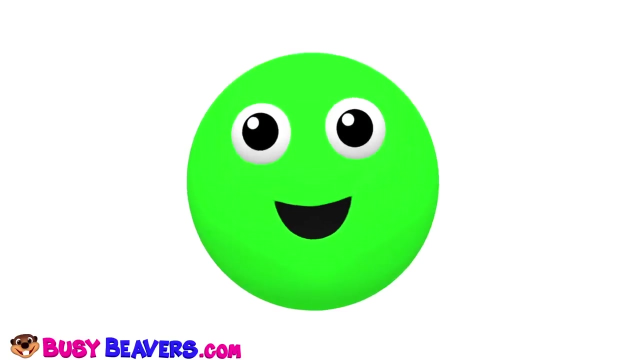 Yellow square. Yellow square, Red red the bus is red, Red, red. the bus is red, Red red. the bus is red. The bus is red, red, red, Green, Green, Green, Green Green. 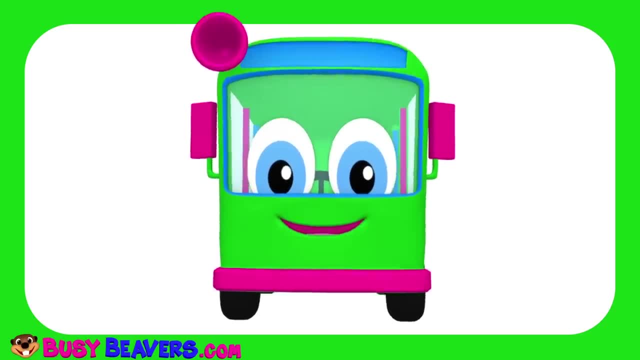 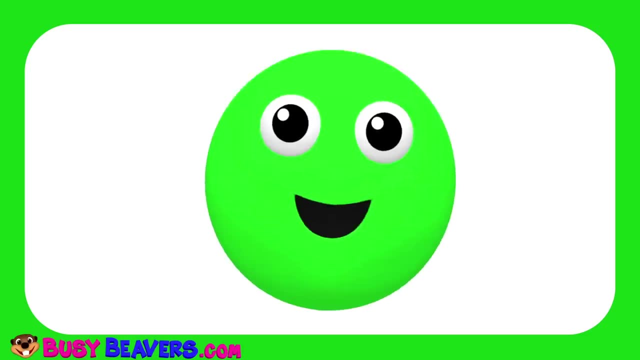 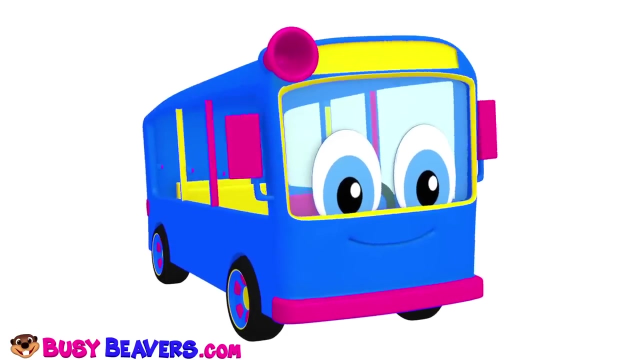 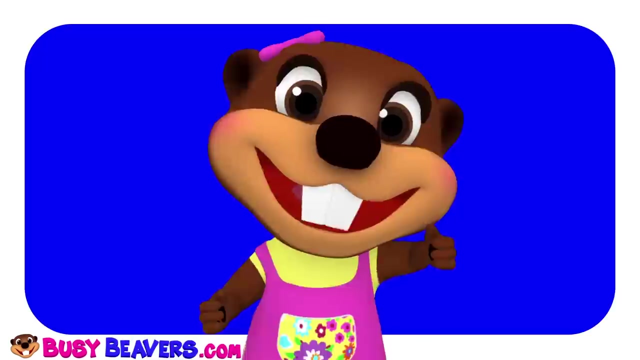 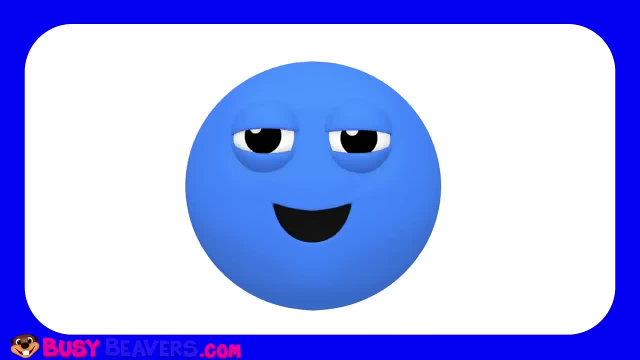 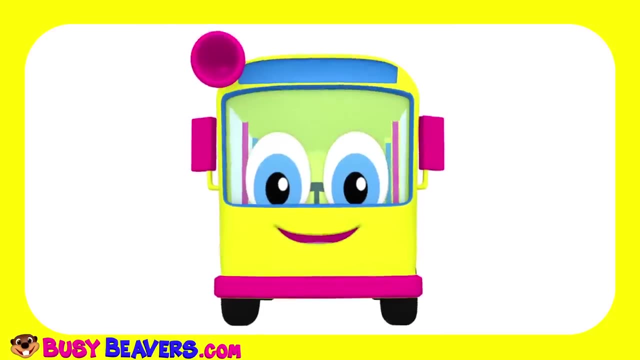 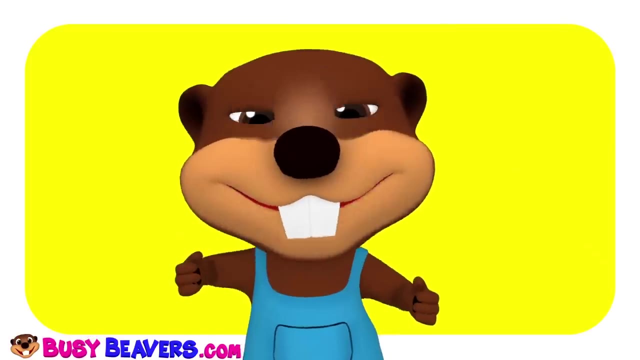 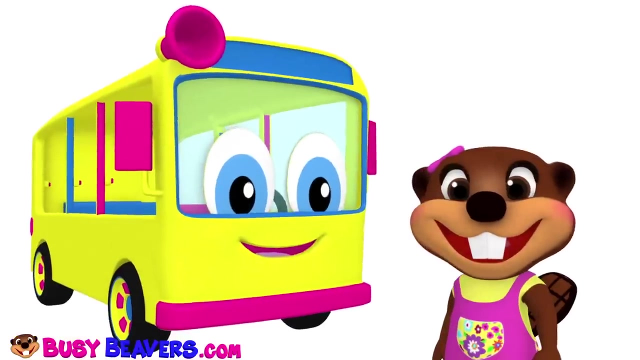 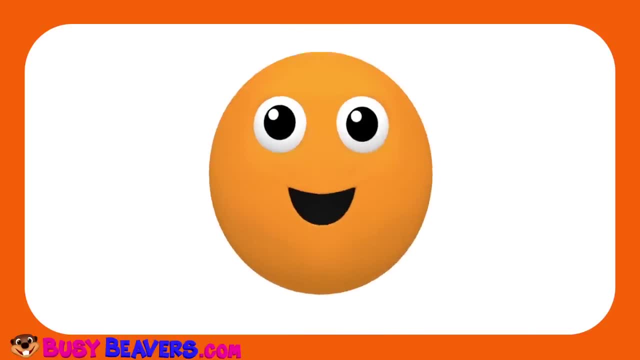 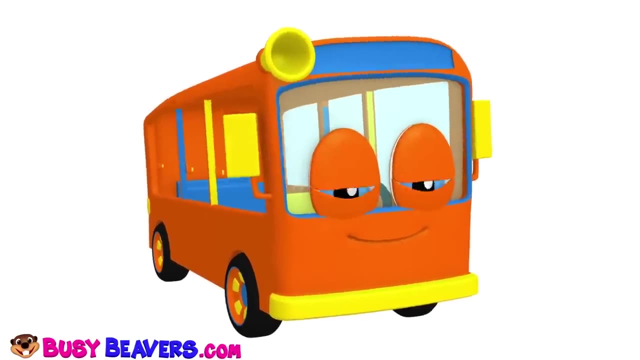 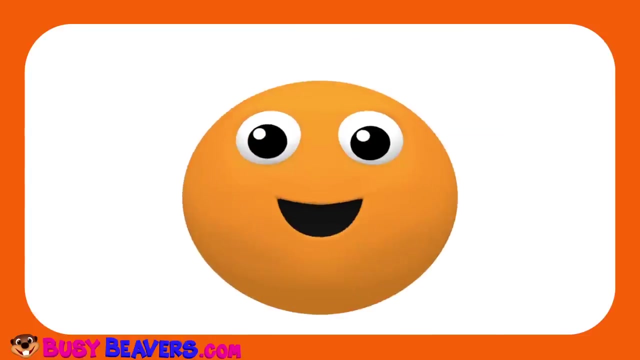 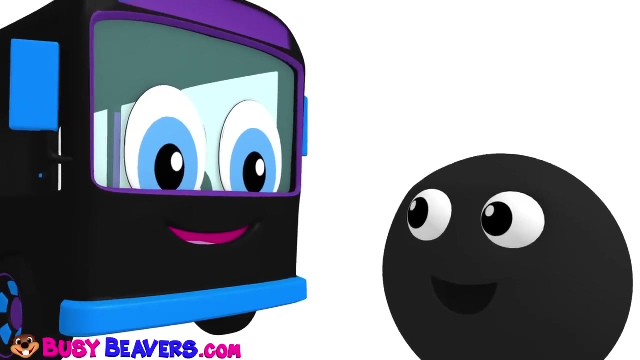 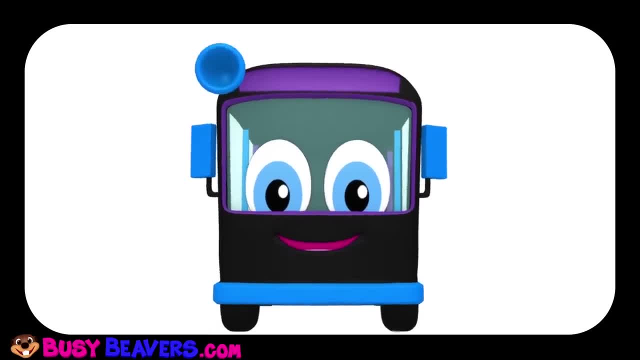 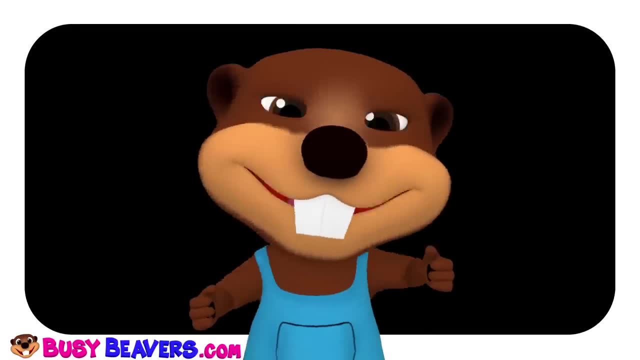 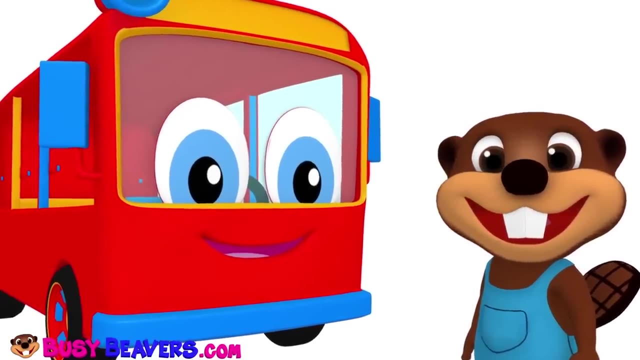 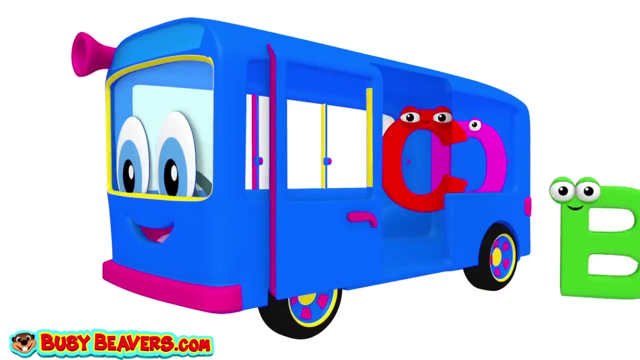 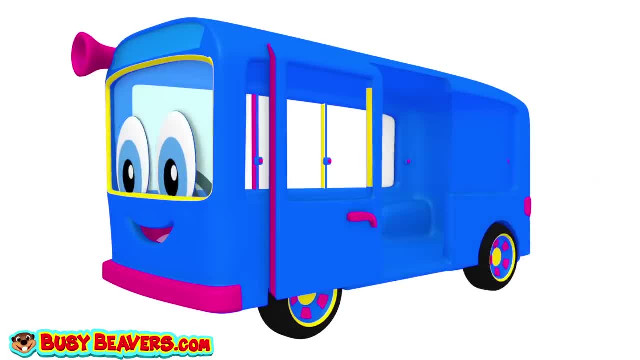 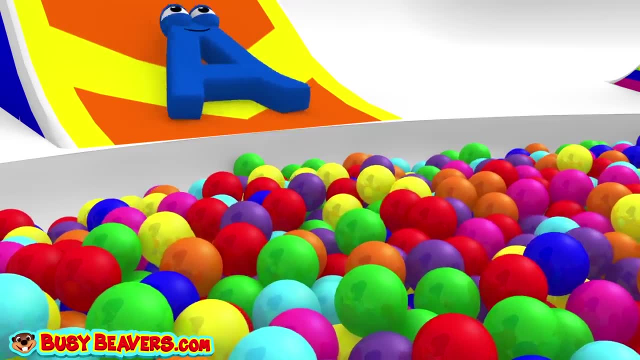 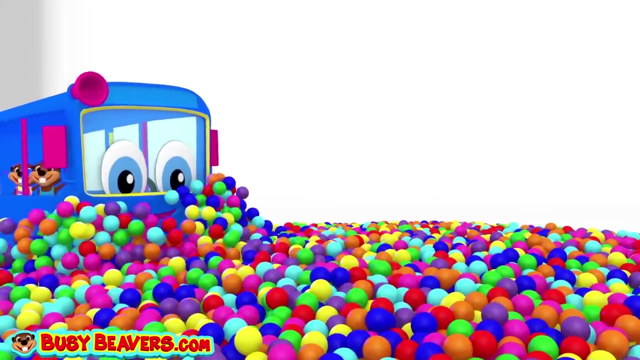 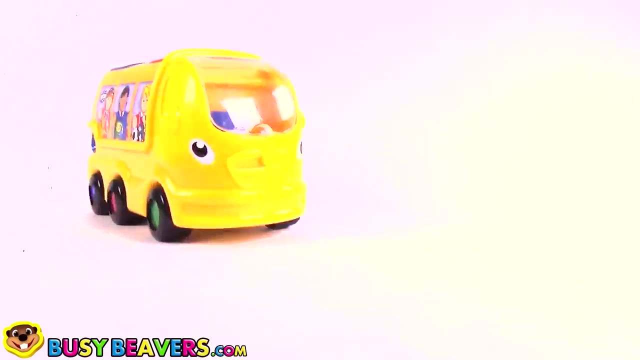 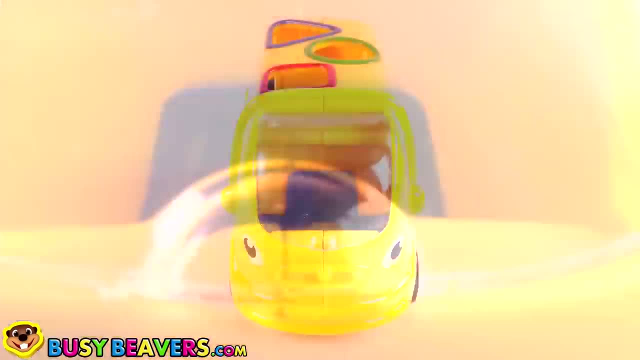 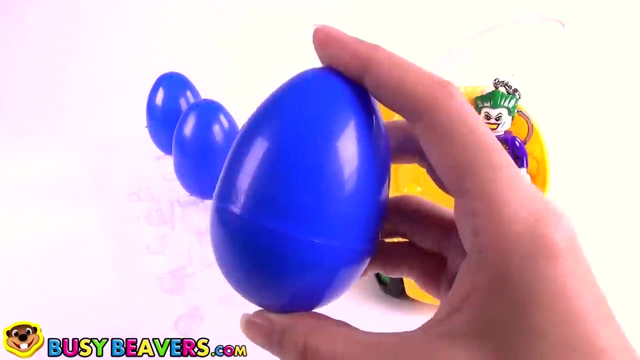 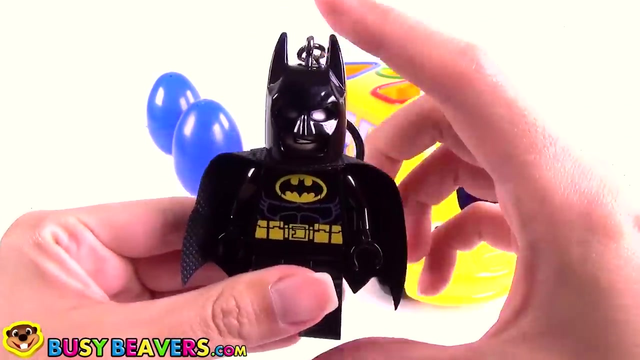 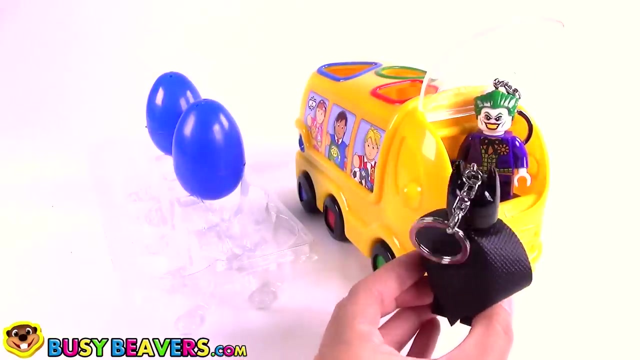 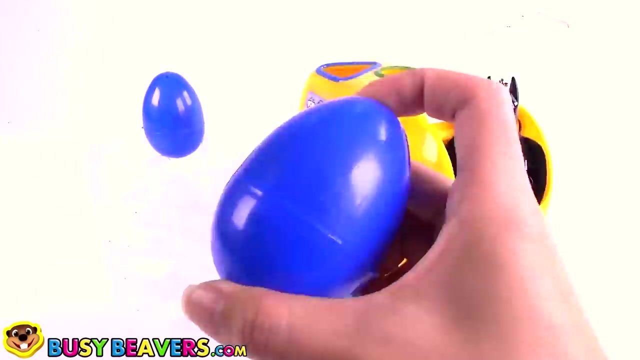 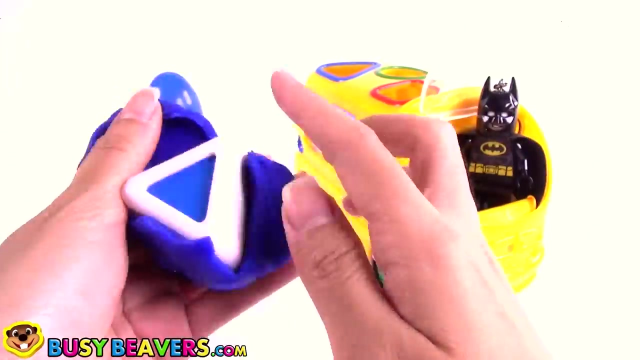 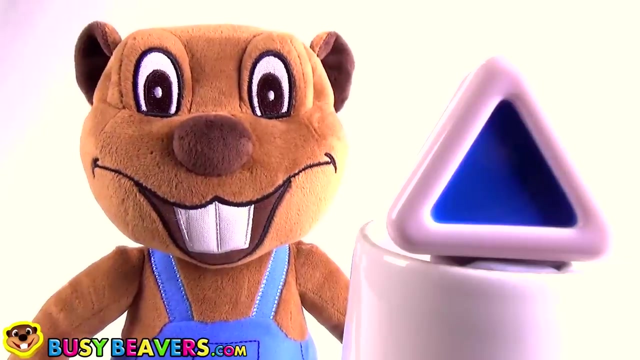 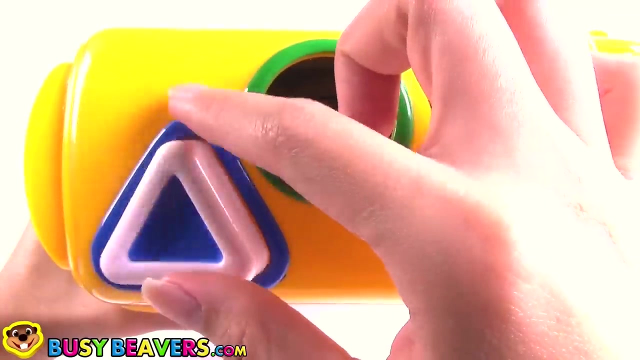 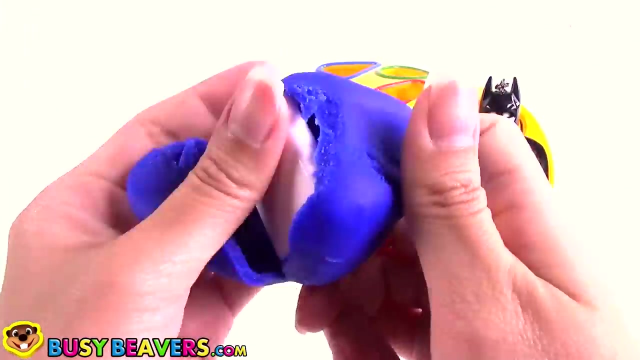 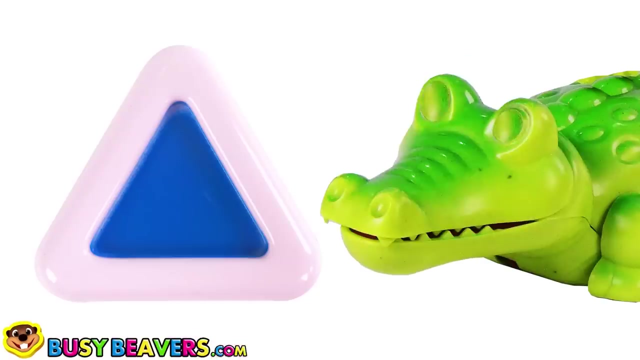 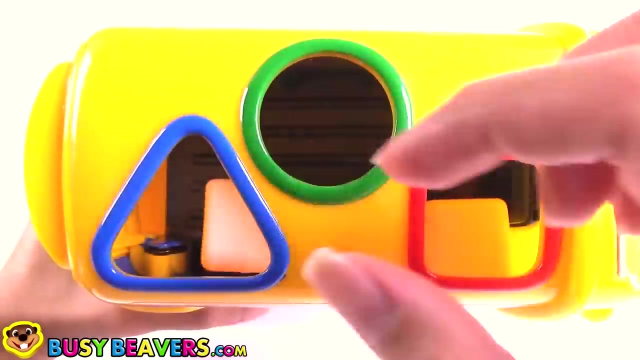 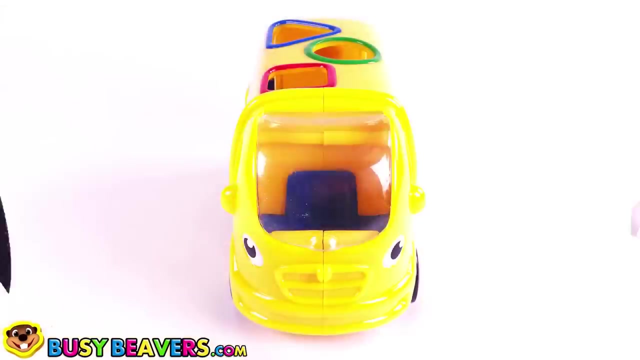 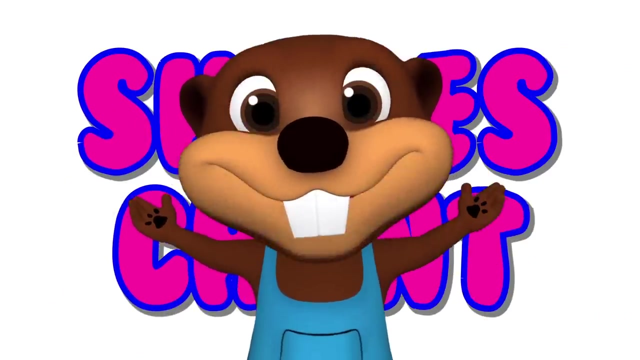 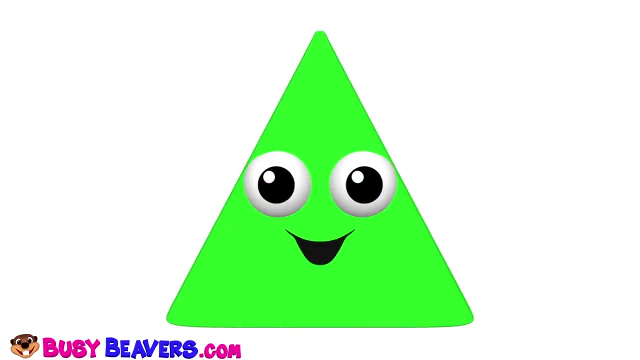 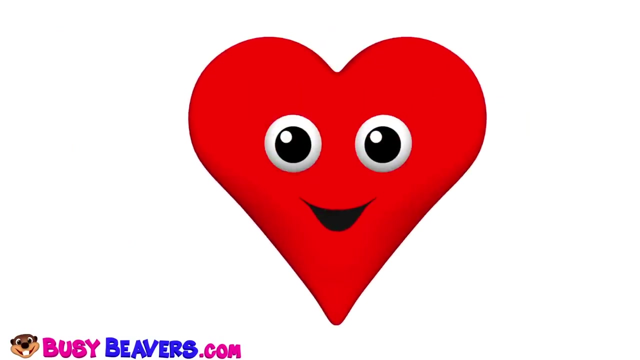 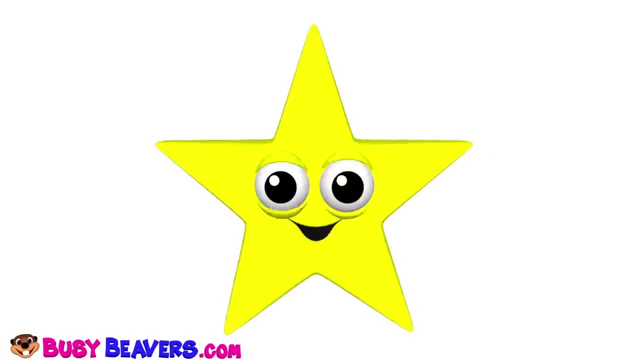 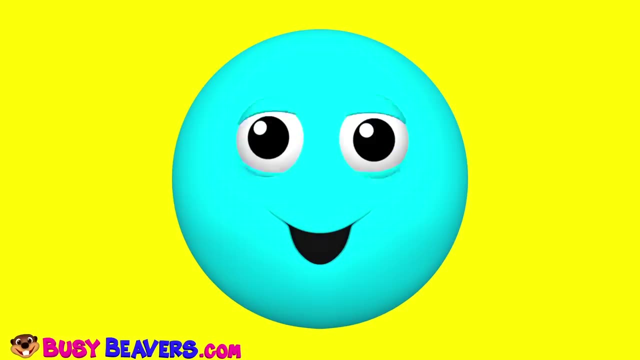 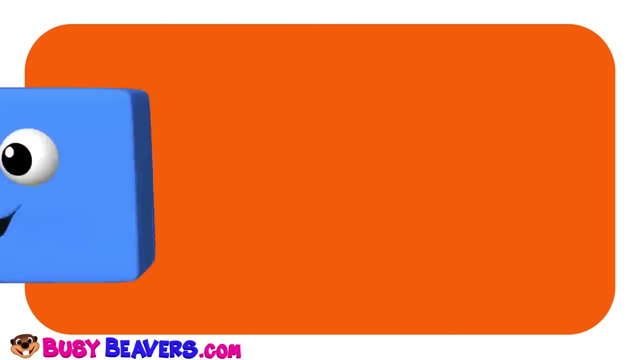 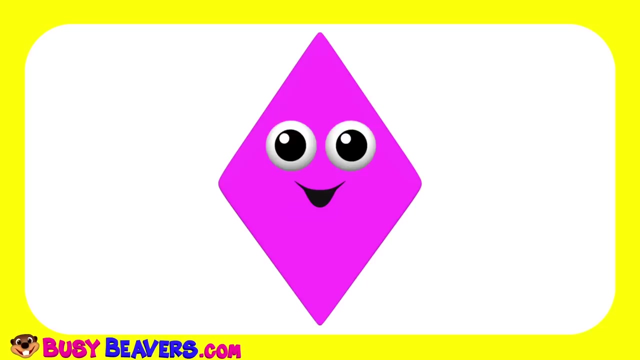 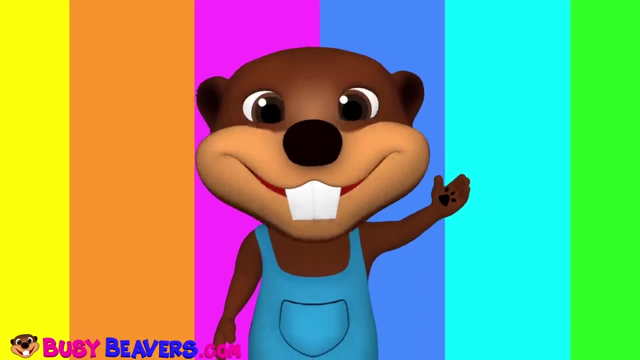 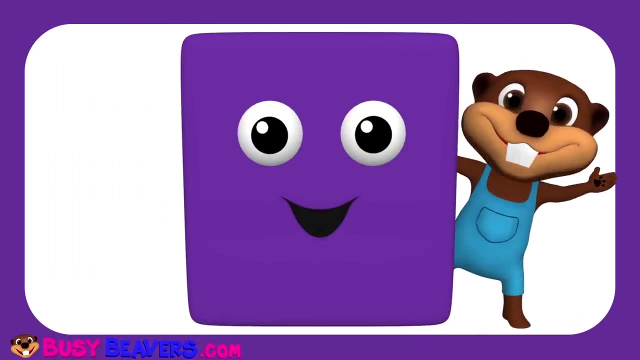 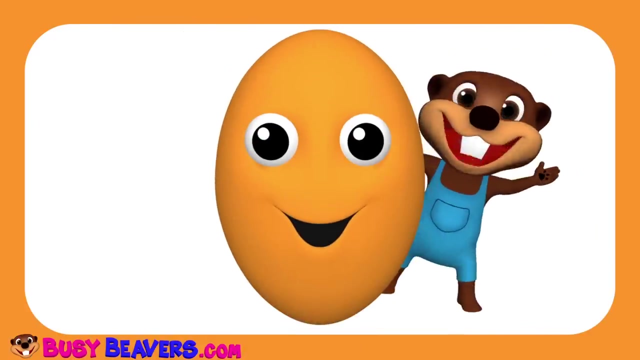 Diamond Star Repeat after me, this time: Circle Square, Triangle, Rectangle, Oval Heart, Diamond Star. Let's be really quiet this time: Circle, Circle, Square, Triangle, Rectangle, Rectangle, Oval Heart, Diamond. 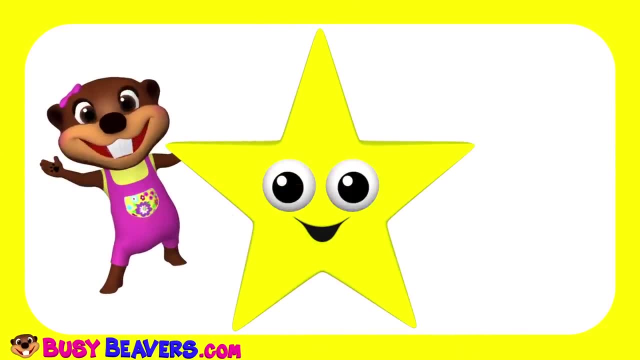 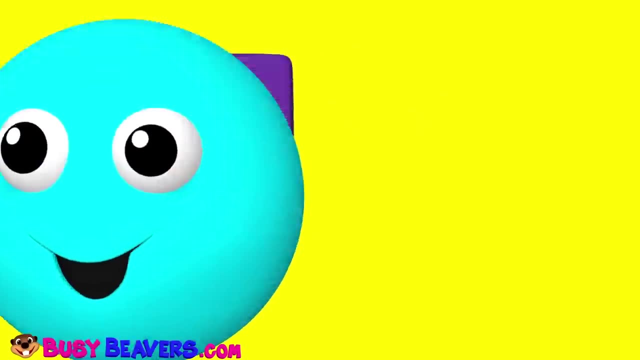 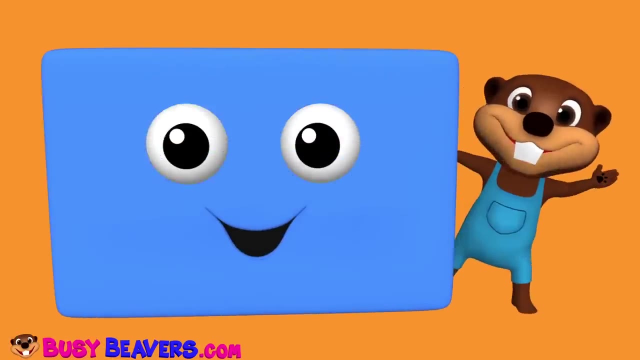 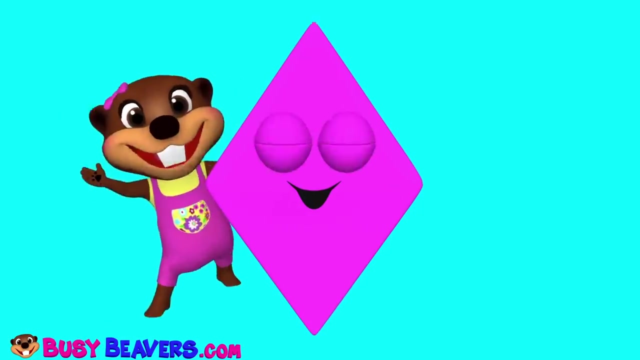 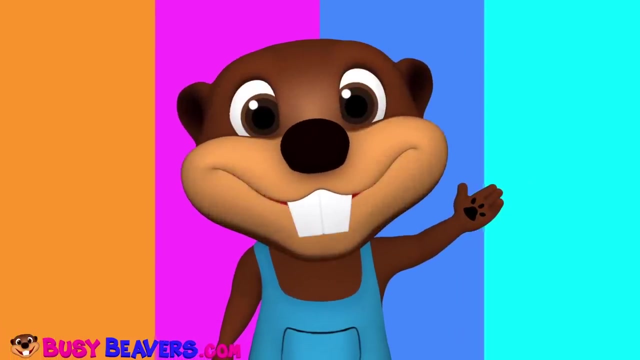 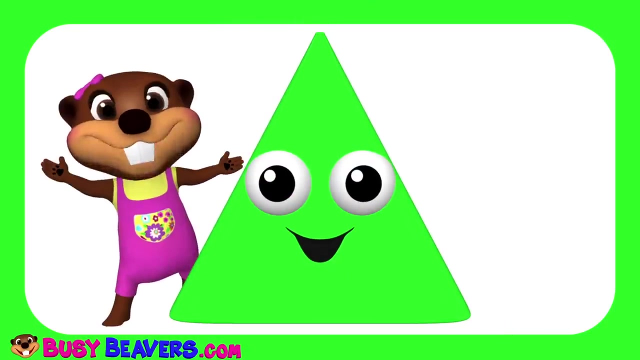 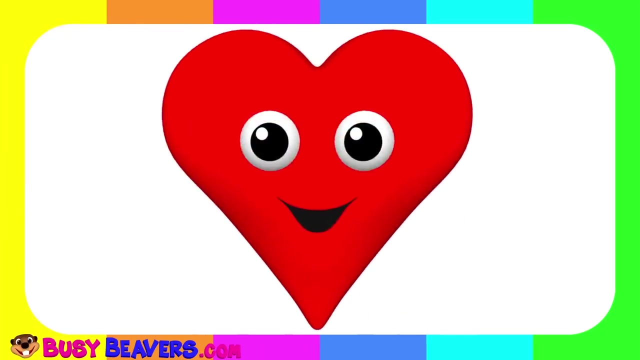 Star Star. Let's try it even quieter. Circle, Circle, Circle Square Square Triangle Triangle Rectangle Rectangle. Oval, Oval, Heart, Heart, Diamond, Diamond Square Triangle Triangle Rectangle Rectangle. 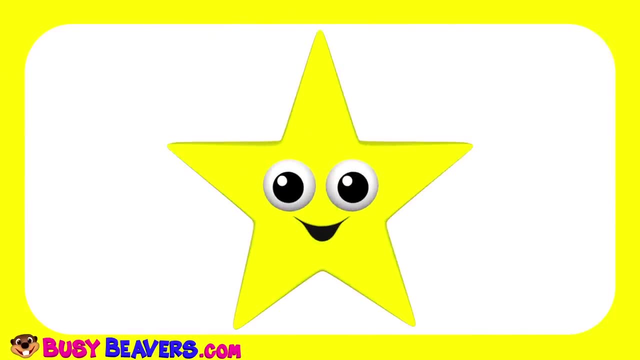 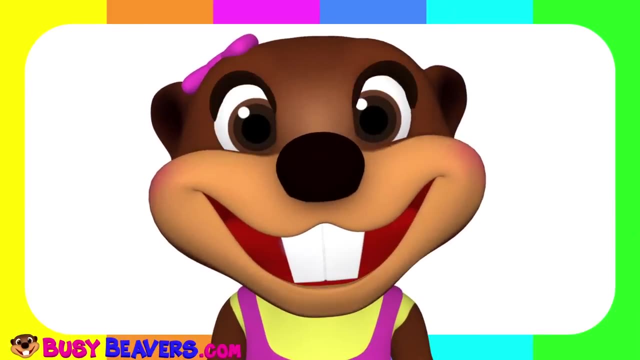 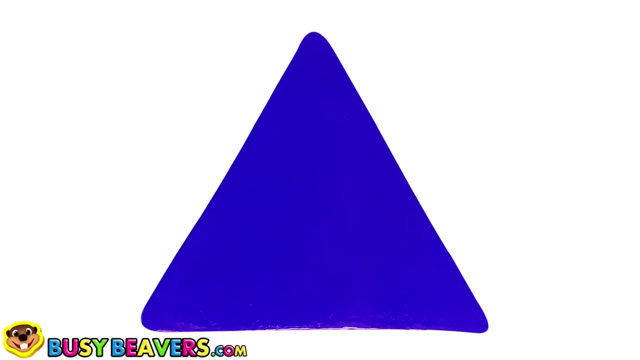 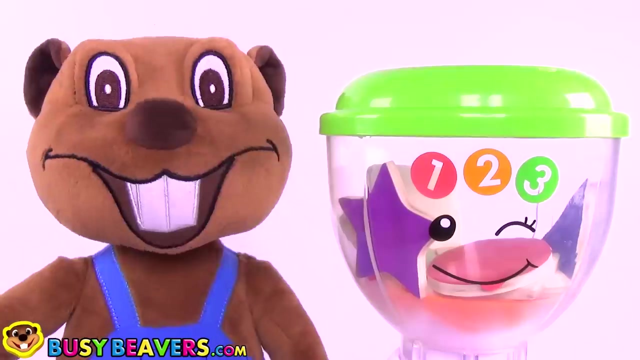 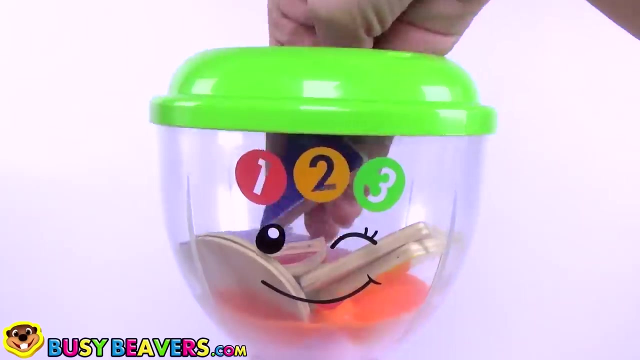 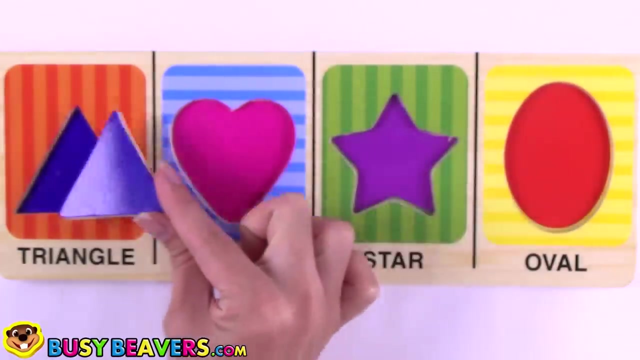 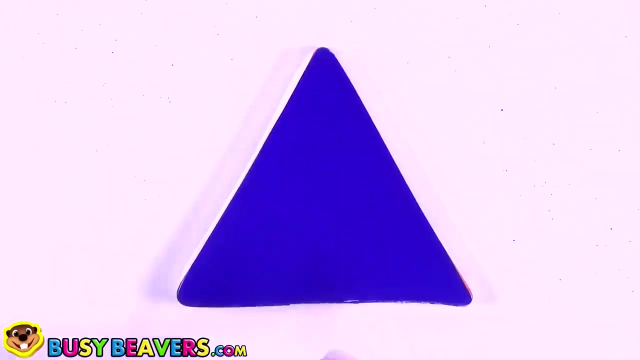 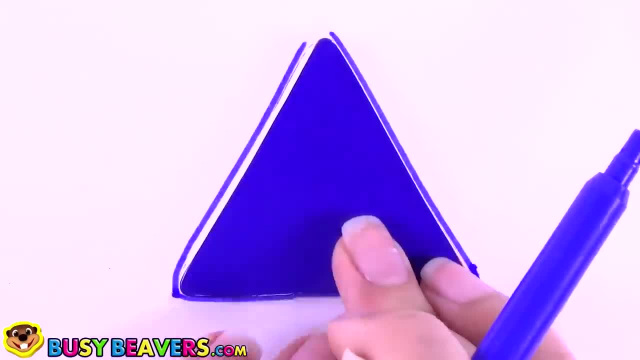 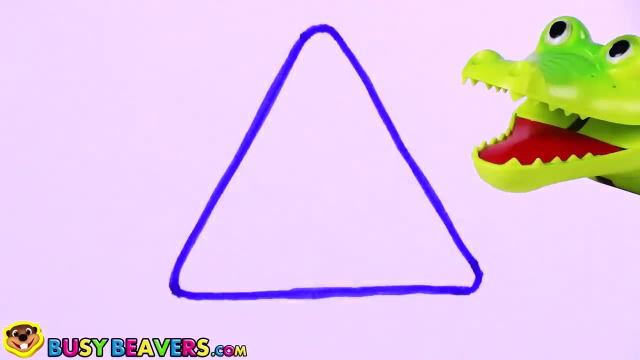 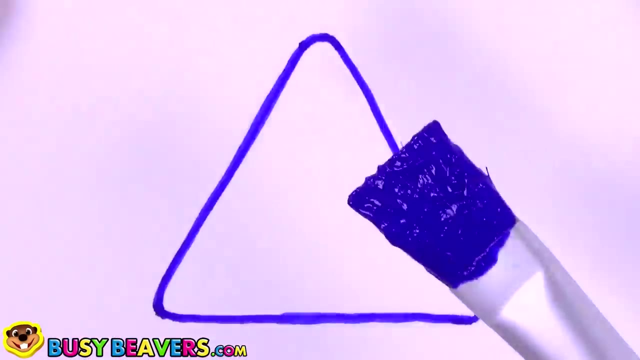 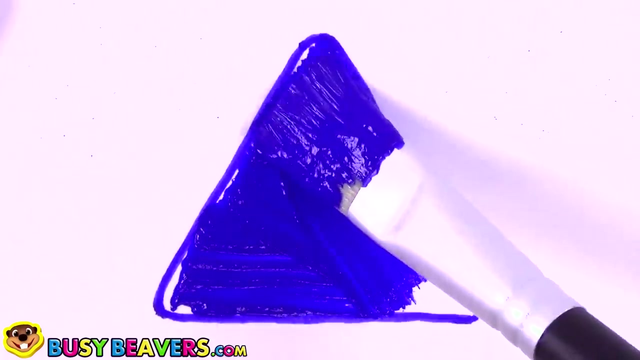 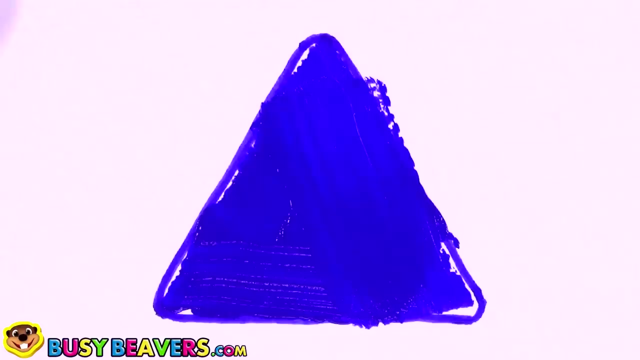 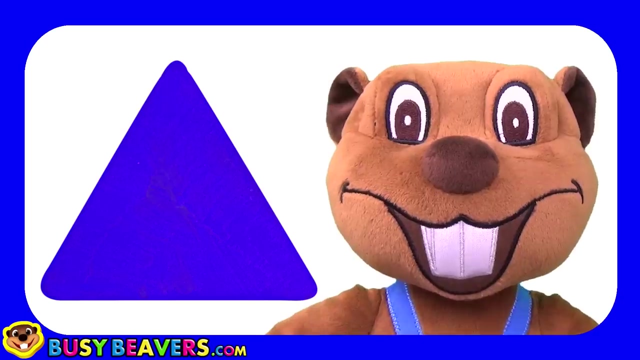 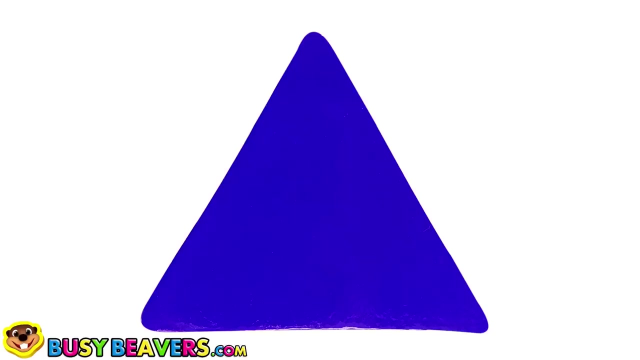 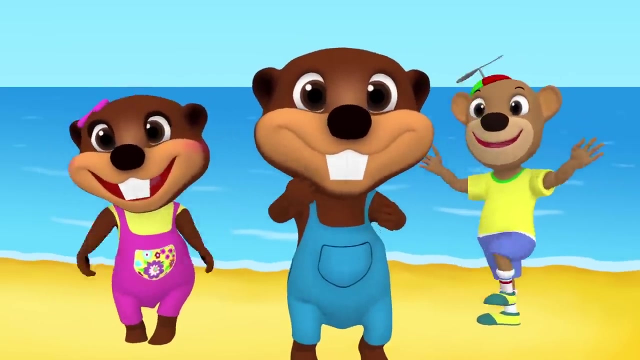 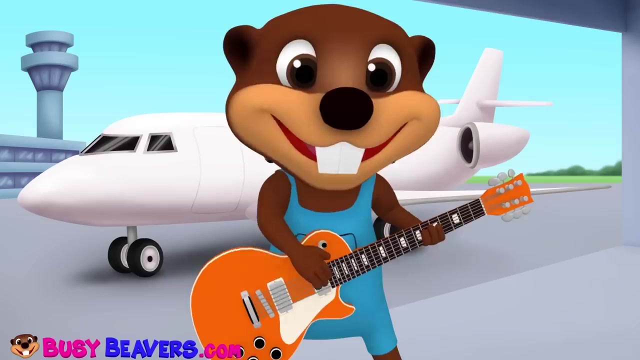 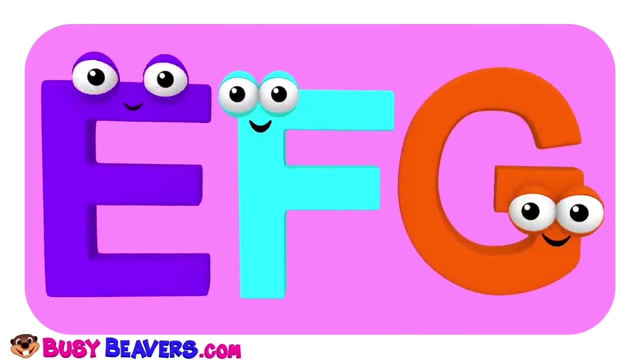 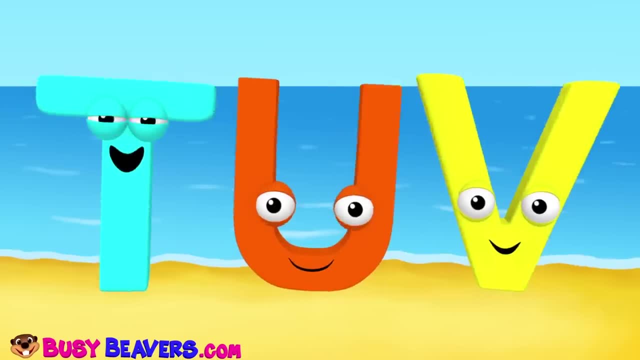 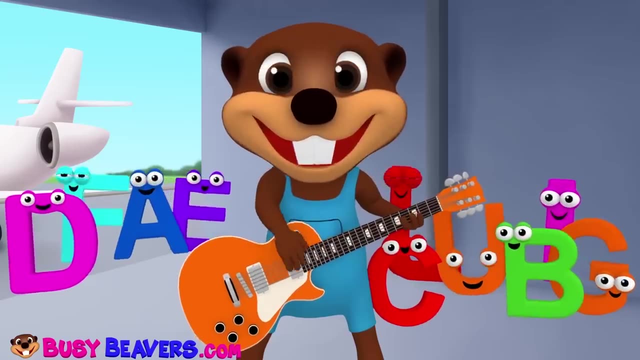 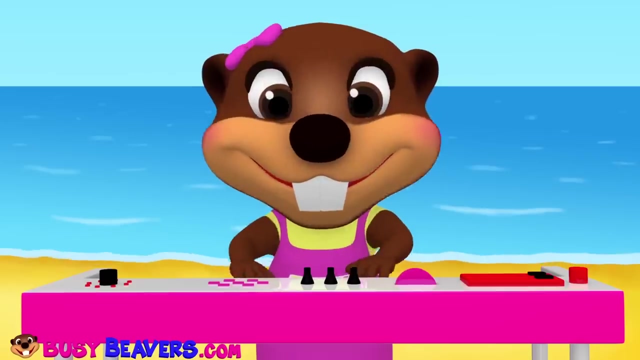 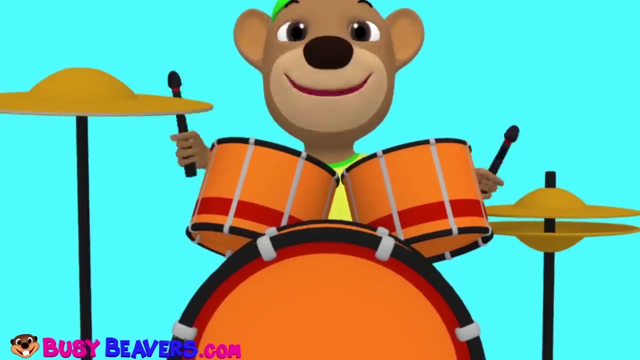 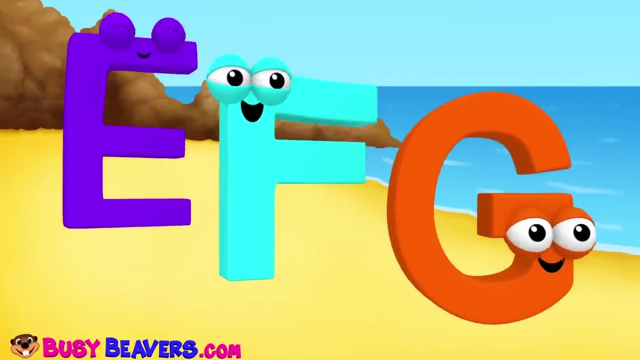 Q R S T U V W X Y Z, W X Y Z One more time. A, B, C, D, E, F, G, H, I, J, K, L, M, N, O P. 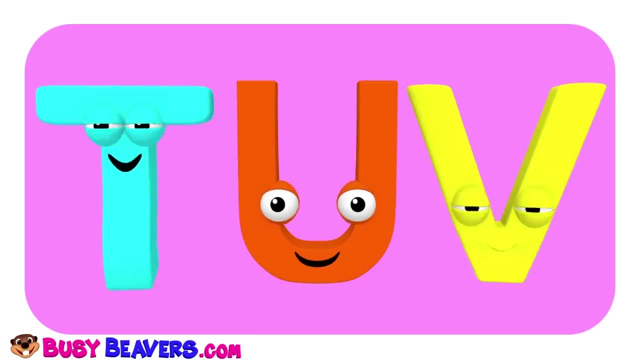 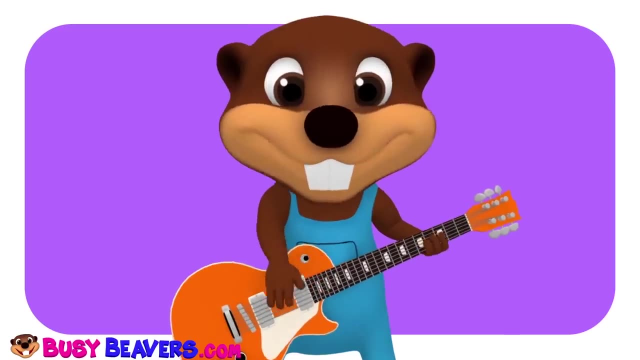 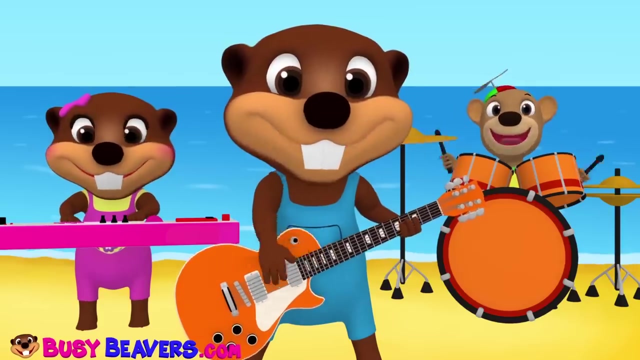 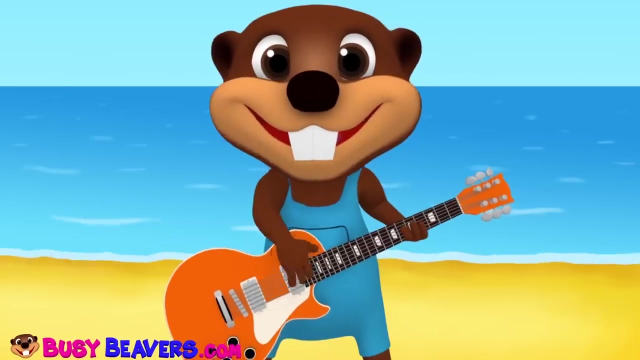 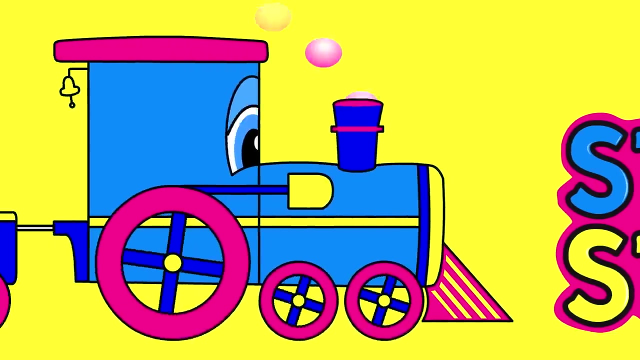 Q R S T U V W X Y Z, W X Y Z A, B, C D N O P Q R S T U V H, I, J, X Y Z. 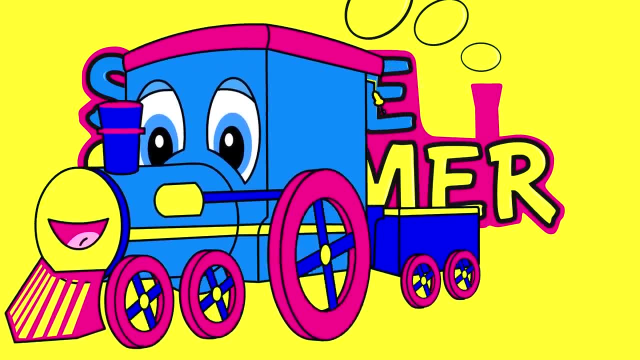 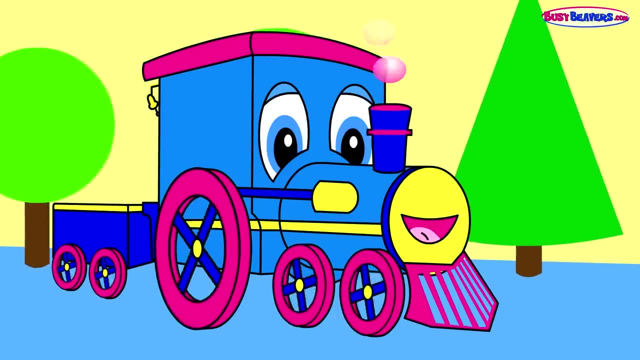 Q, R, S, T, U, V, H, I, J, X, Y Z. Another one. Hello, I'm Stevie Steamer. I'm a train Today. I'm pulling some shapes. Let's go say hi to the shapes and count them. 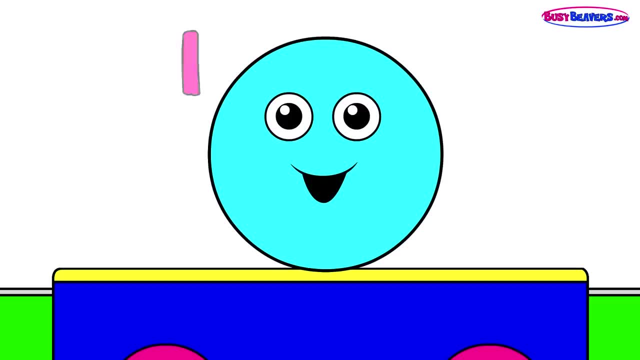 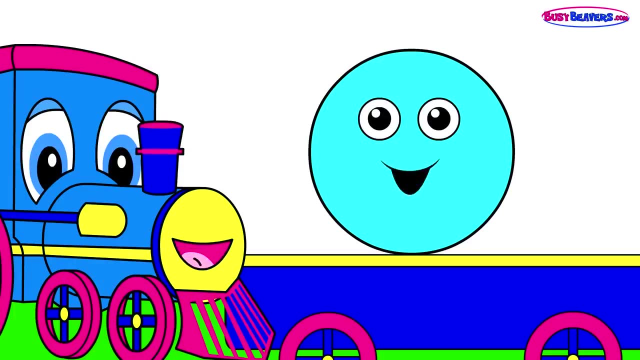 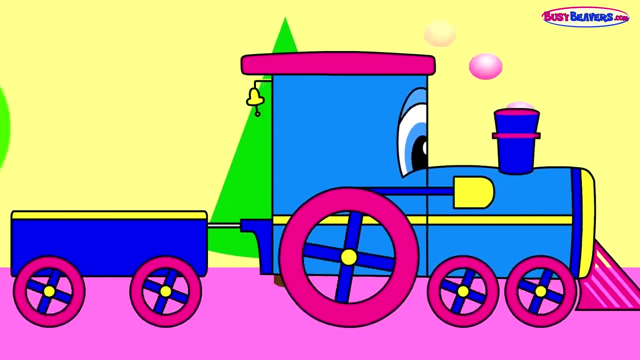 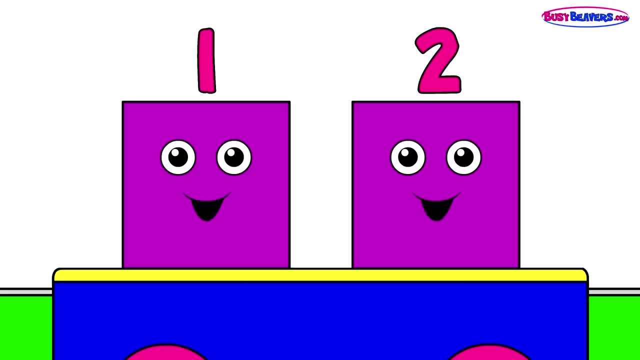 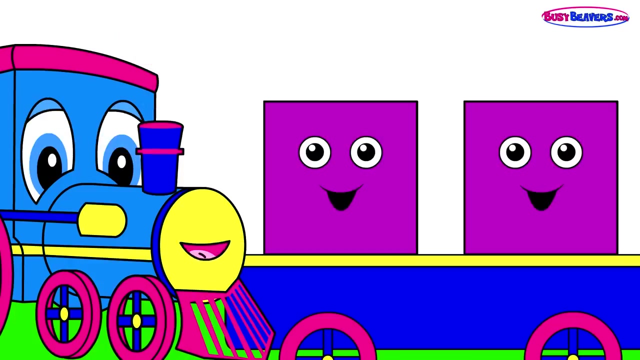 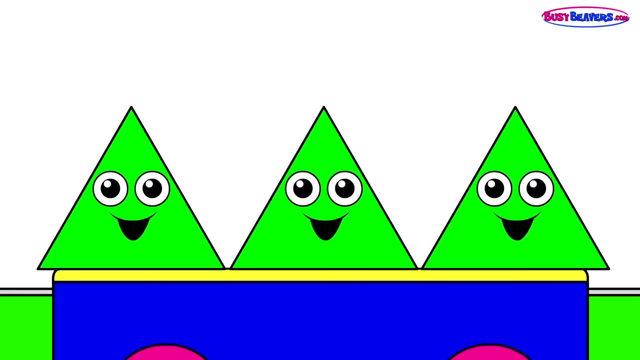 Circle One, One circle, Hello Circle, Oh, Stevie, Cool circle. Squares One, Two, Two squares, Hi. Squares, Hi, Stevie Steamer Squares. Triangles One, Two, Three, Three triangles, Hello, Triangles, Hello. 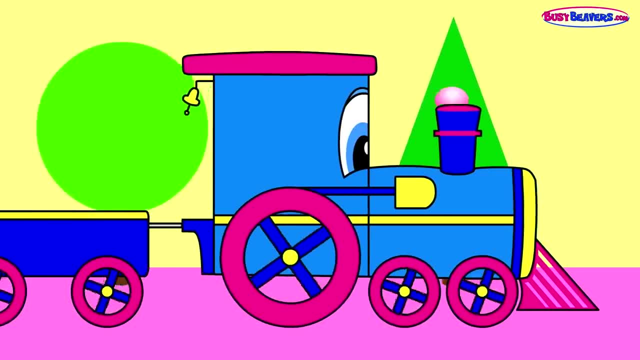 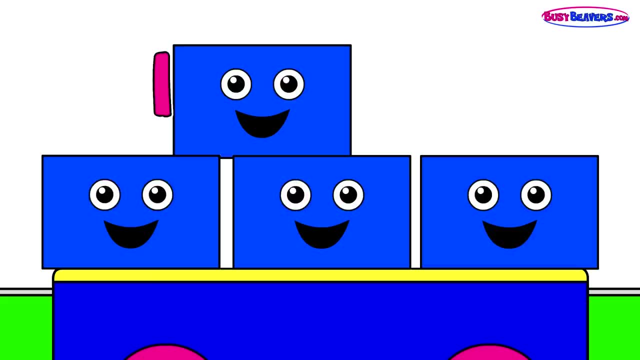 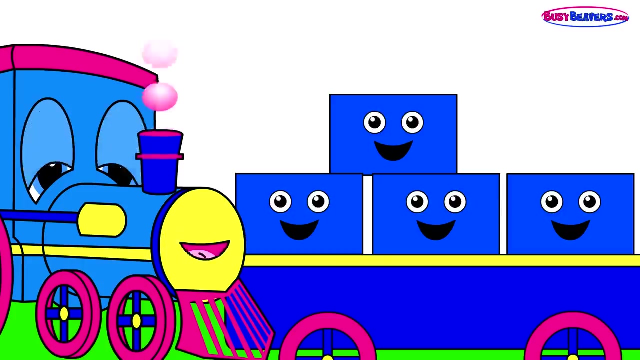 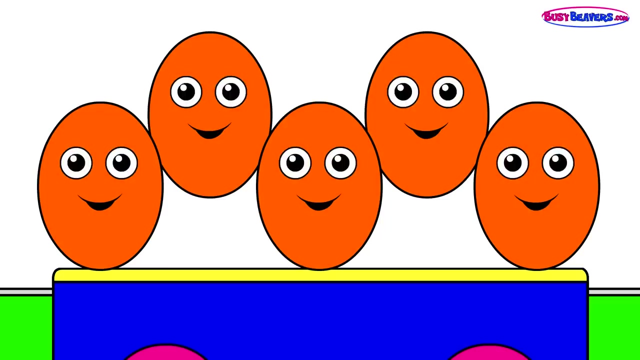 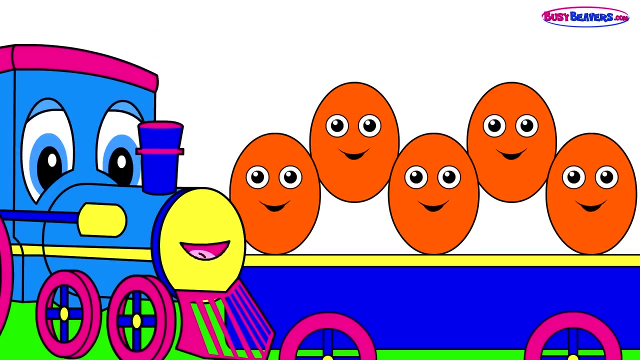 Nice shapes: Rectangles: One, Two, Three, Four, Four. rectangles, Hi, Rectangles, Hi. Stevie Steamer Love the rectangles. Ovals: One, Two, Three, Four, Five, Five ovals, Hey, Ovals, Hi, How you doing Well. that's all the shapes for today. 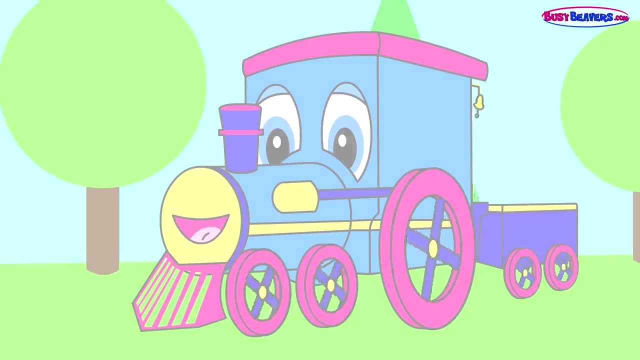 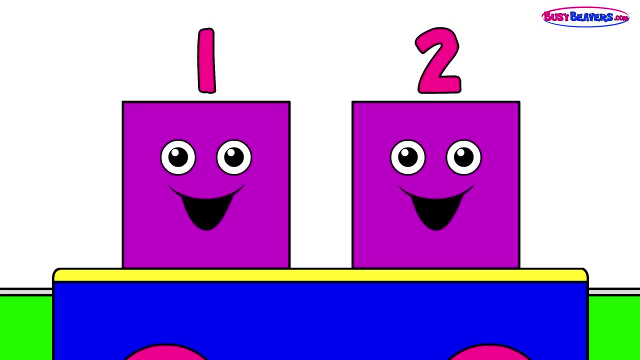 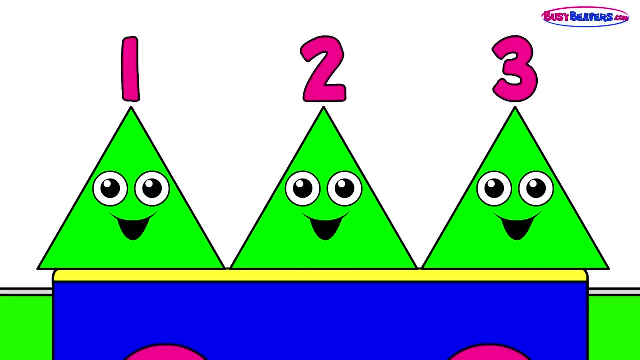 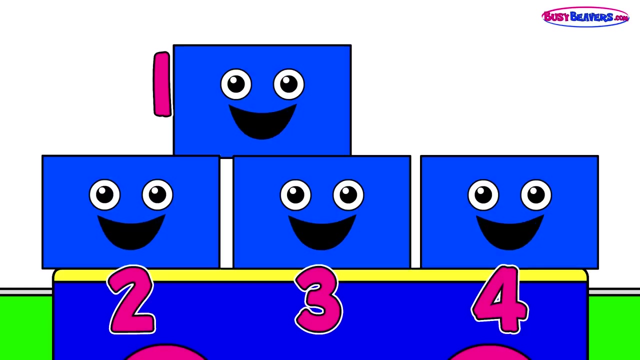 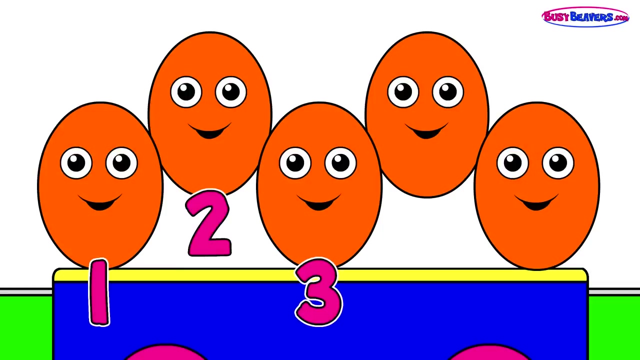 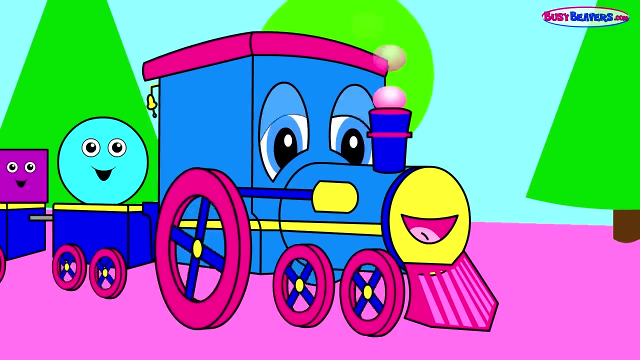 Let's count them one more time: One circle: One. Two squares. One, Two, Three triangles. One, Two, Three, Four rectangles Down hearts: One, Two, Three, Three, Four, Five Ovals, Yip-yip-yip, All aboard. Hehe, here we go. 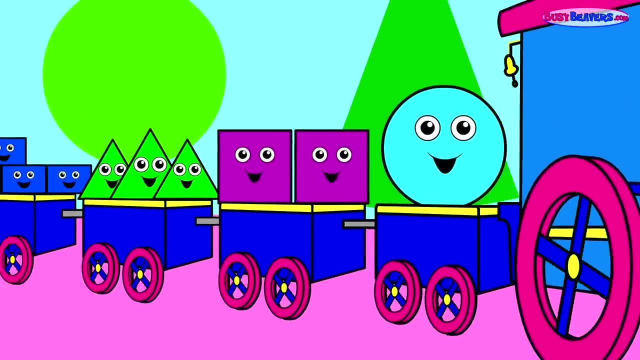 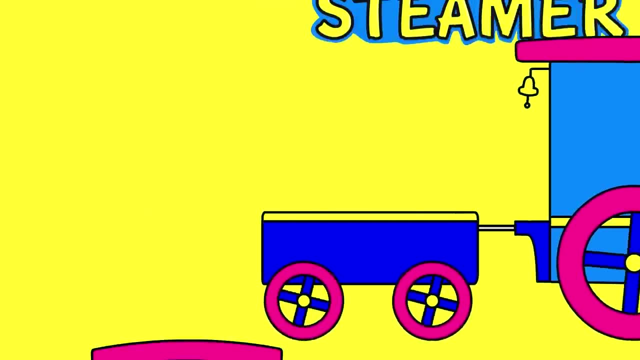 By-yip-yip-yip-yip-yip-yip-yip-yip-yip-yip-yip-yip-yip, Whip-whip. Stevie Steamer. That's my name, Stevie Steiner. I'm a train. 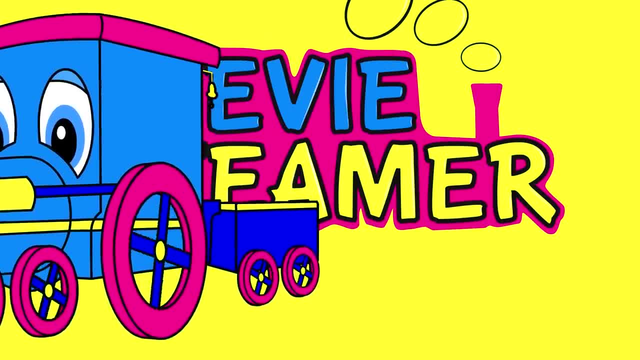 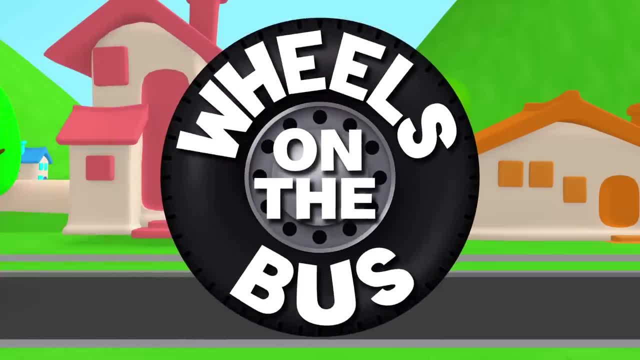 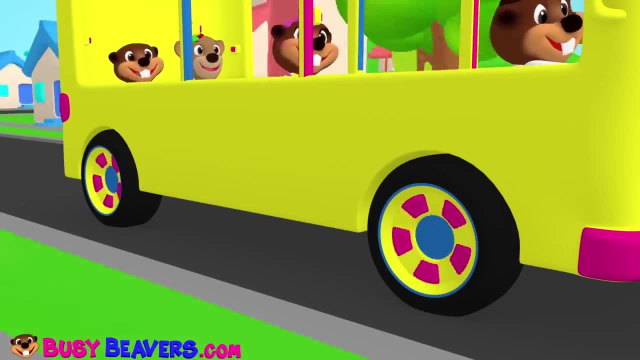 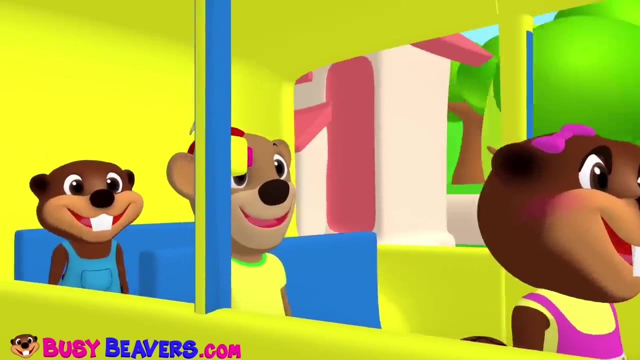 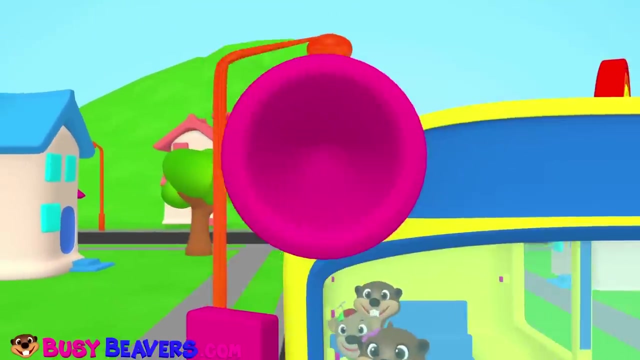 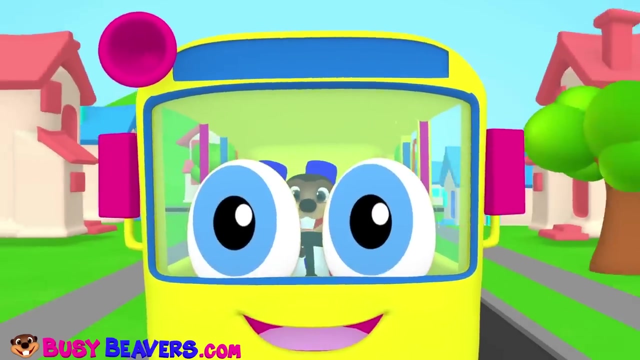 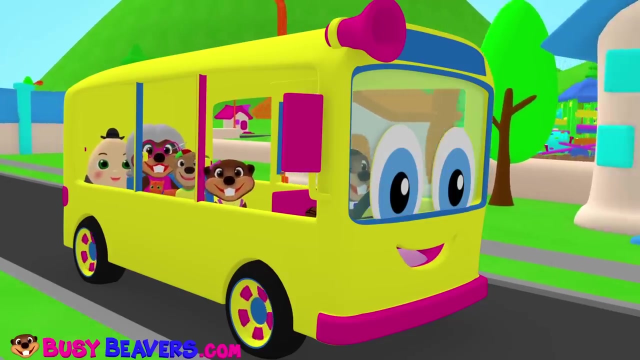 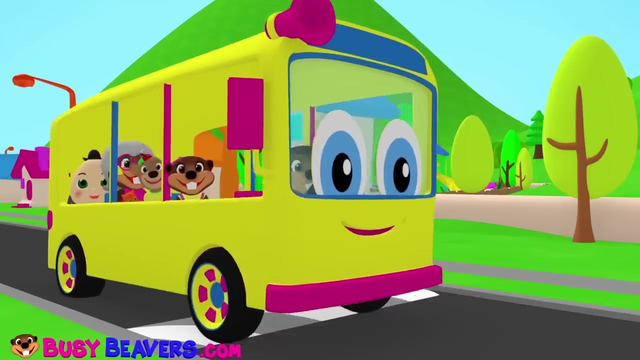 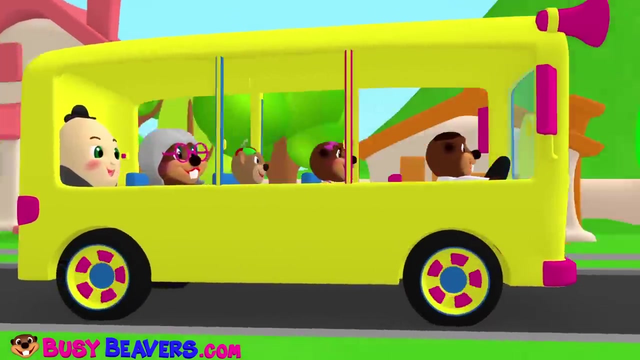 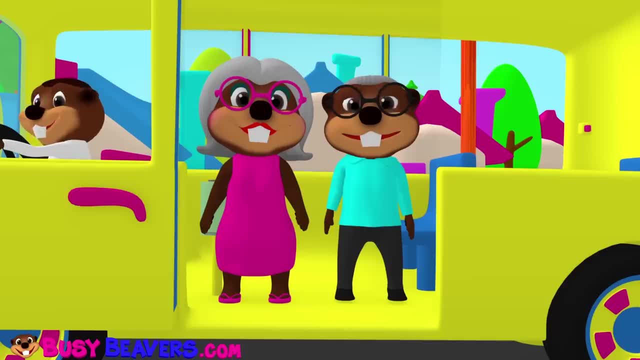 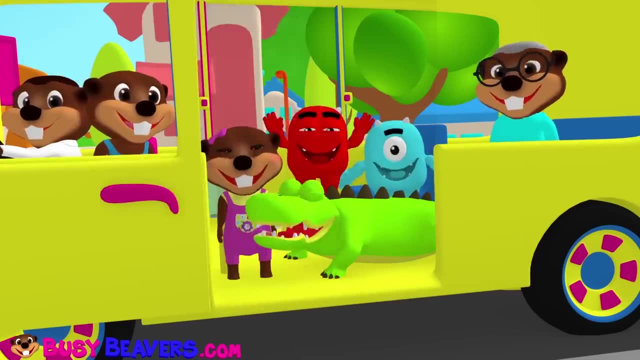 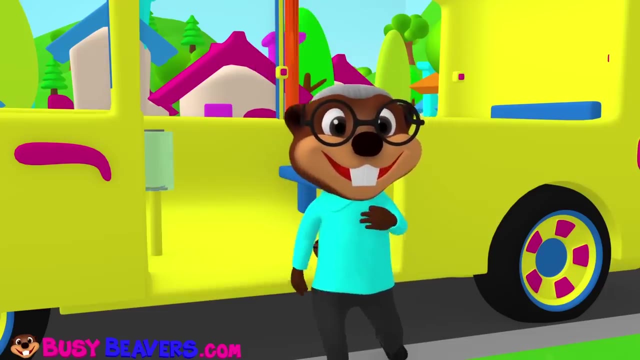 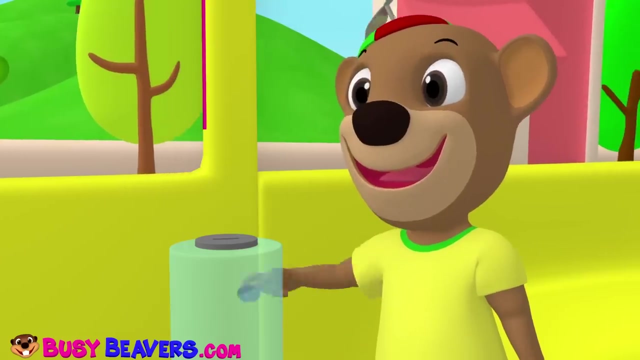 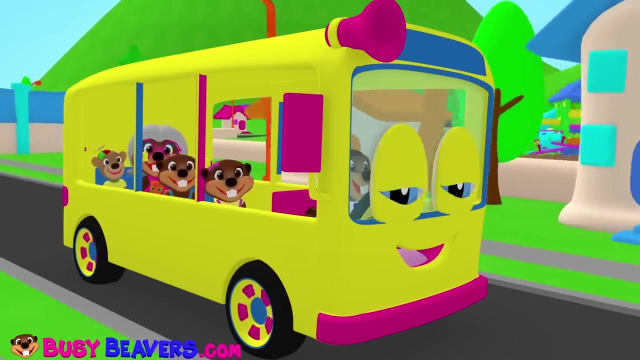 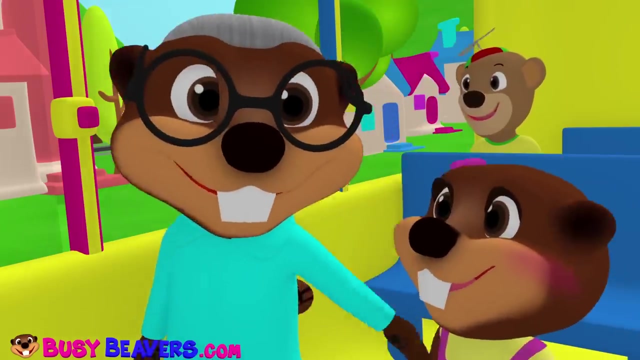 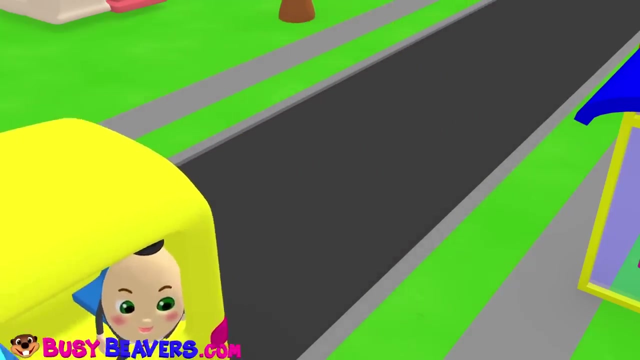 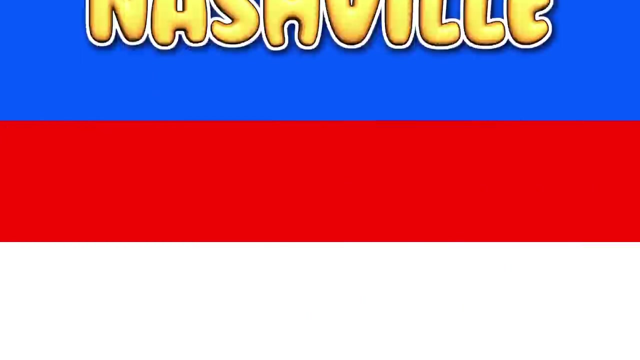 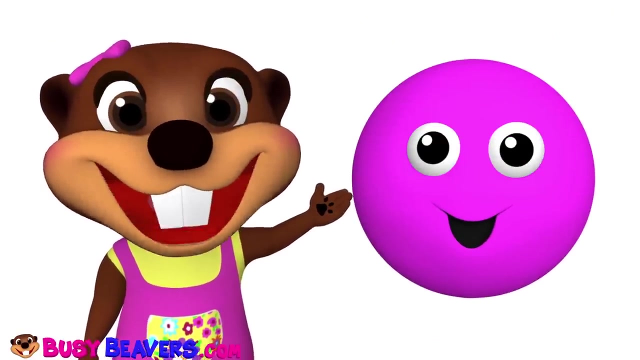 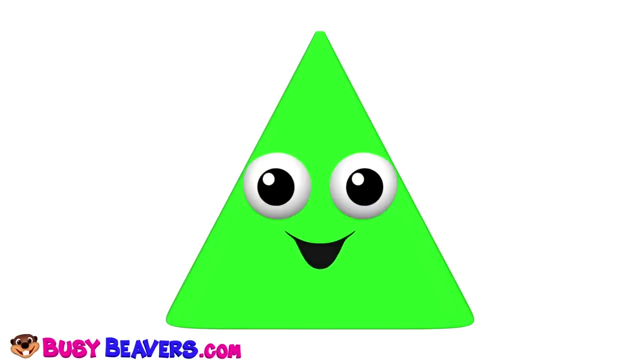 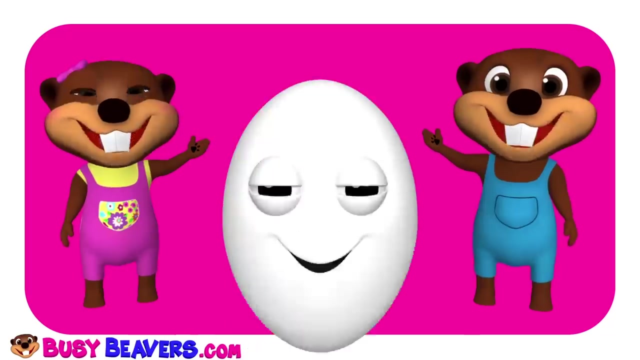 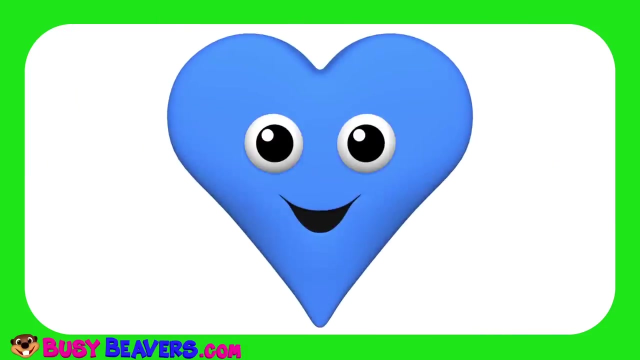 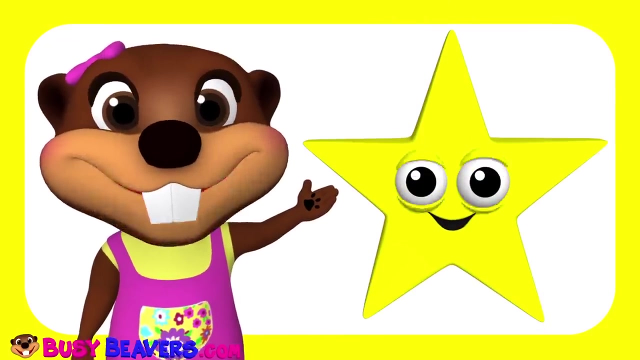 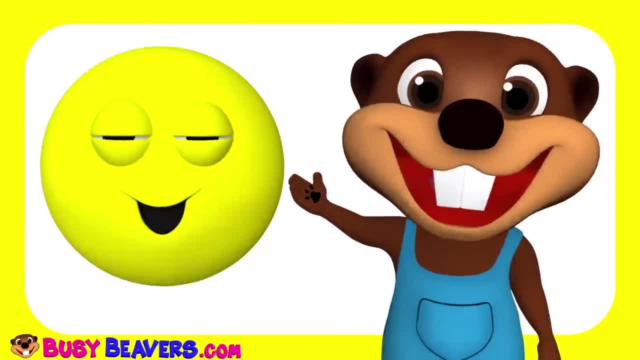 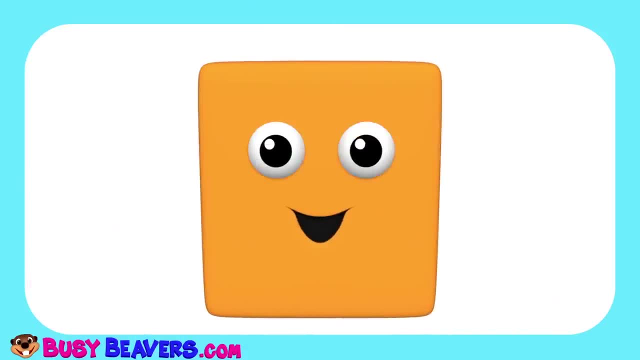 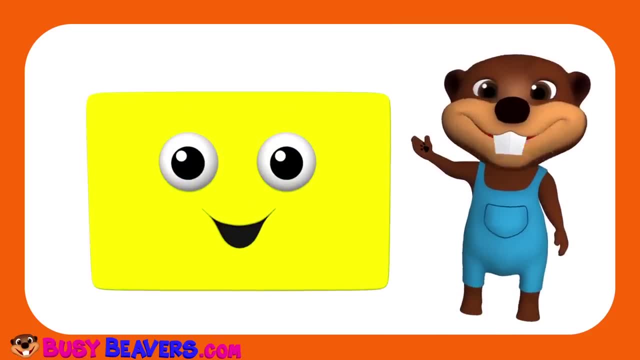 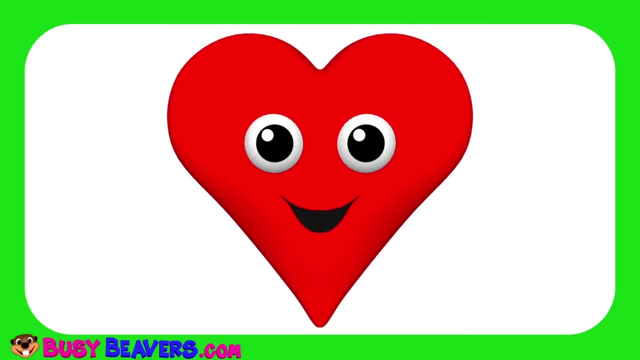 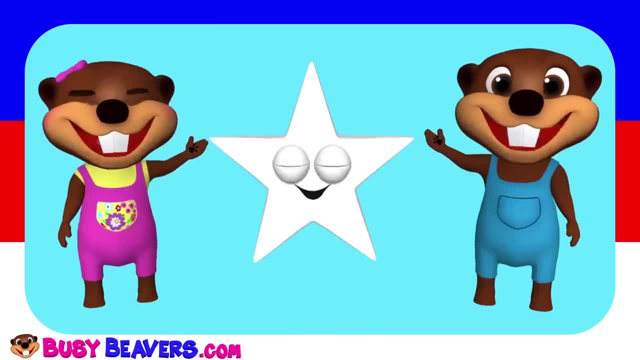 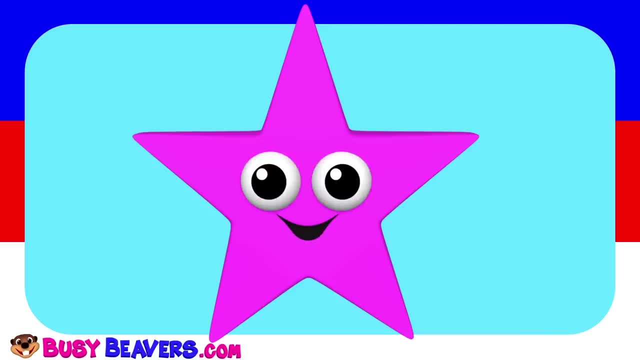 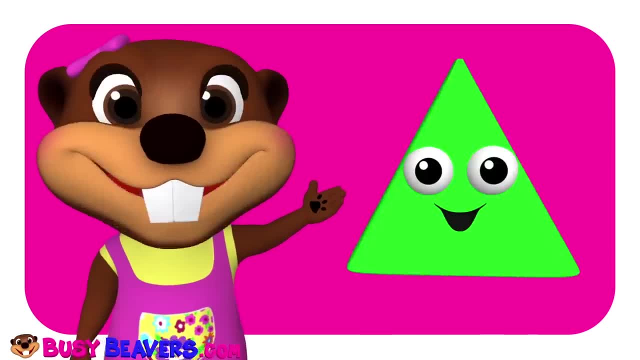 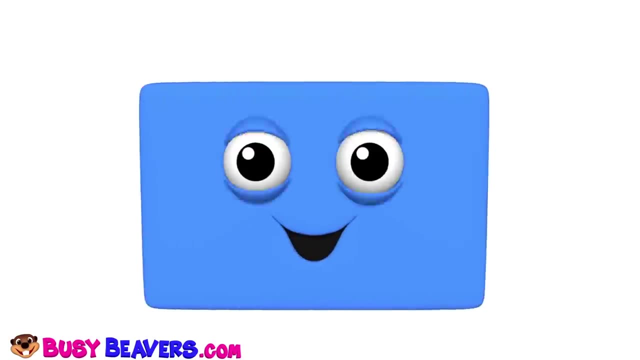 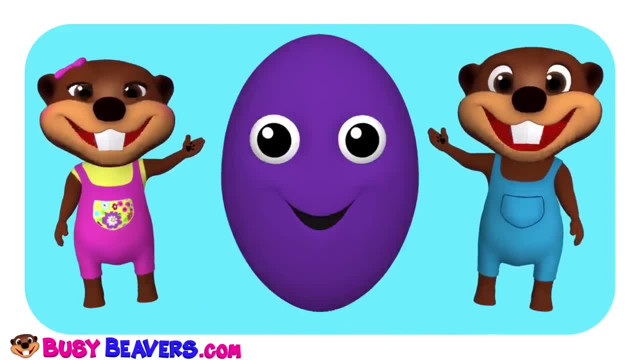 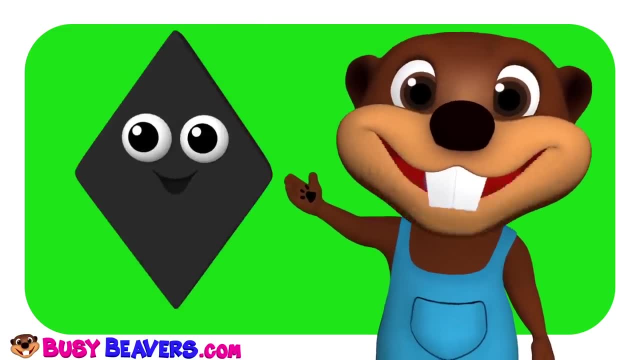 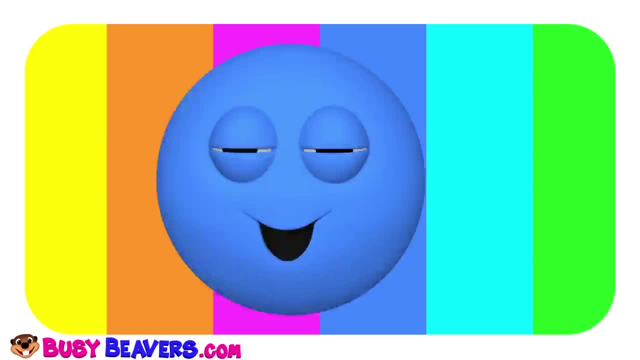 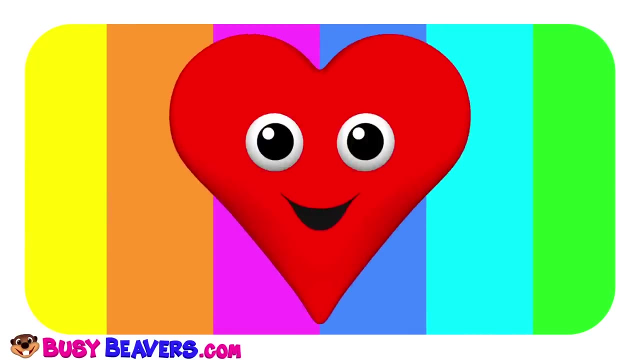 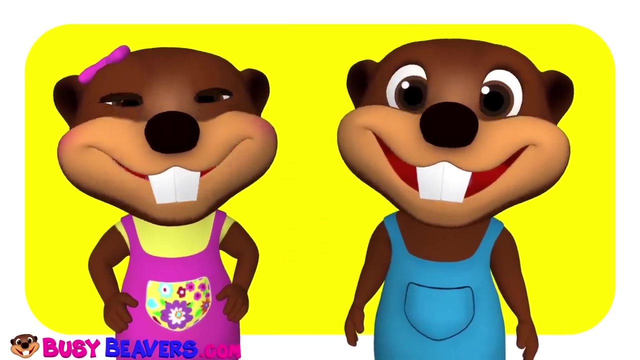 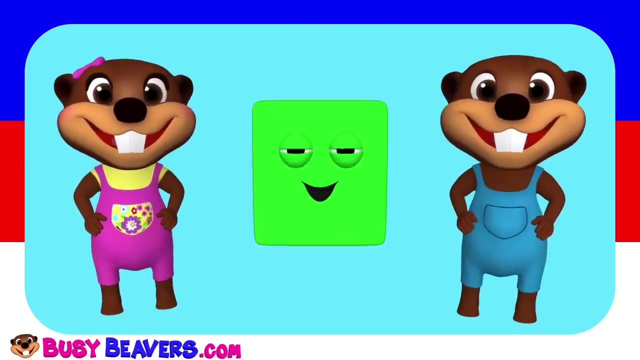 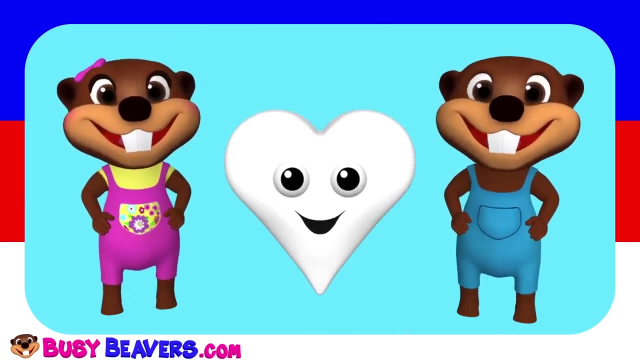 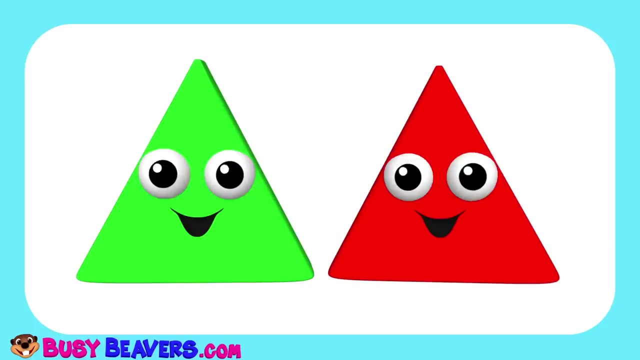 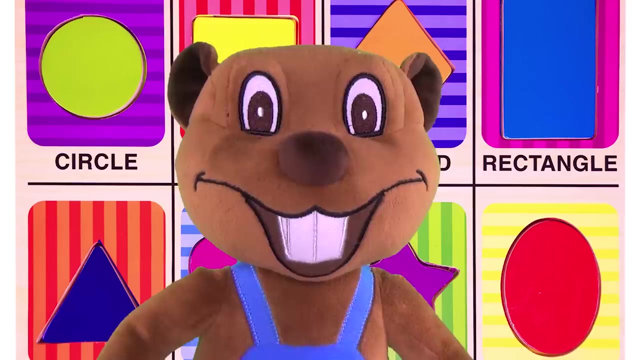 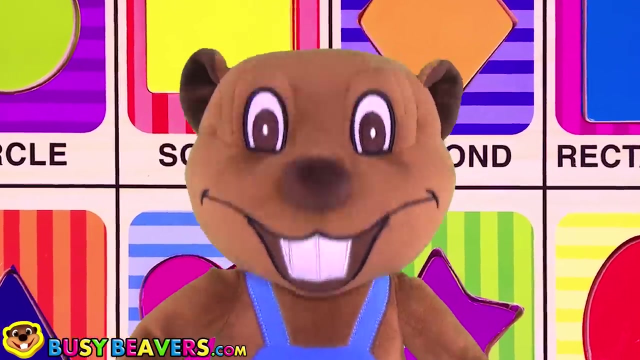 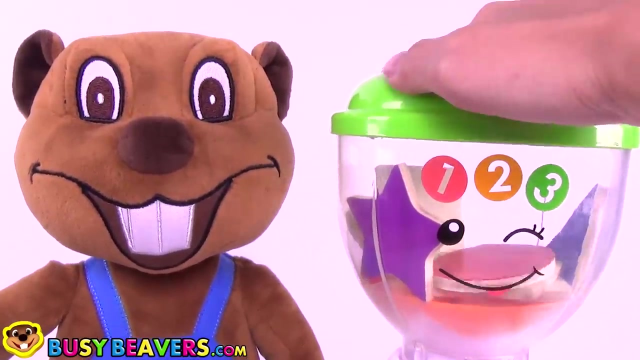 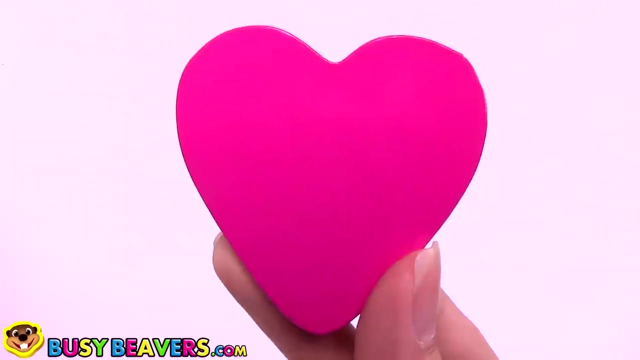 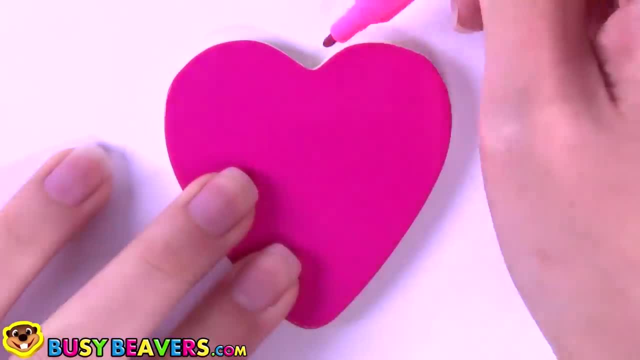 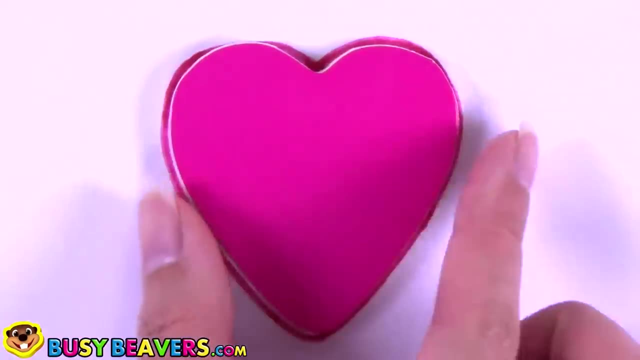 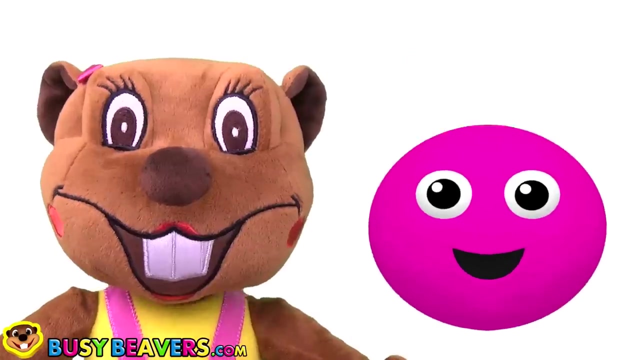 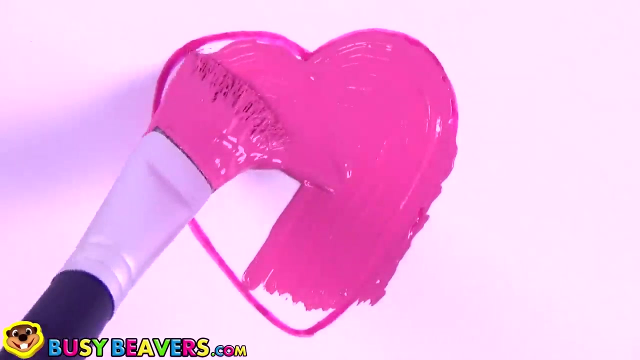 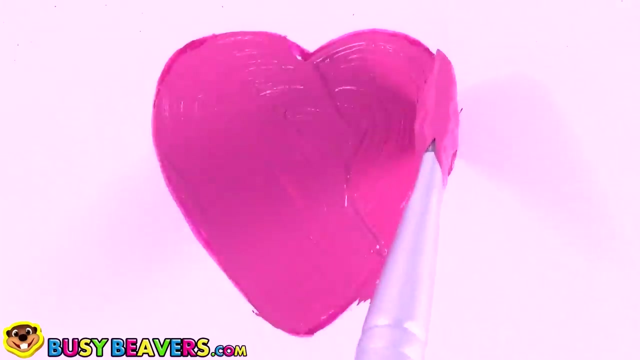 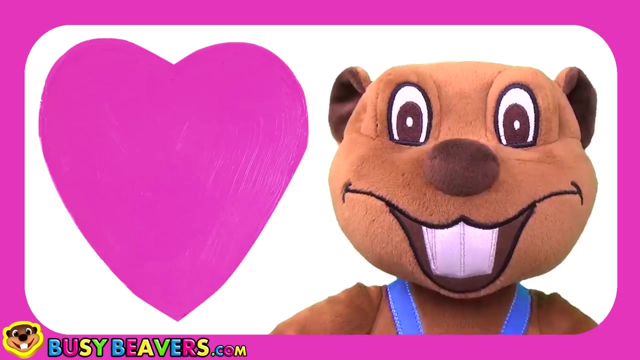 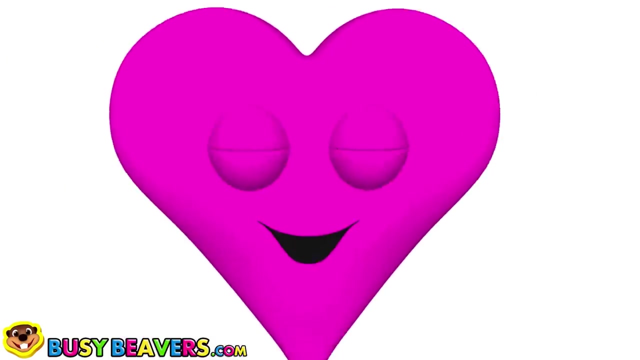 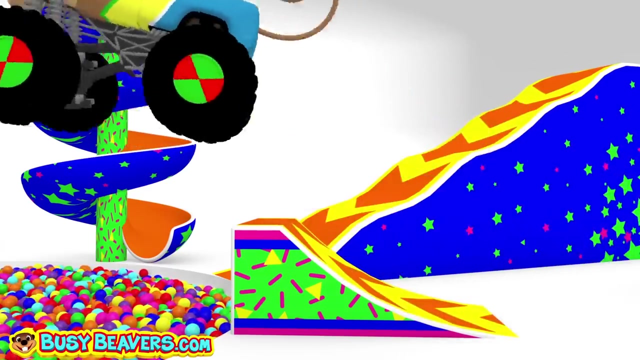 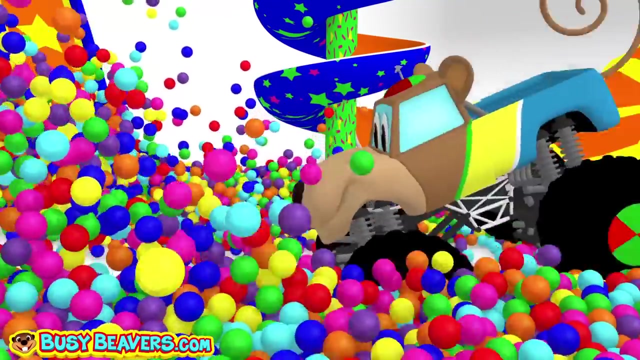 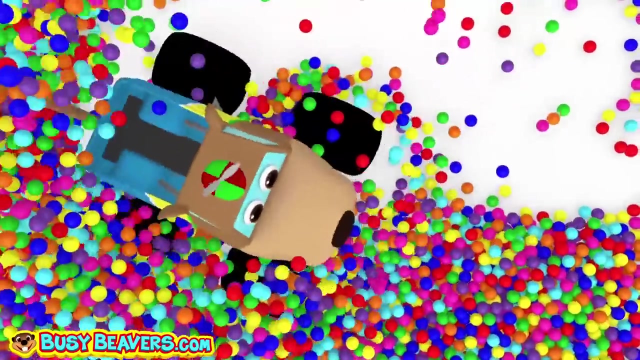 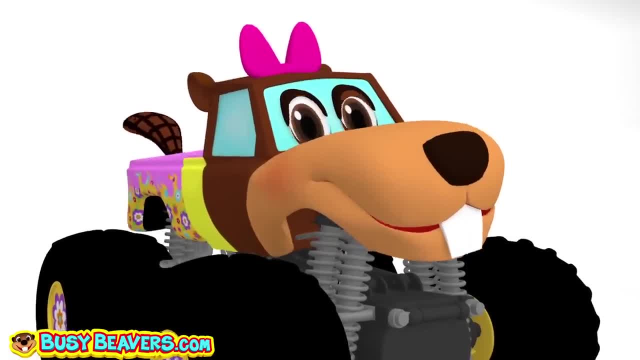 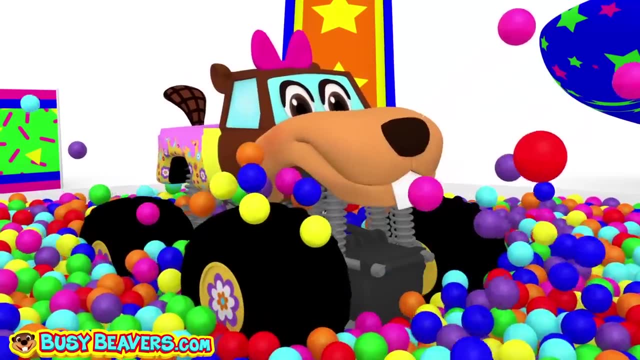 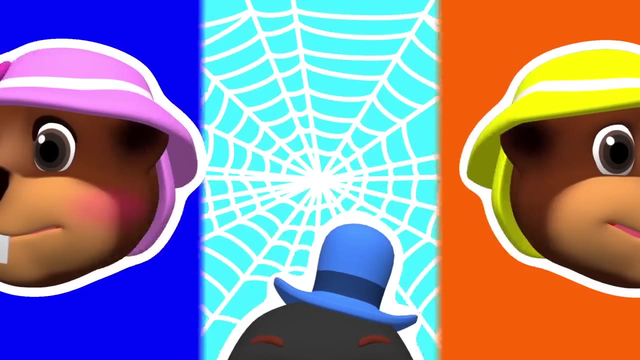 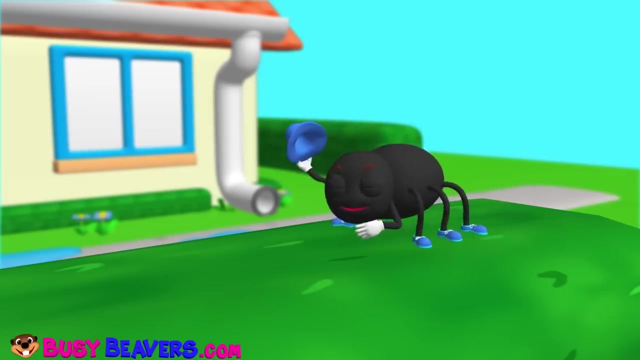 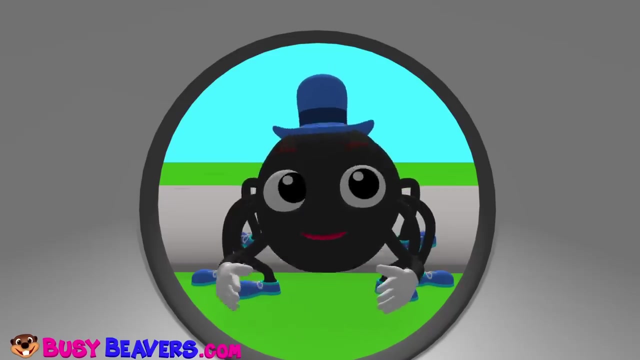 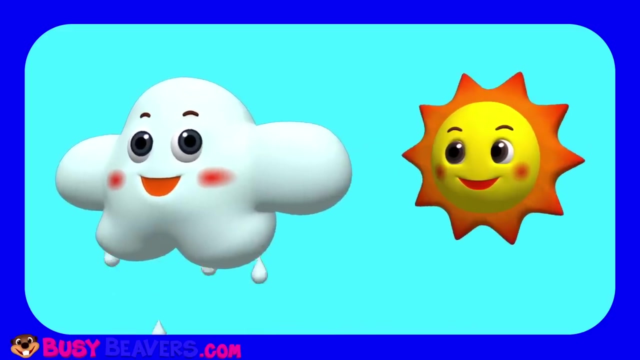 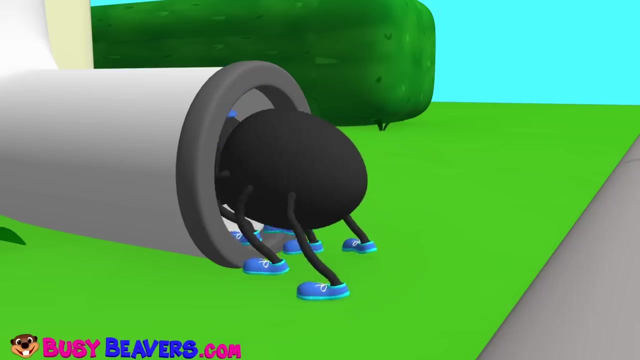 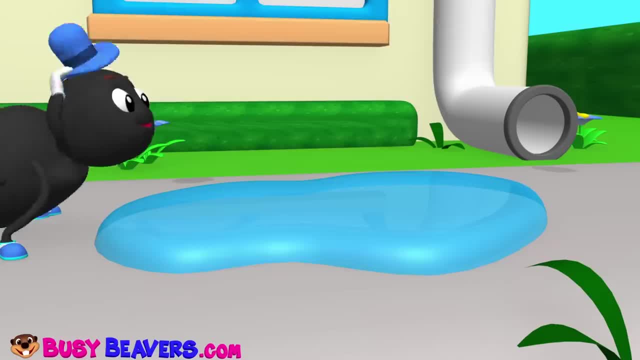 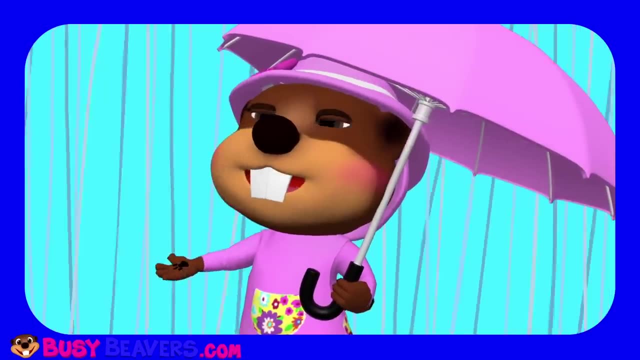 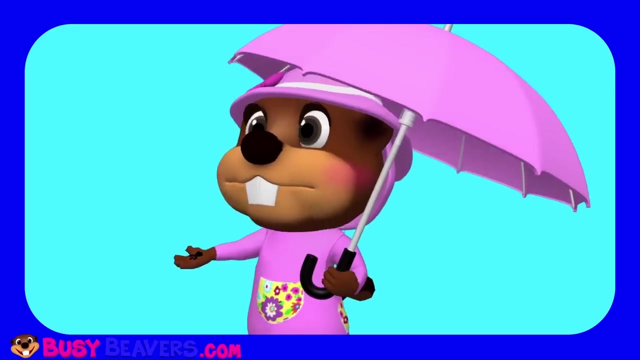 The Incy Wincy Spider went up the water spout. Down came the rain and washed the spider out. Out came the sun and dried up all the rain. That's good. The Incy Wincy Spider went up the water spout. The Incy Wincy Spider went up the water spout again. 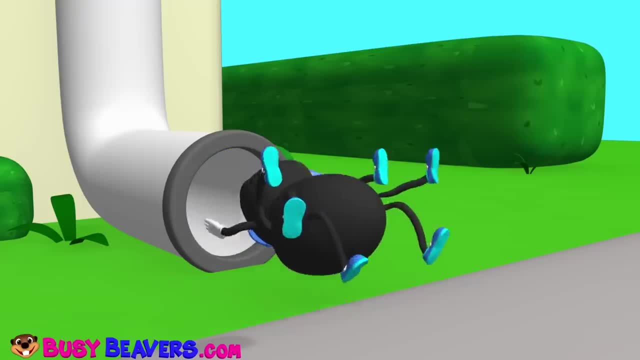 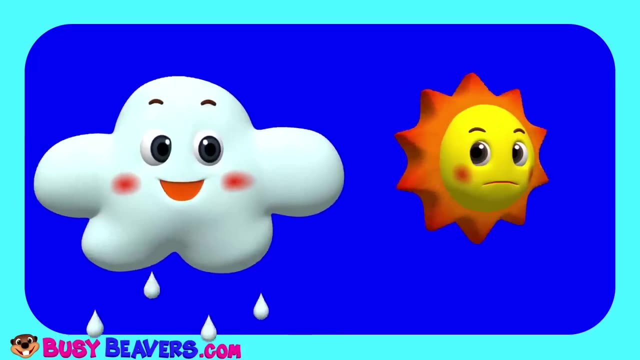 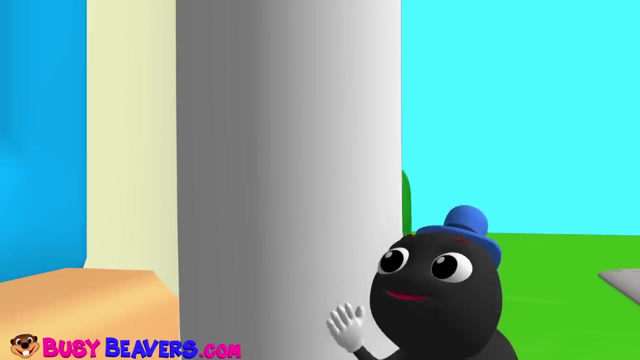 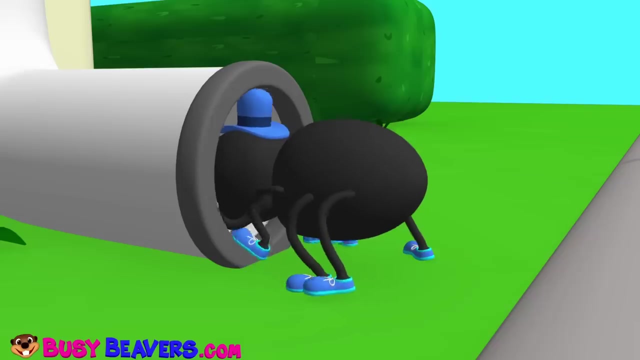 The Incy Wincy Spider went up the water spout, Down came the rain and washed the spider out. Out came the sun and dried up all the rain. That's good. The Incy Wincy Spider went up the water spout Down came the rain and washed the spider out. 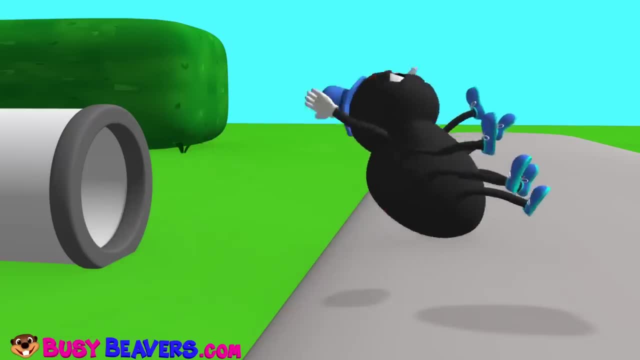 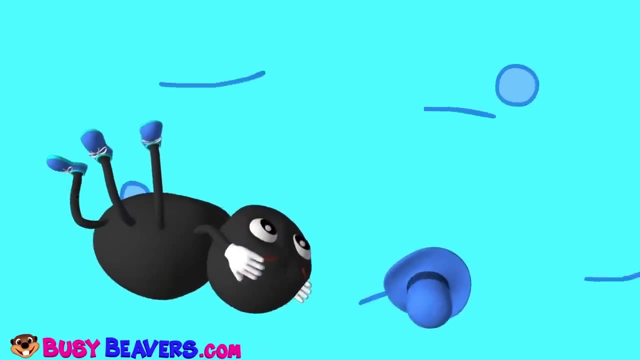 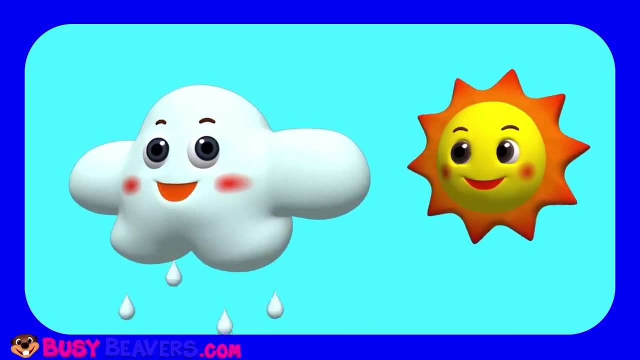 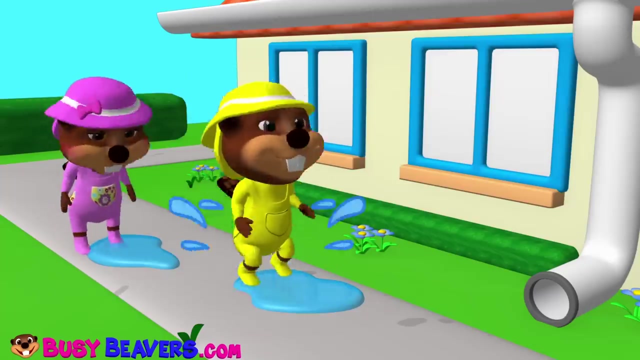 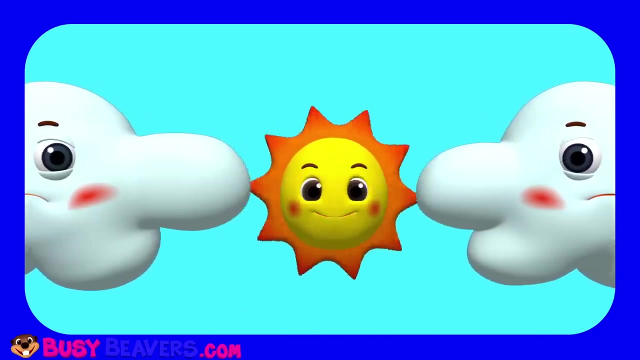 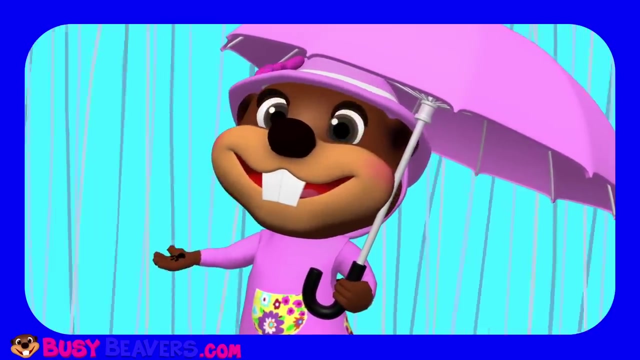 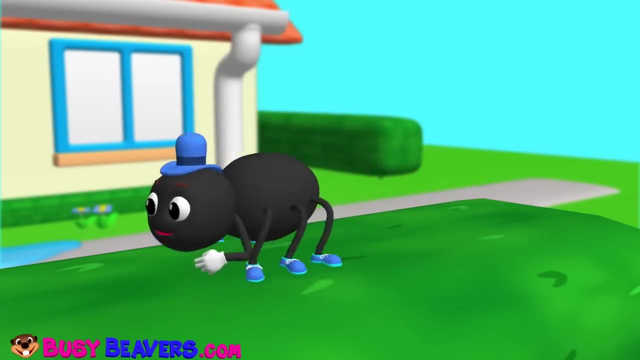 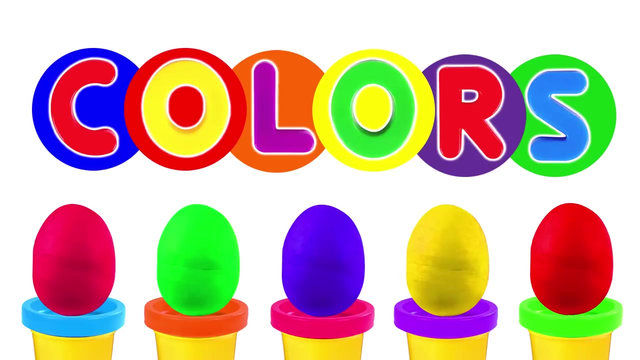 Out came the sun and dried up all the rain. The Incy Wincy Spider went up the water spout. Down came the sun and dried up all the rain. The Incy Wincy Spider went up the water spout again. I really like that. I can't stop smiling now. 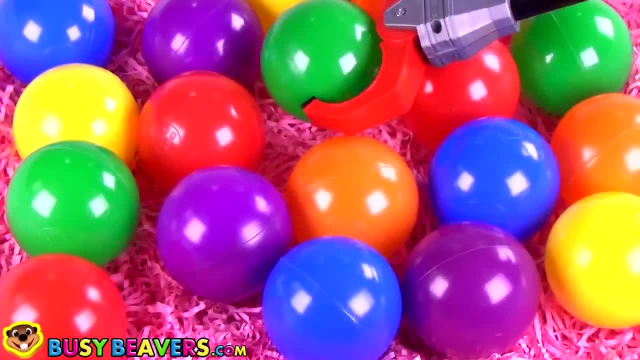 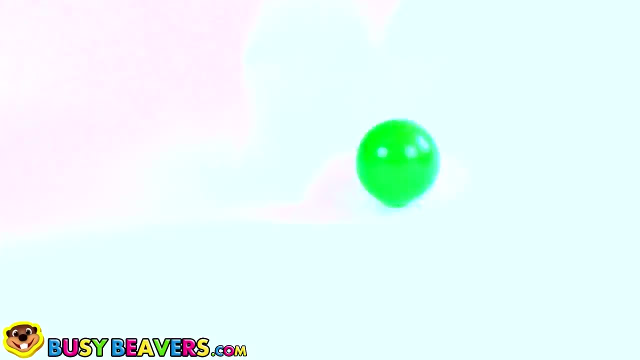 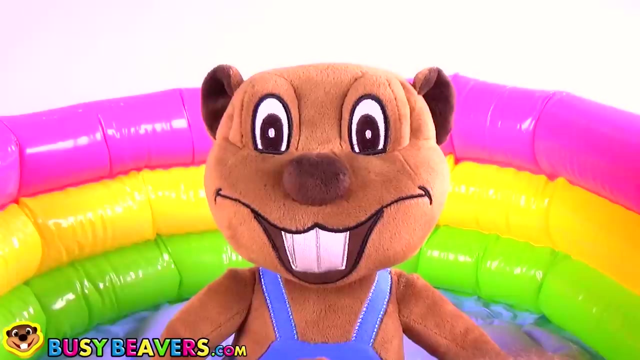 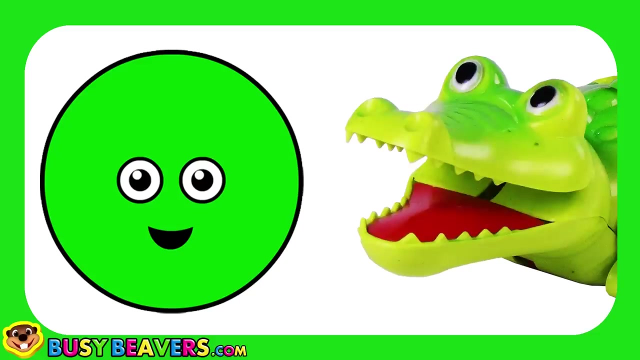 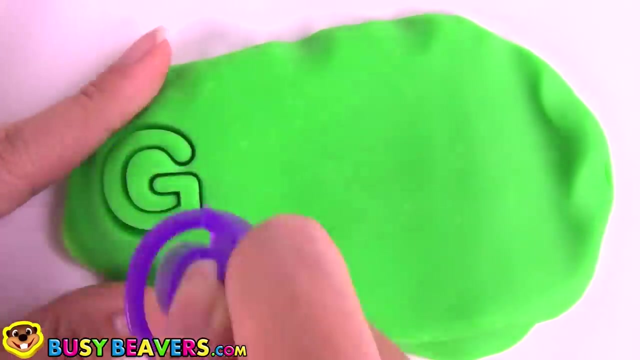 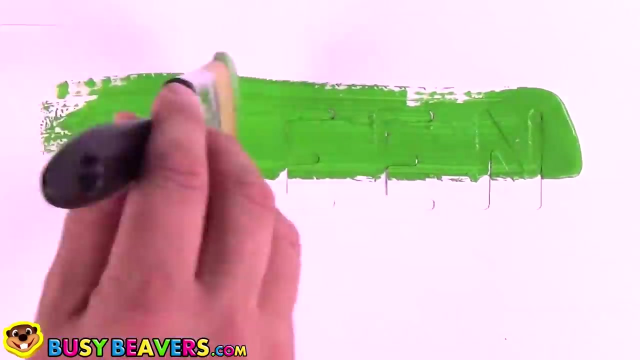 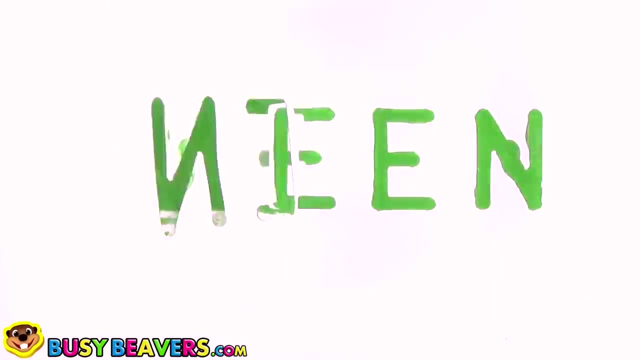 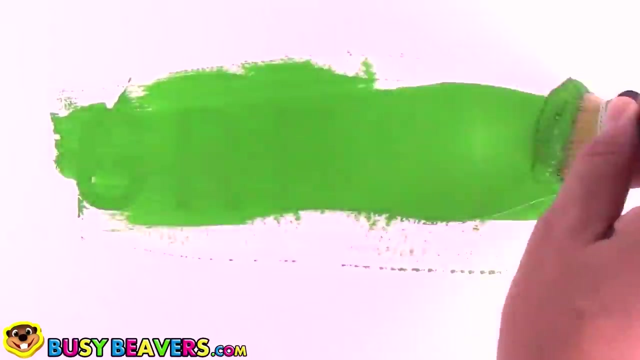 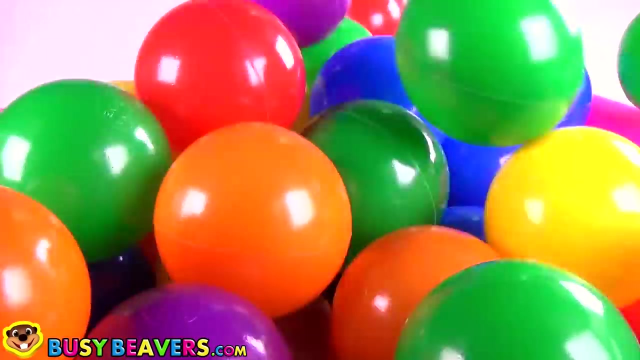 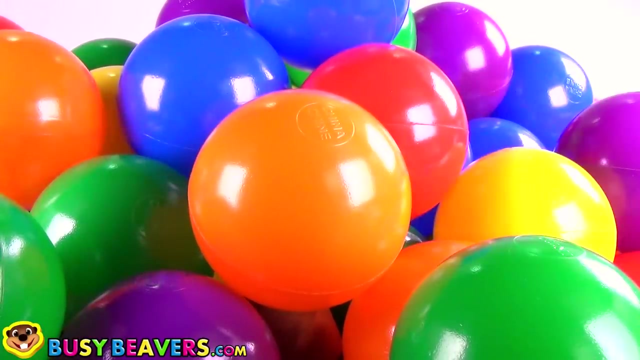 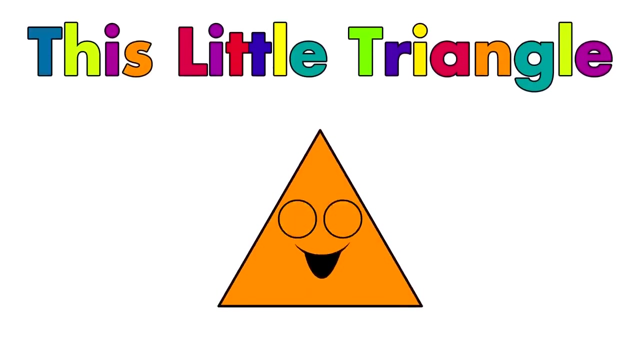 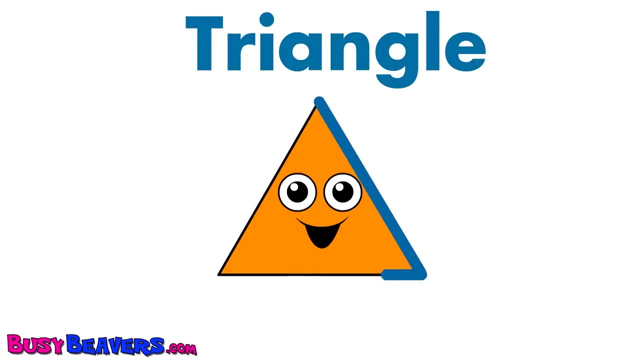 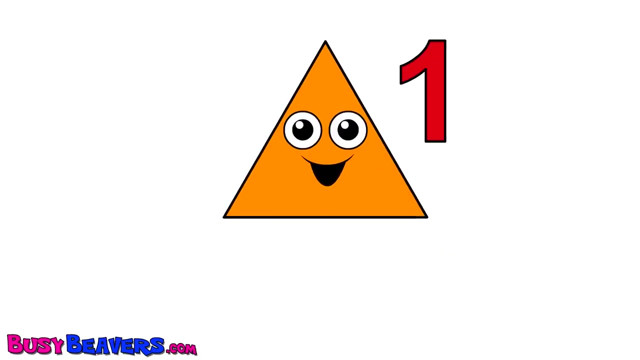 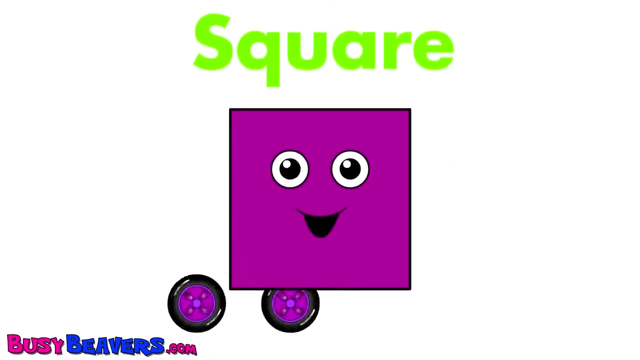 I know, ha, Green, Green, Green, Green, Green, Green Green, Surprise, Surprise. Okay, here we go. This little triangle has three sides. This little triangle has three sides. This little triangle has three sides: One, two, three, he sides. This little square has four sides. 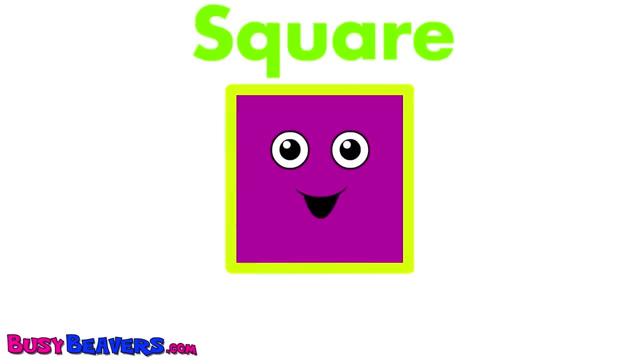 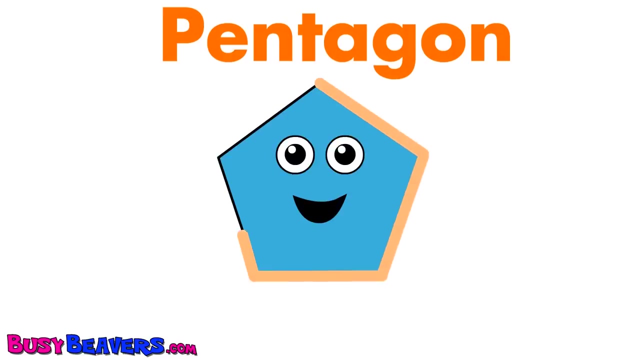 This little square has four sides. This little square has four sides: One, two, three, four sides. This little pentagon has five sides. This little pentagon has five sides. This little pentagon has five sides: One, two, three, four, five. This little hexagon has six sides. 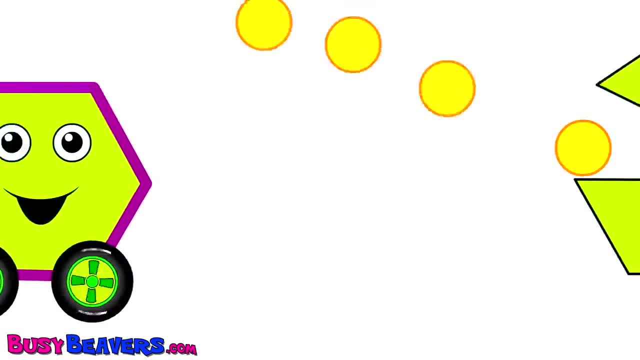 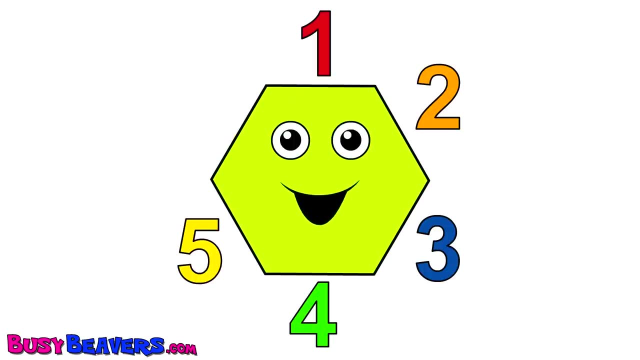 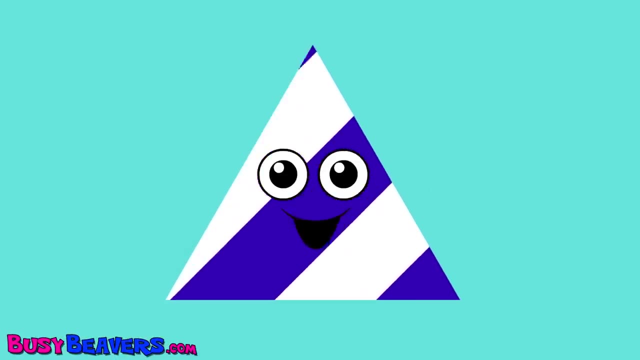 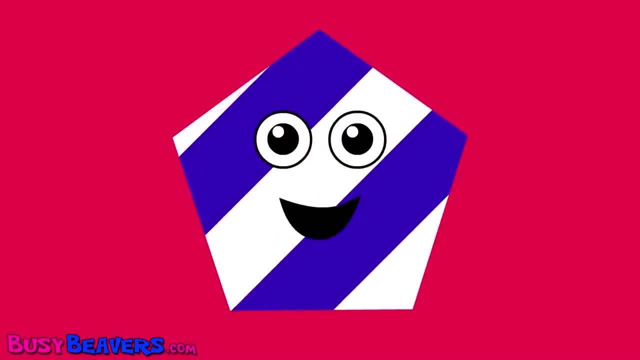 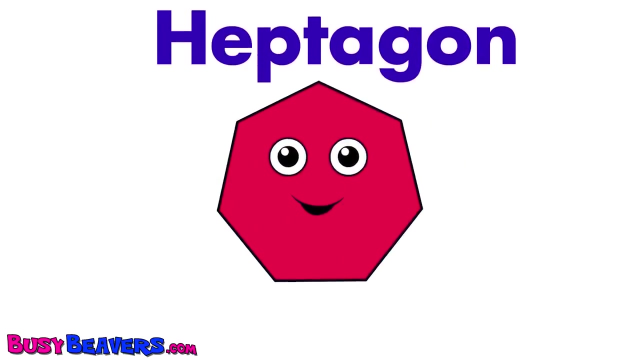 This little hexagon has six sides. This little hexagon has six sides: One, two, three, four, five, six Sounds pretty good. It's fun, Let's play. This little hexagon has seven sides. This little hexagon has seven sides. 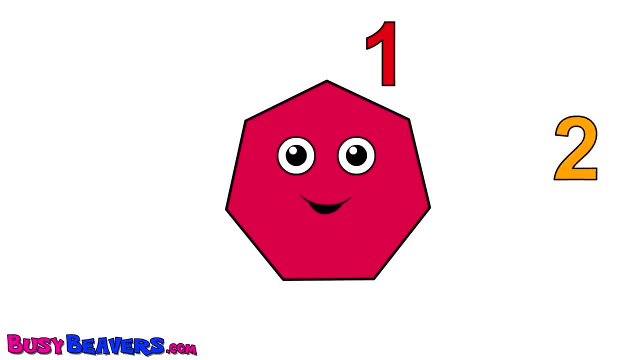 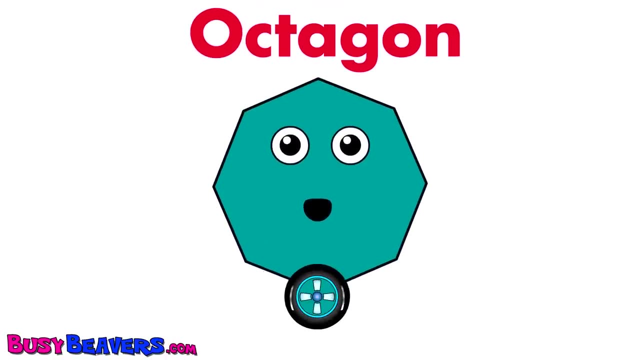 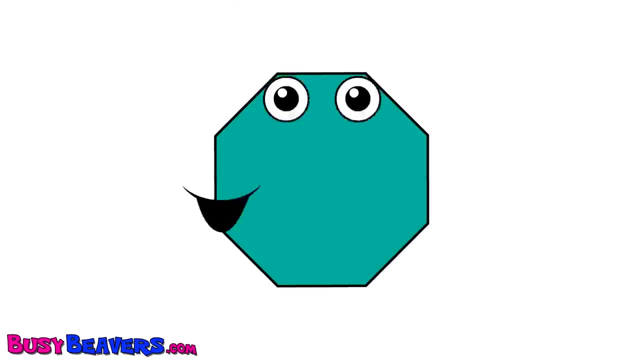 This little hexagon has seven sides: One, two, three, four, five, six, seven. This little octagon has eight sides. This little octagon has eight sides. This little octagon has eight sides: One, two, three, four, five, six, seven, eight. 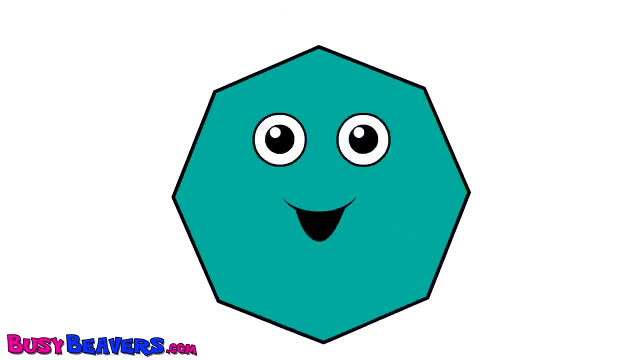 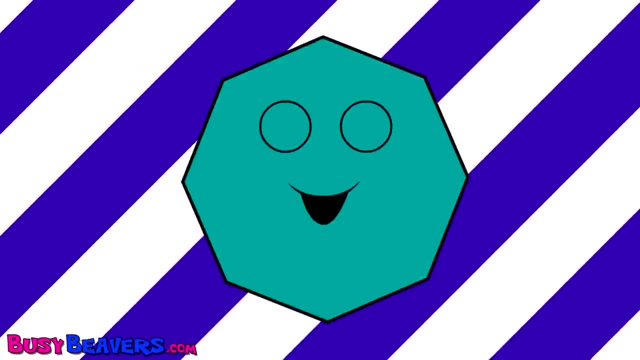 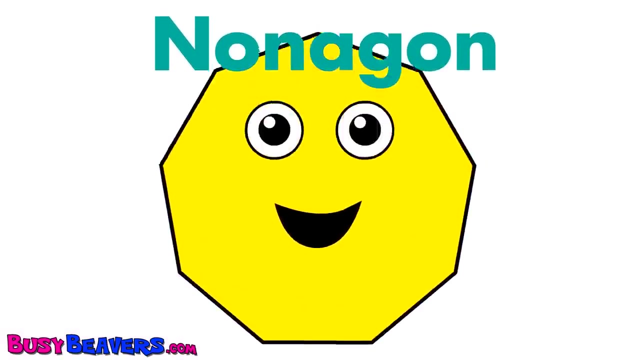 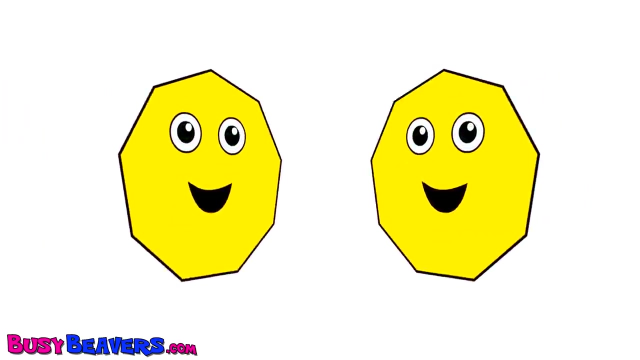 This little monogon has nine sides. This little monogon has nine sides. This little monogon has nine sides: 1, 2,, 3, 4,, 5,, 6,, 7, 8.. 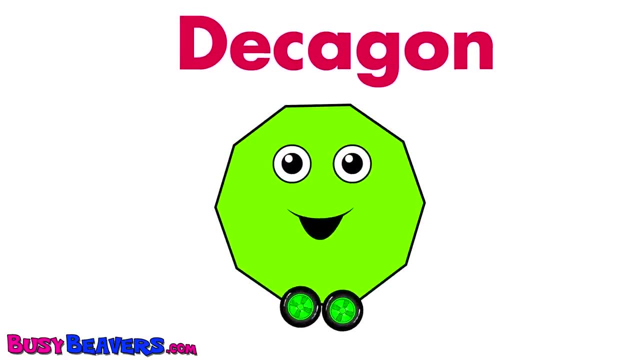 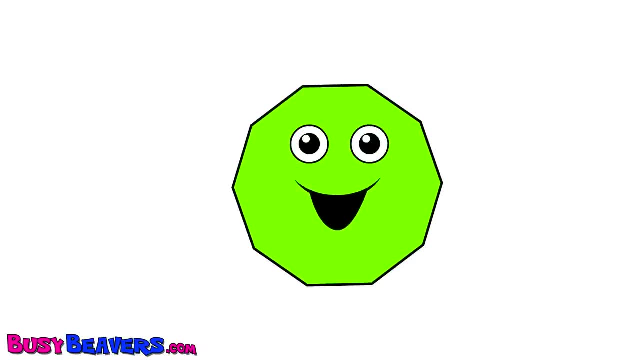 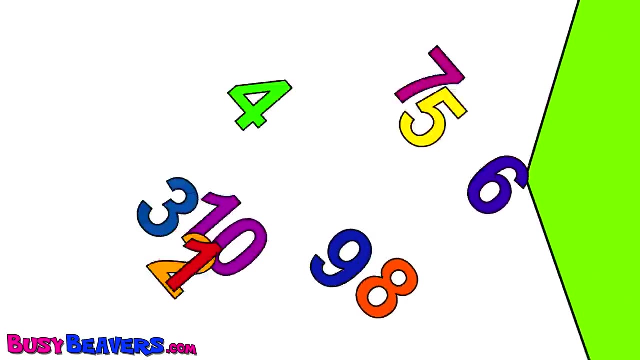 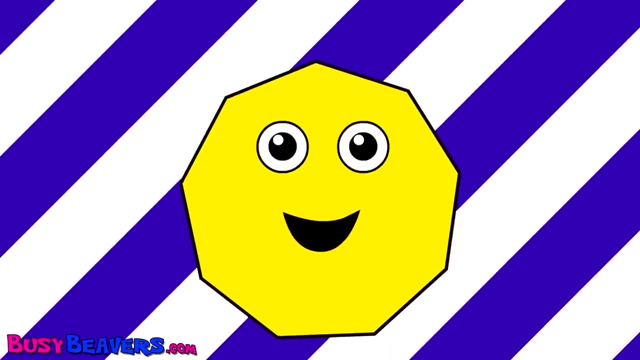 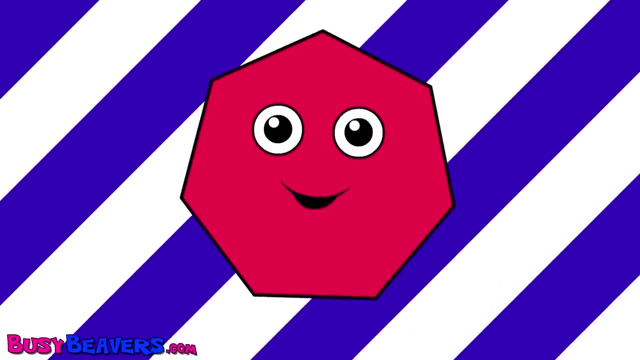 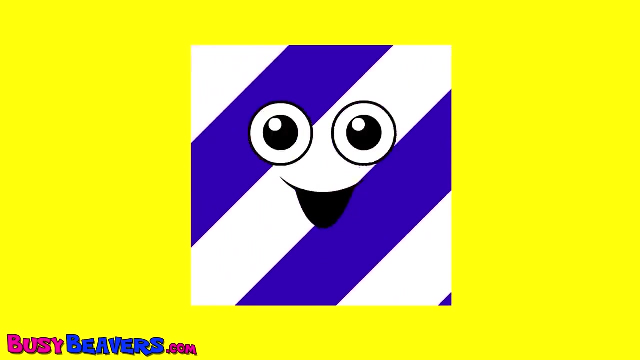 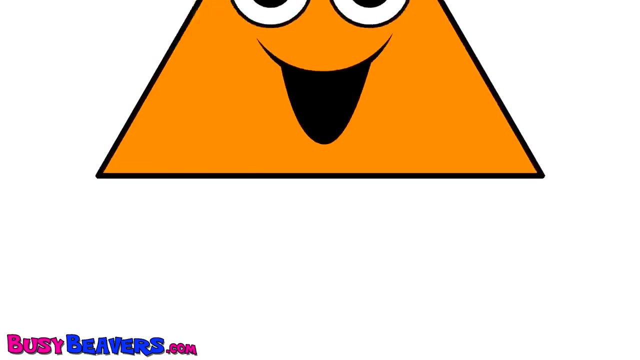 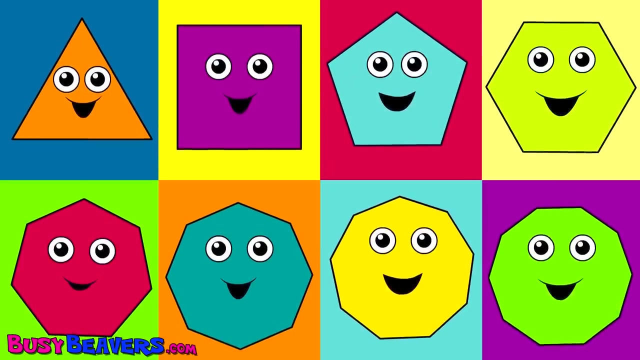 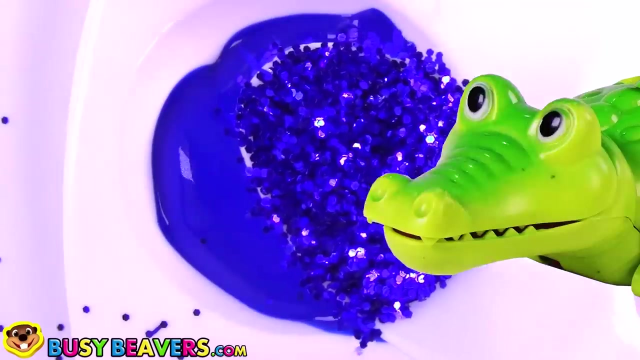 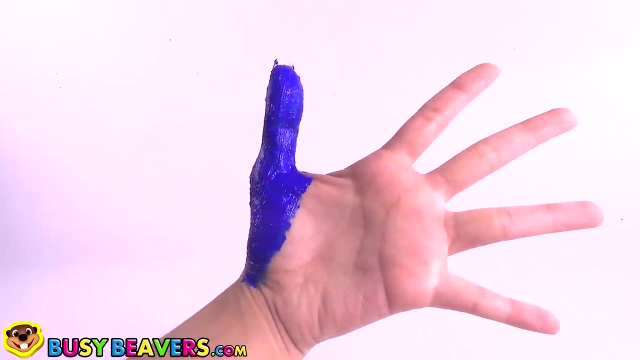 This little decagon has ten sides: One, two, three, four, five, six, seven, eight, nine, ten, Wow, Boom, boom, boom, boom. Very, very good, Very good, Daddy Blue Blue. 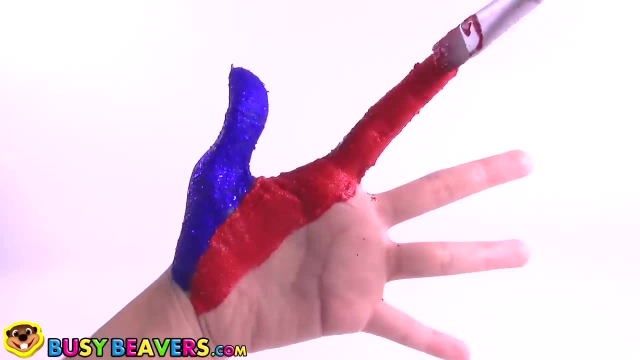 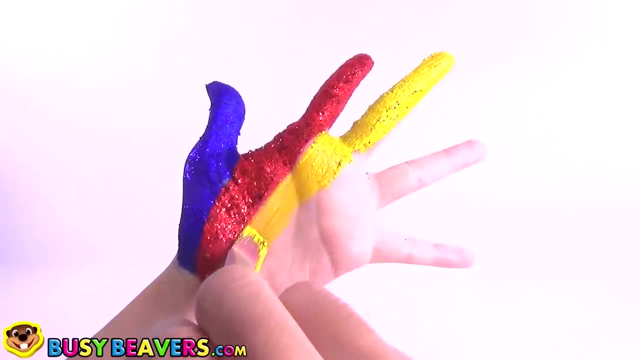 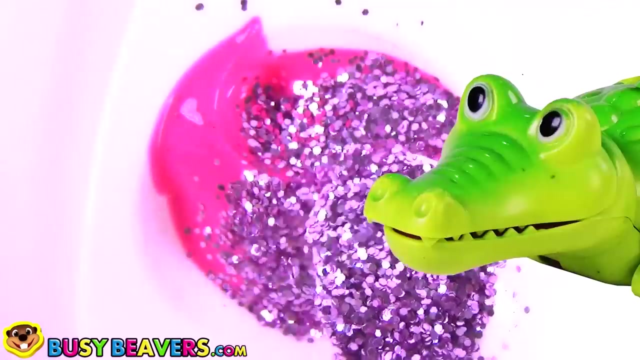 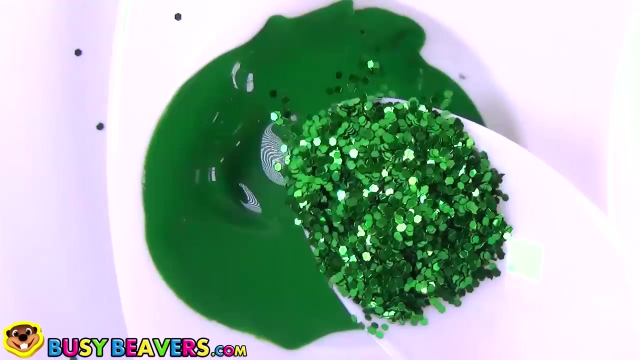 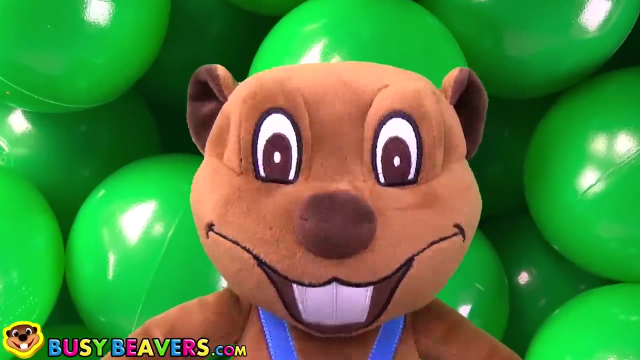 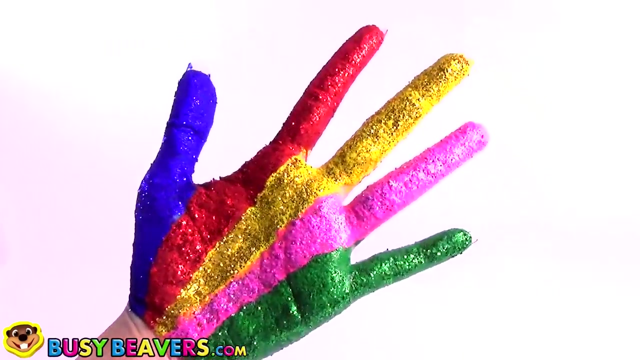 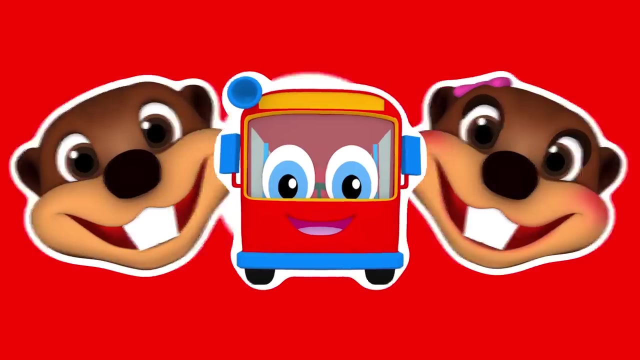 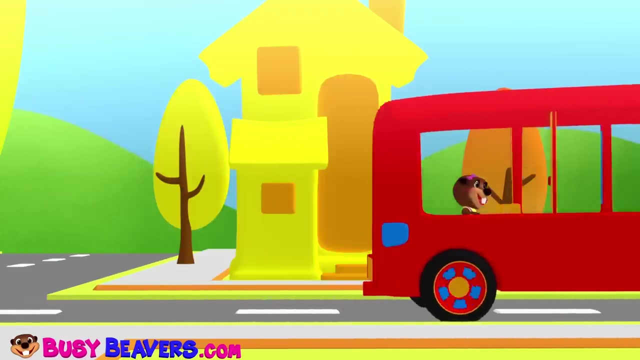 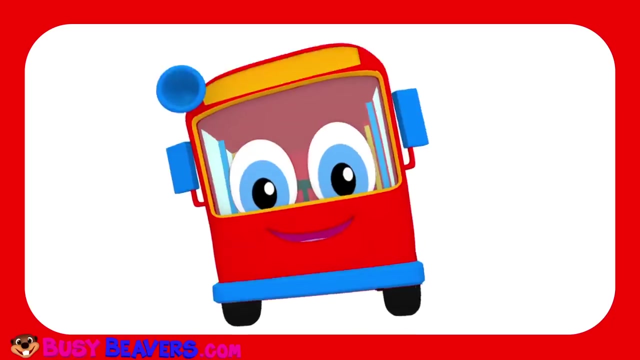 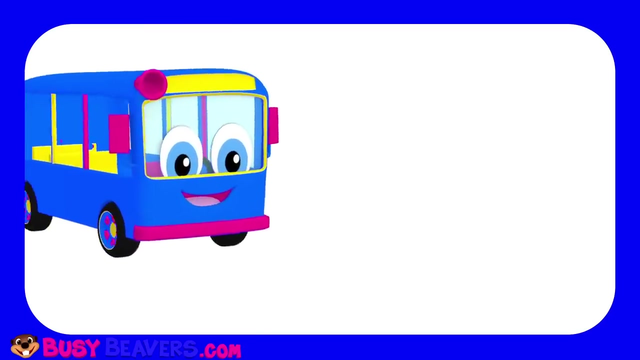 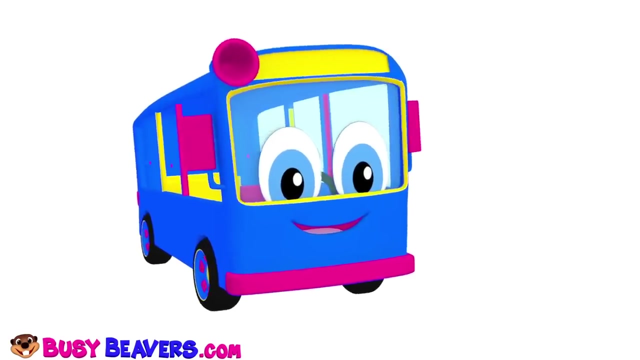 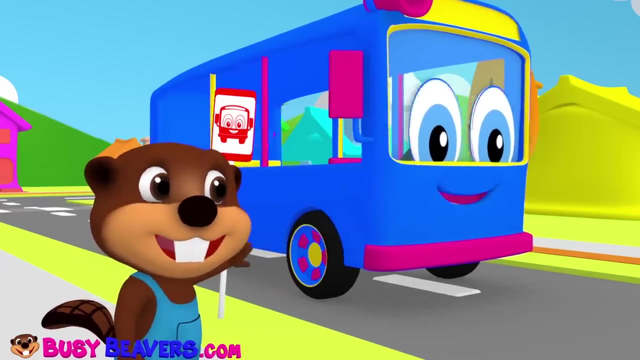 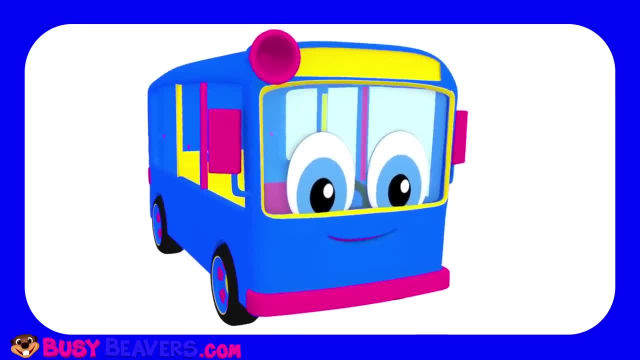 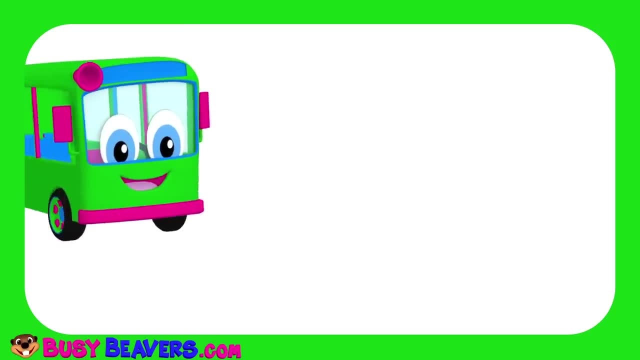 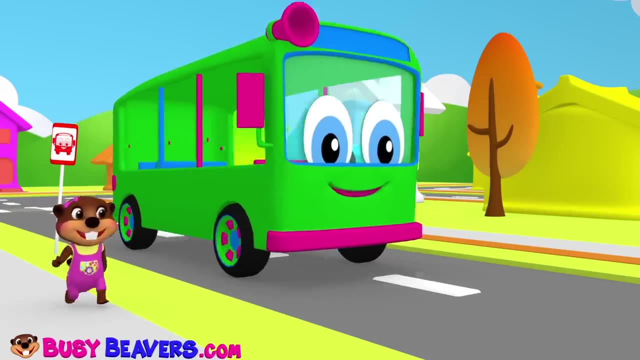 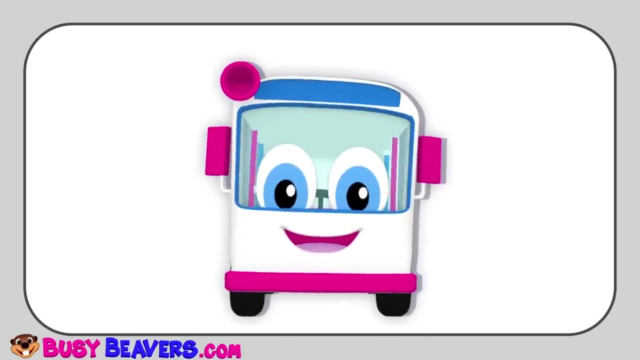 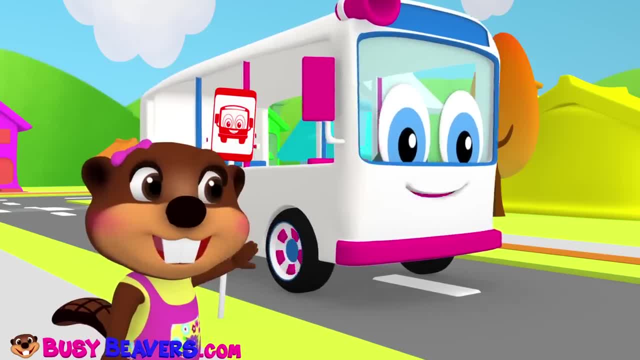 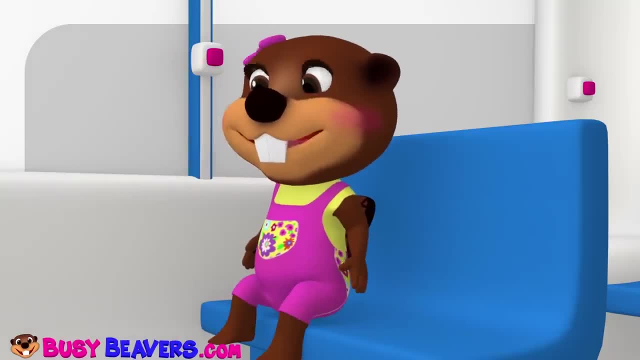 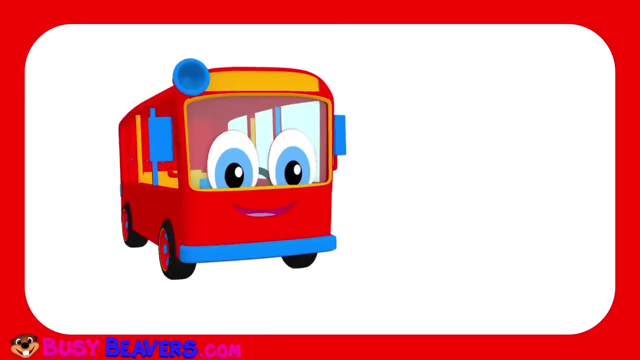 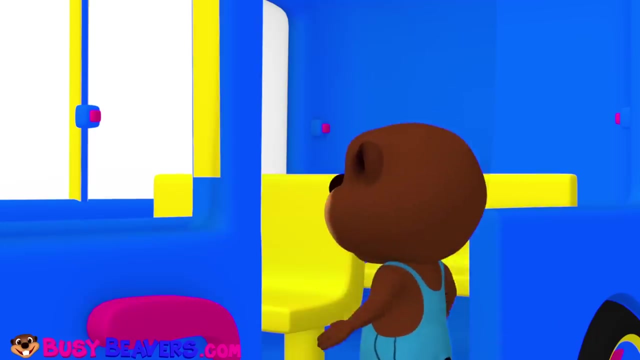 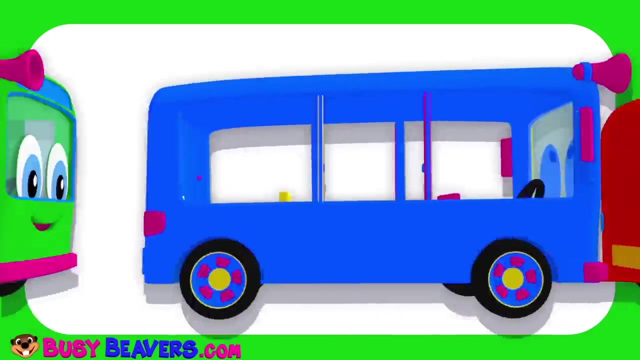 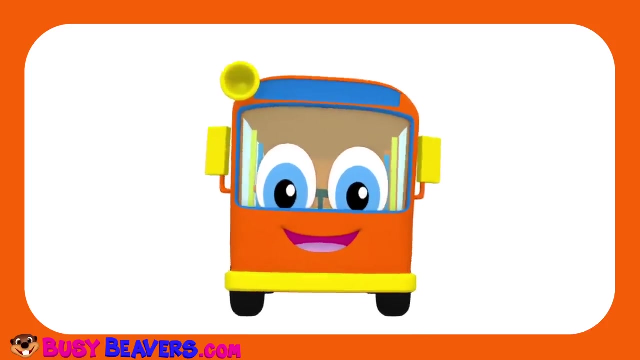 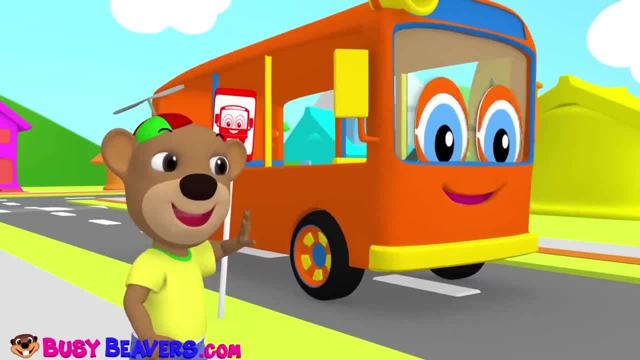 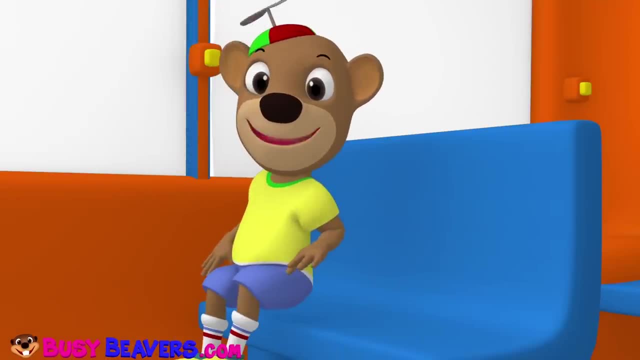 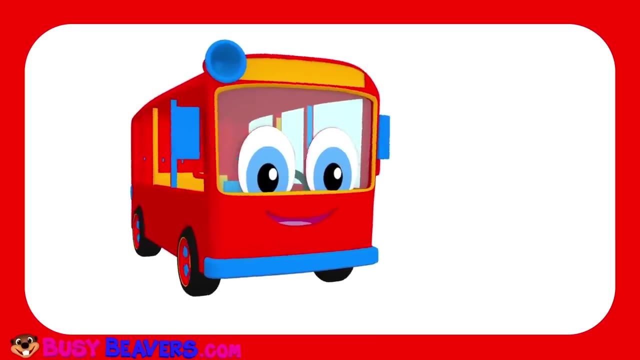 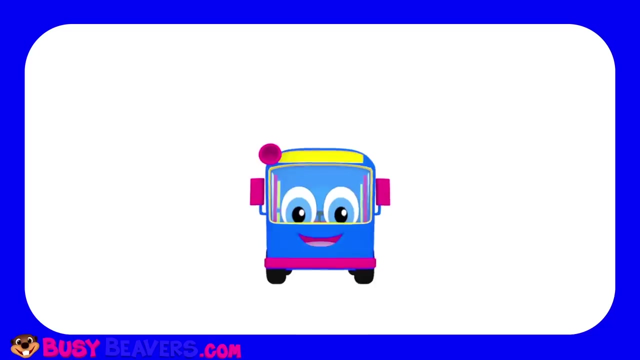 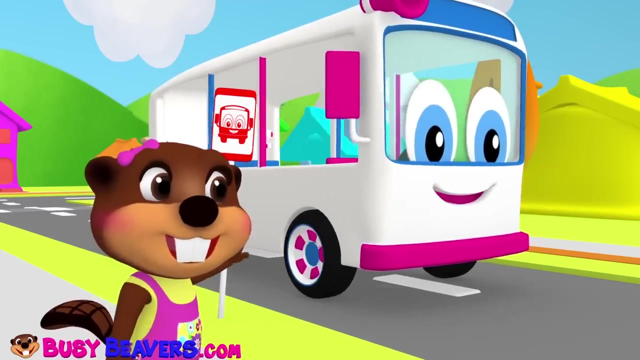 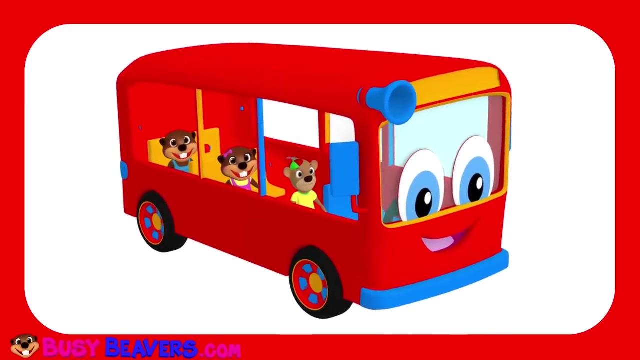 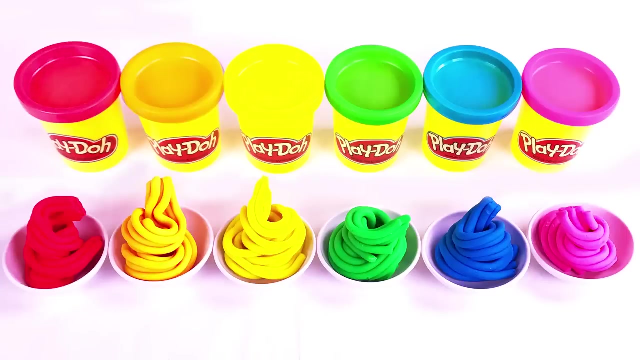 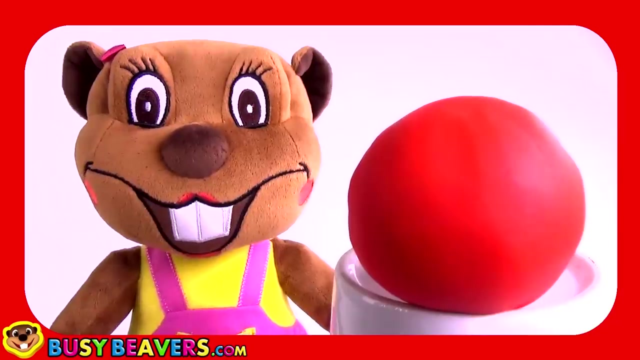 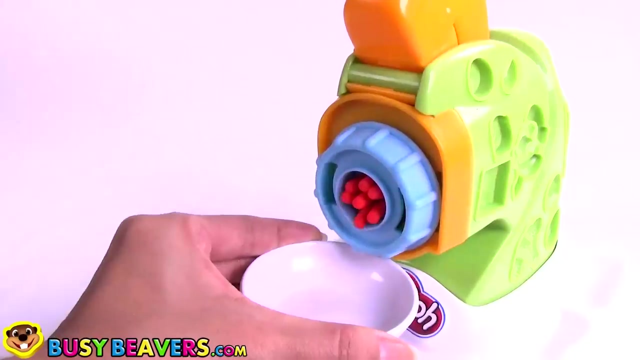 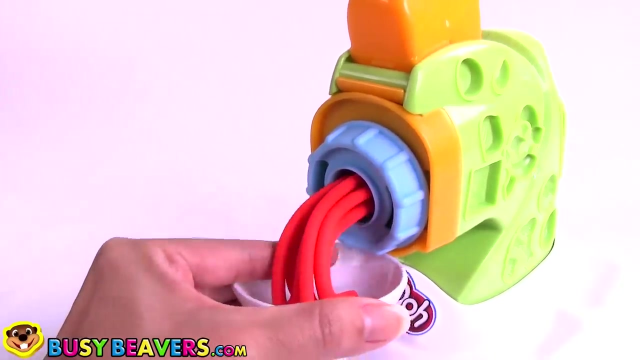 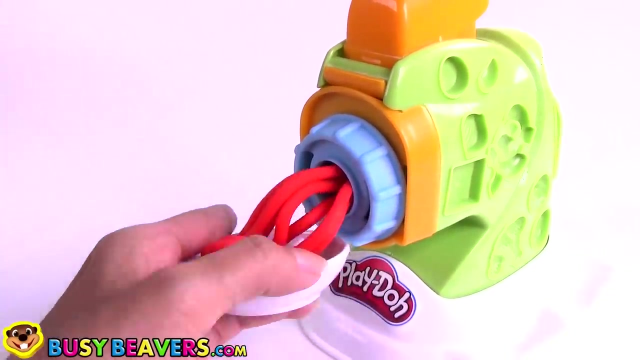 Orange bus. orange bus wait for me. Thank you, You're welcome. Thank you, You're welcome. Play-Doh Colors: Spaghetti Red. Yum, yum, Yummy, Yummy-yummy, Yummy-yummy. 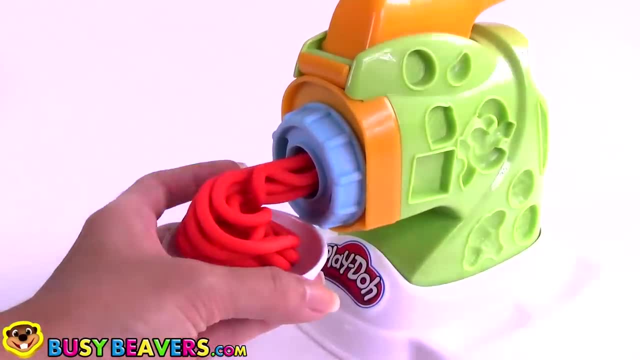 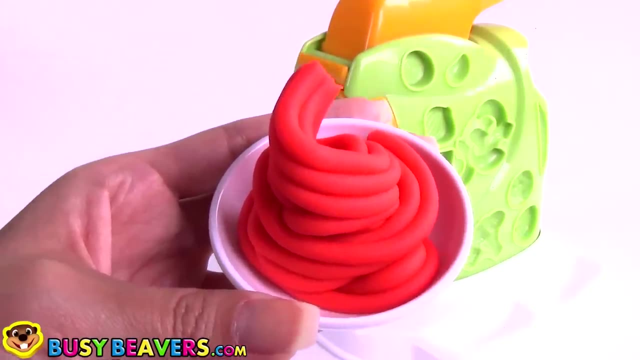 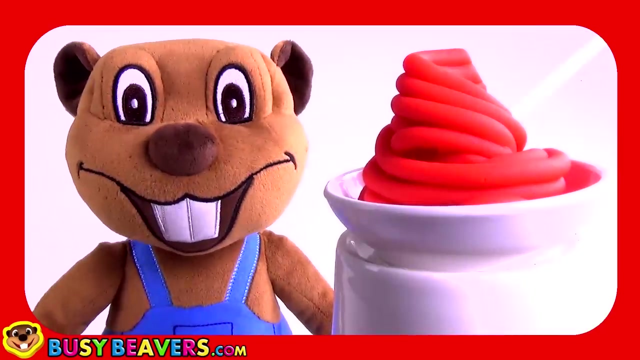 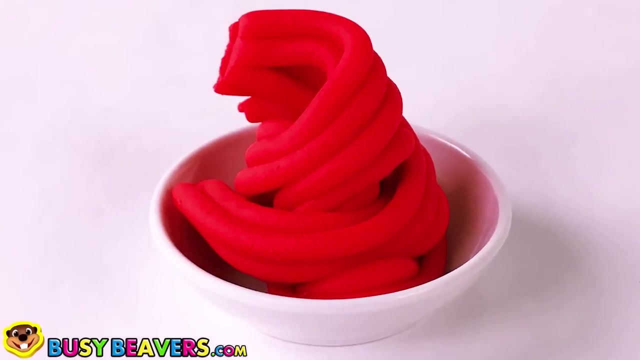 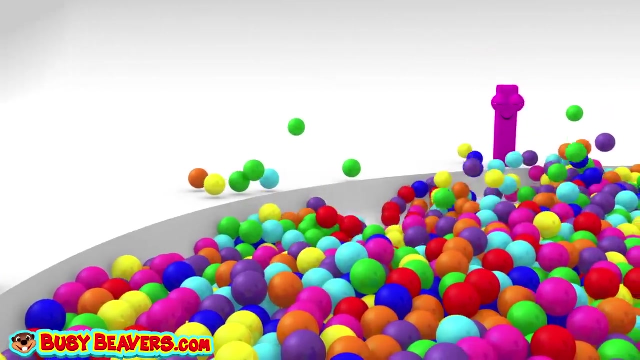 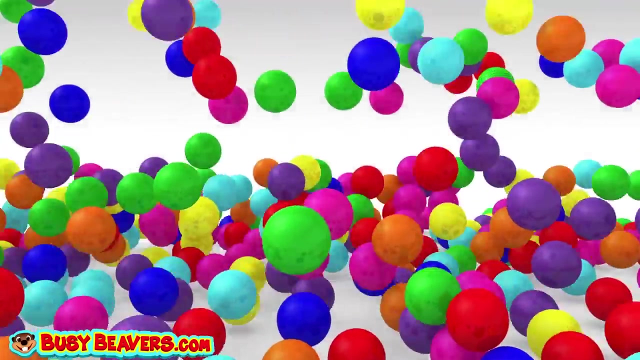 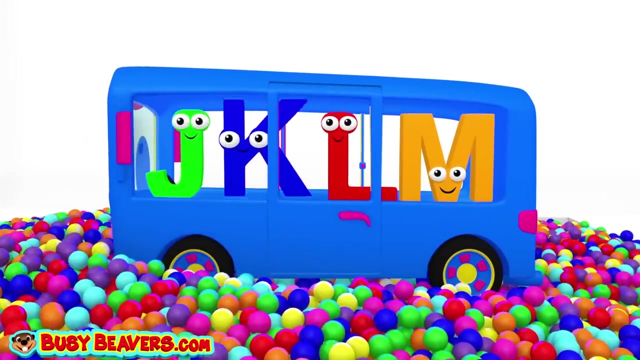 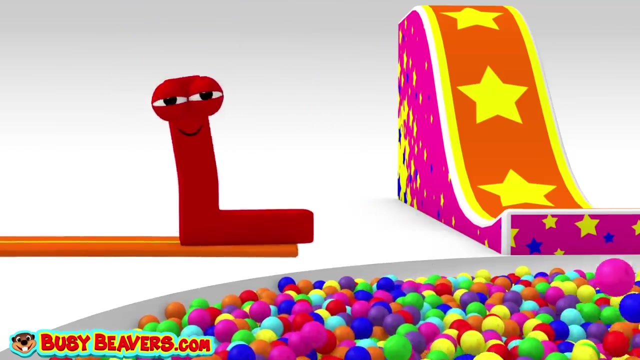 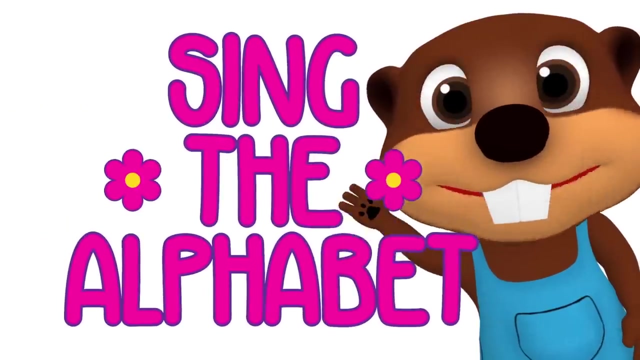 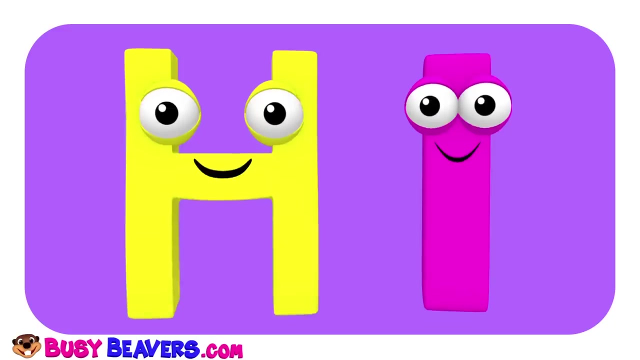 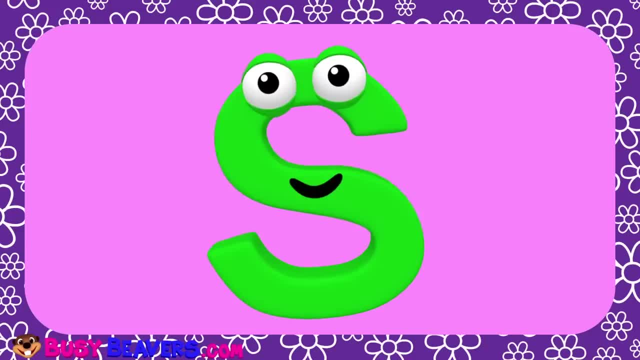 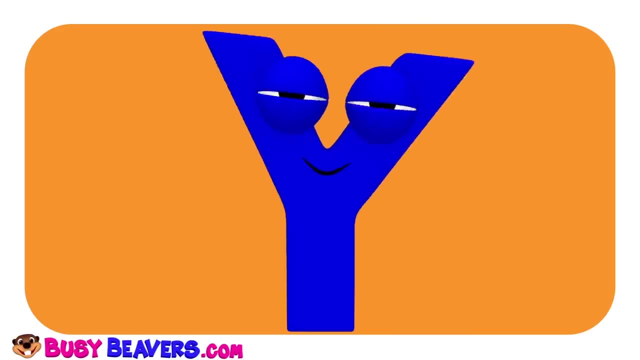 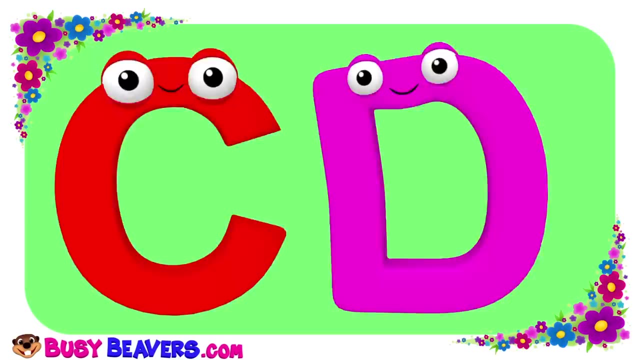 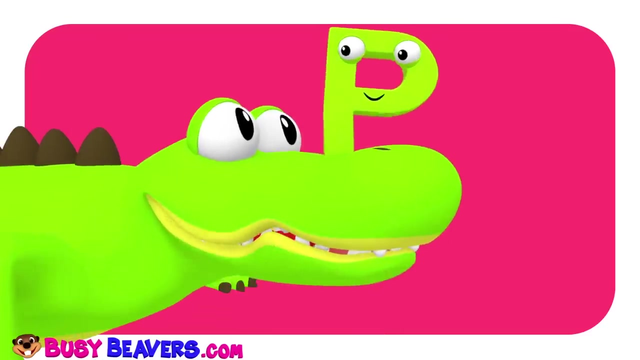 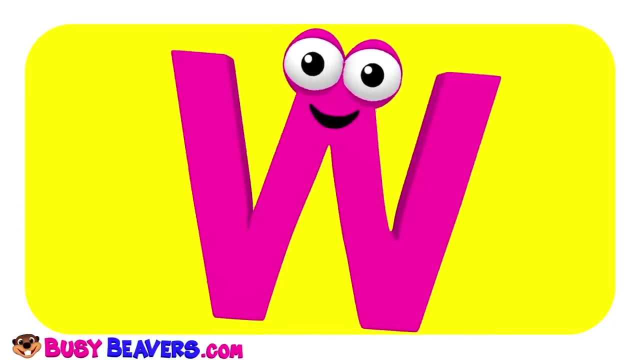 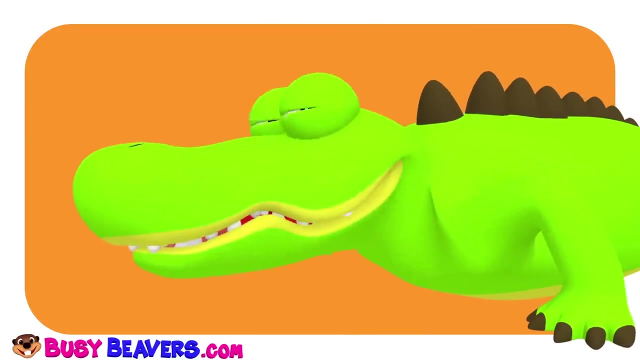 L M N O P Q R S T U V, W, X, Y and Z Again, A, B, C, D, E, F, G, E, H, I, J, K. L M N O P Q R S T U V, W, X, Y and Z. Can you do it? 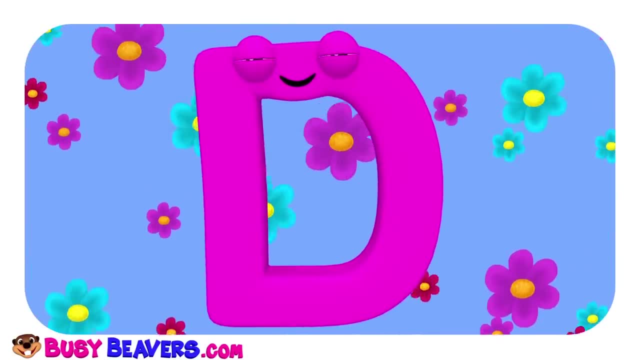 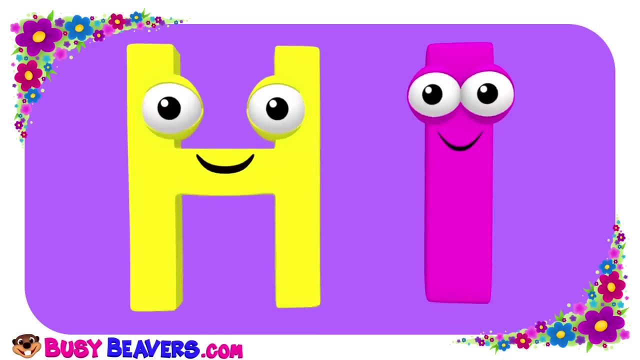 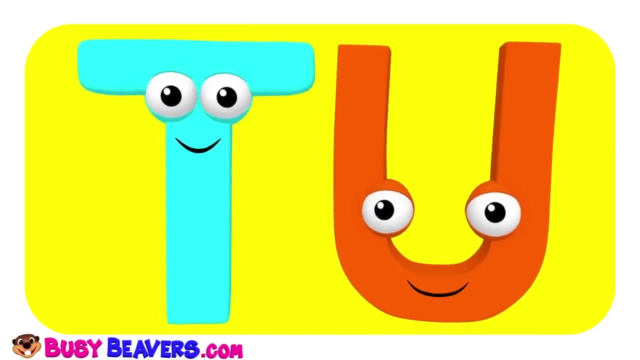 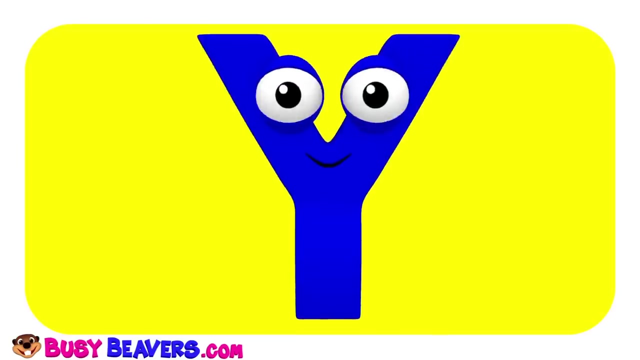 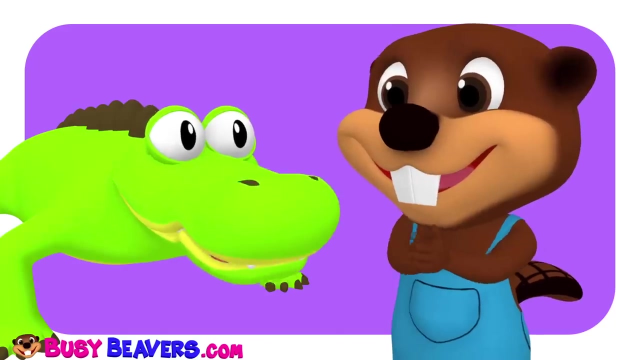 It's easy, I'm going to sing it with you this time. Here I go: A, B, C, D, E, F, E, F, G, H, I, J, K, L, M, N, O, P, Q, R, S, T, U, V, W, X, Y and Z. I did a very good job. 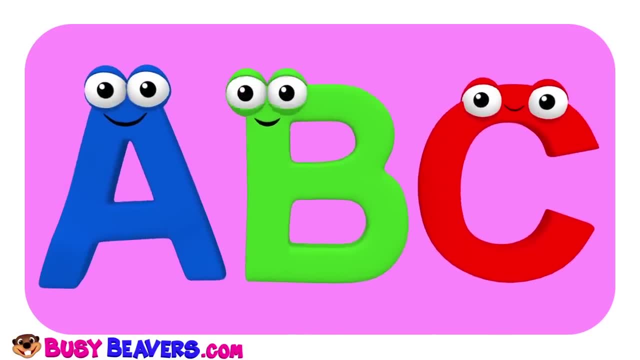 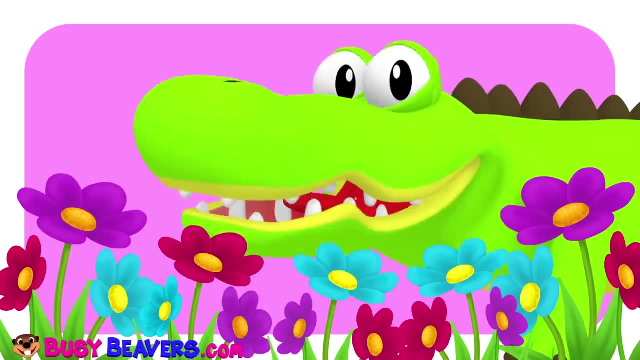 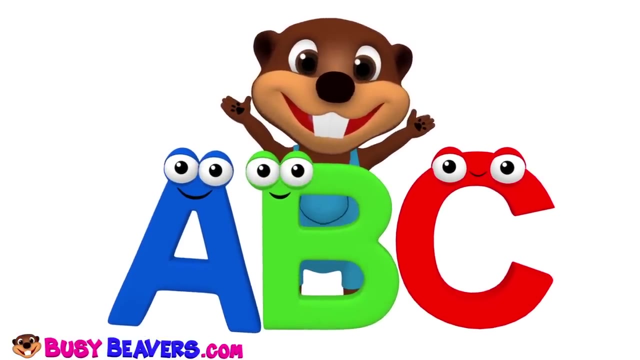 Did you hear me? I was good. Yes, Oh yes. How's that old guy And honey? Now say that one more time. Yes, H R I S T U series And the round's ready. Yet there's one final thing we want to talk about. 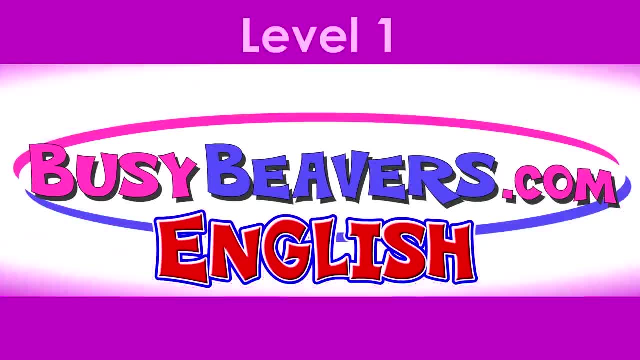 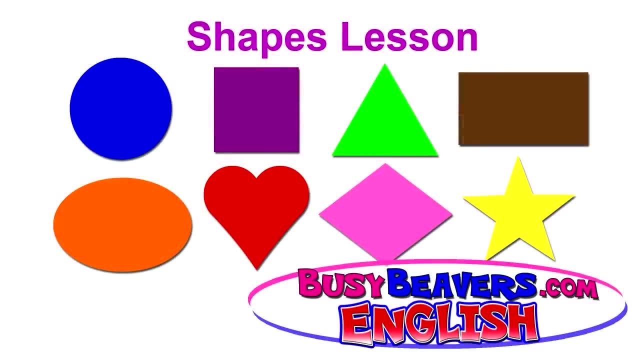 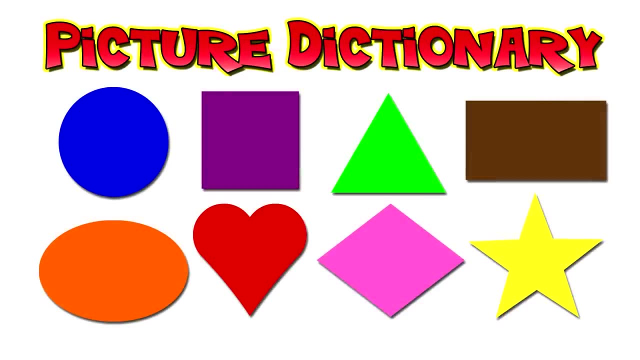 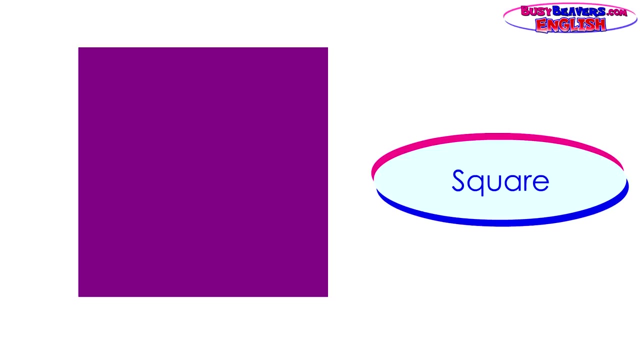 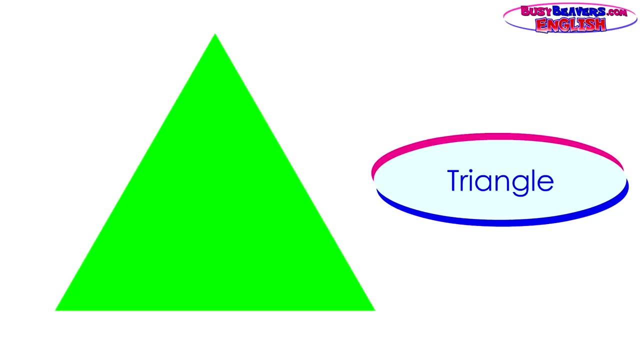 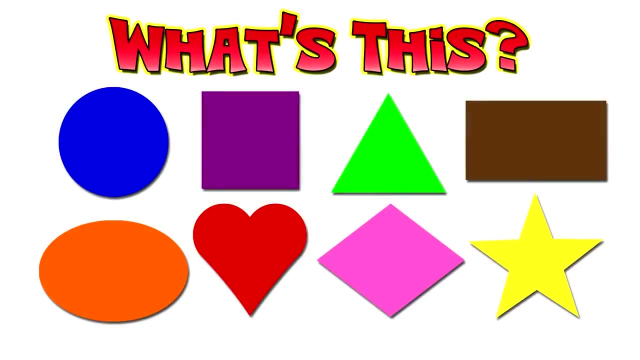 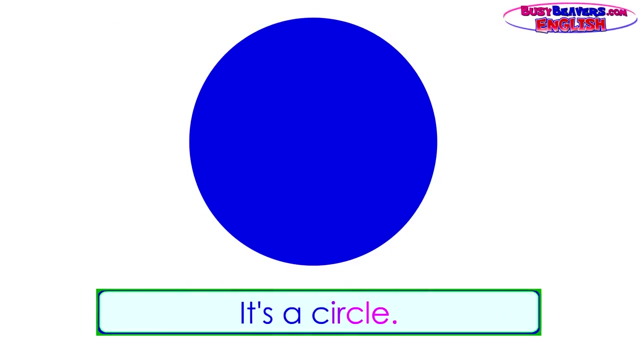 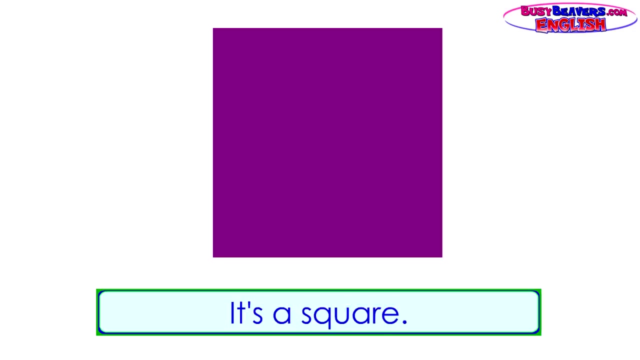 I hope you will enjoy this video. I've got to make a brand new one for you. Shapes, Lesson, Circle, Square, Triangle, Rectangle, Oval, Heart, Diamond Star. What's this? It's a circle. What's this? It's a square. What's this? 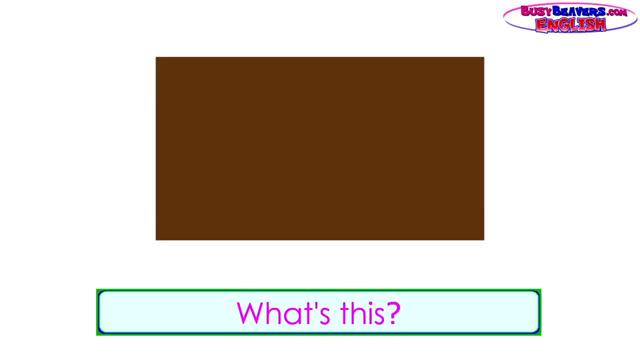 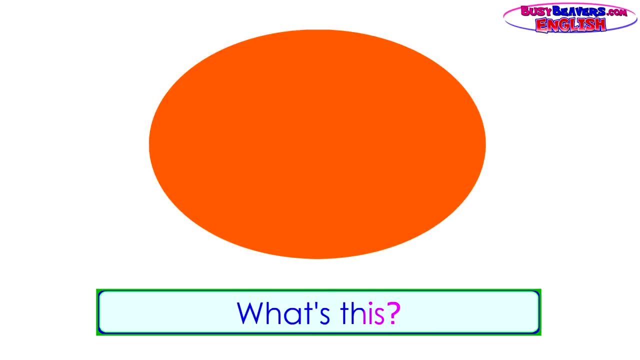 It's a triangle. What's this? It's a rectangle. What's this? It's an oval. What's this? It's a heart. What's this? It's a diamond. What's this? It's a star. It's a diamond. 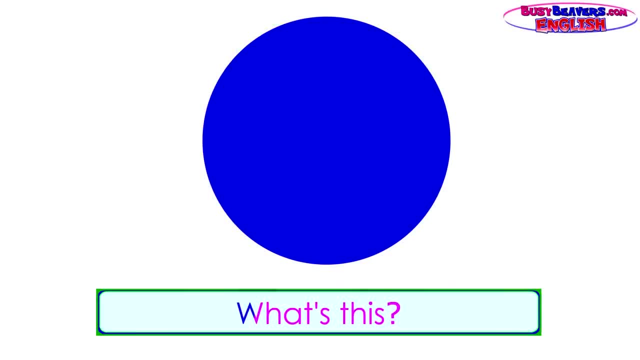 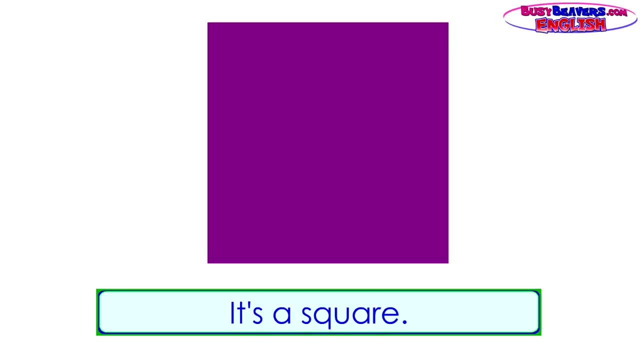 It's a diamond. It's a diamond. What's this? It's a circle. What color is the circle? The circle is blue. What's this? It's a square. What color is the square? The square is purple. What's this? 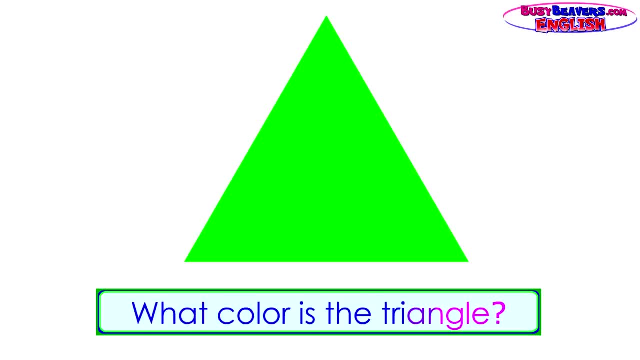 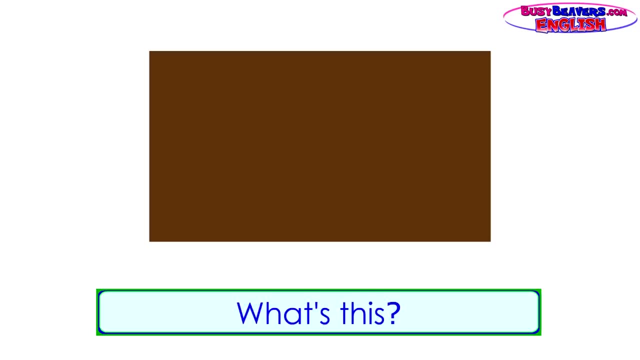 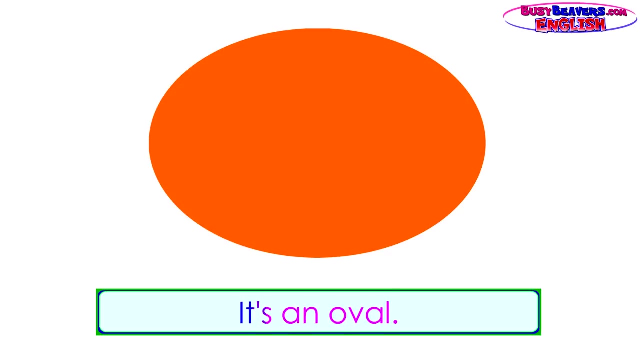 It's a triangle. What color is the triangle? The triangle is green. What's this? It's a rectangle. What color is the rectangle? The rectangle is brown. What's this? It's an oval. What color is the oval? 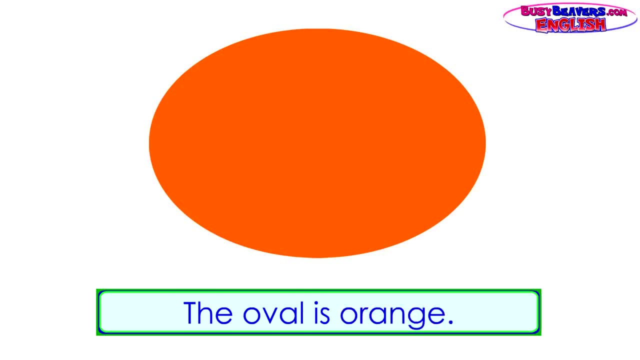 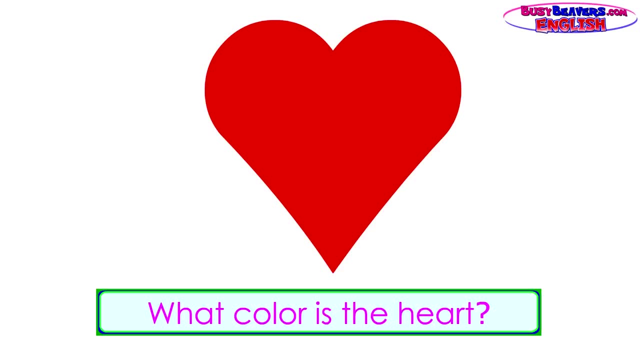 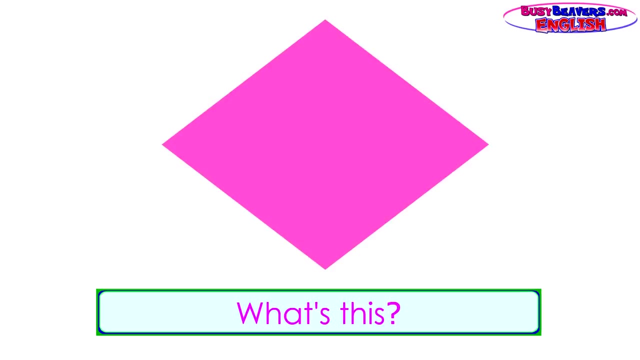 The oval is orange. What's this? It's a heart. What color is the heart? The heart is red. What's this? It's a diamond. What color is the diamond? The diamond is pink. What's this? It's a star. 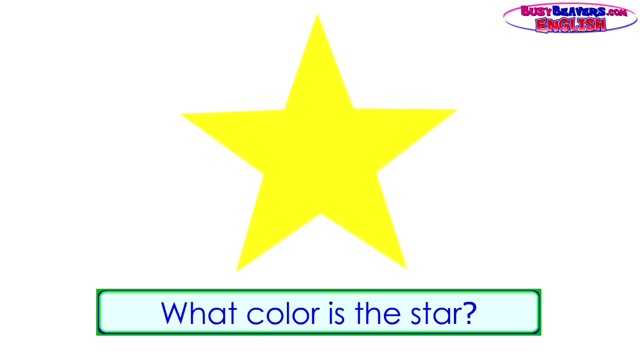 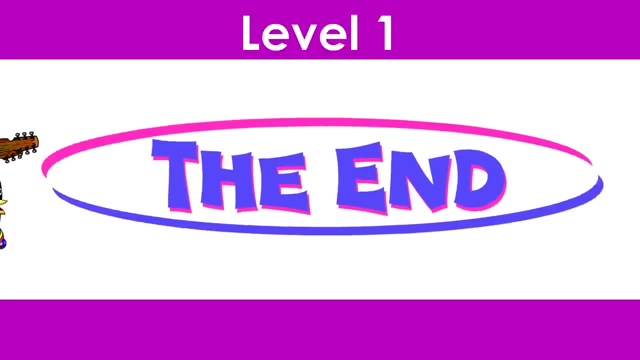 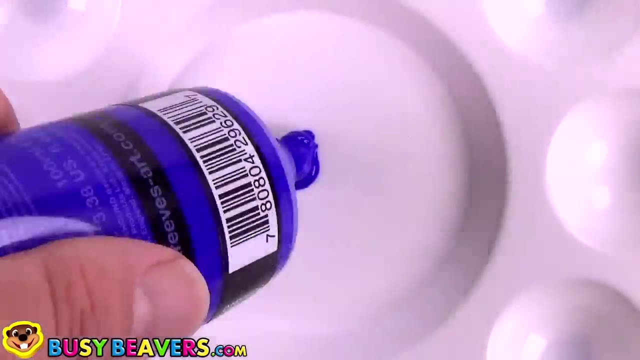 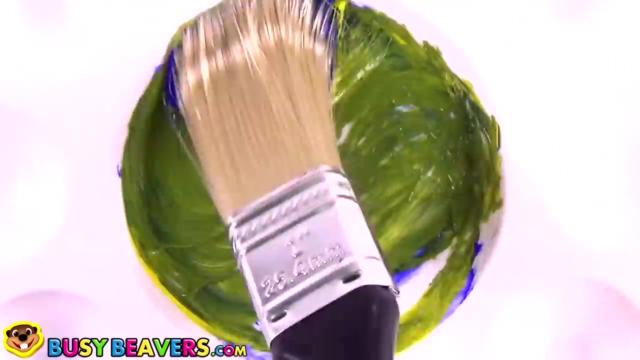 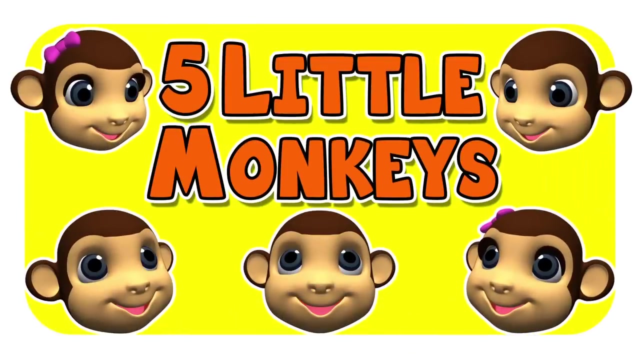 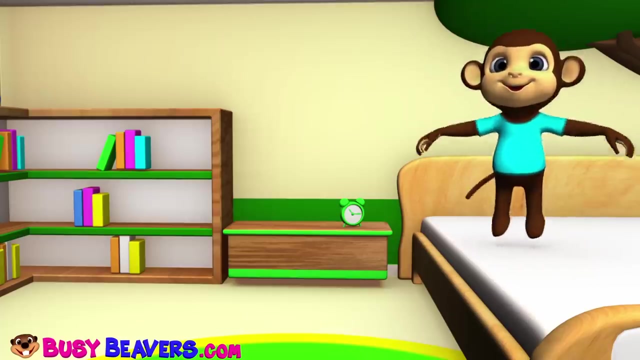 What color is the star? The star is yellow. What color is the star? The star is blue. What color is the star? The star is red. What color is the star? The star is blue. What color is the star? The star is red. 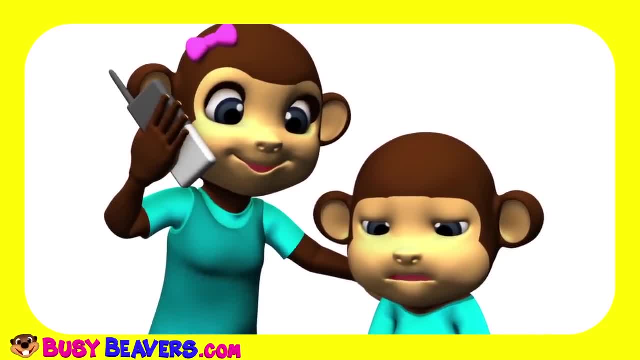 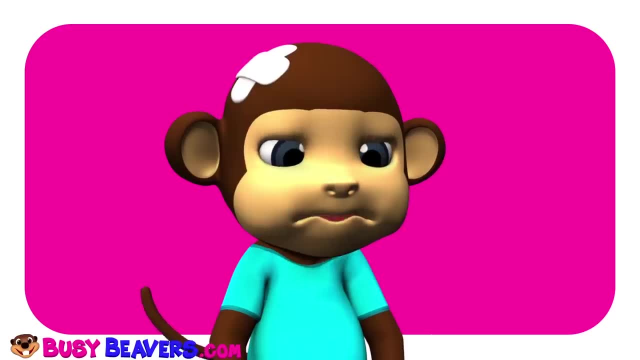 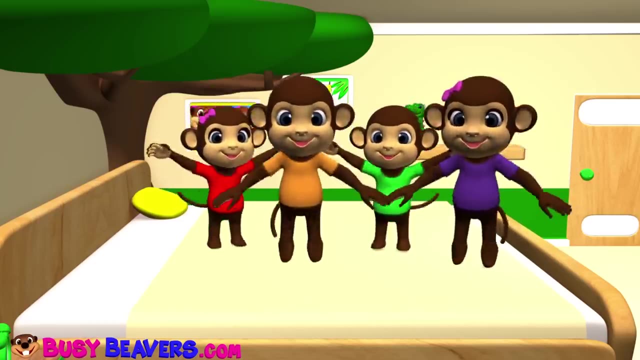 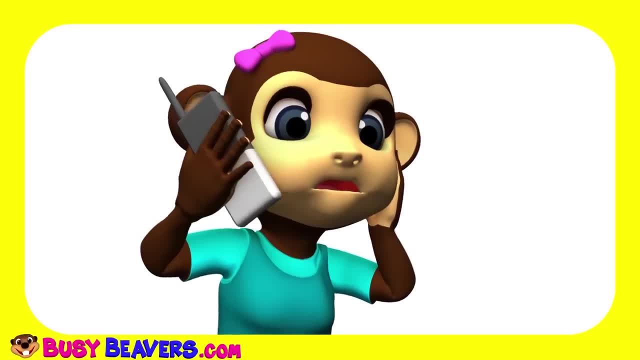 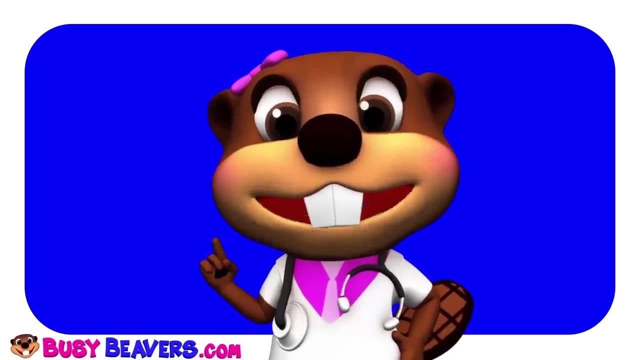 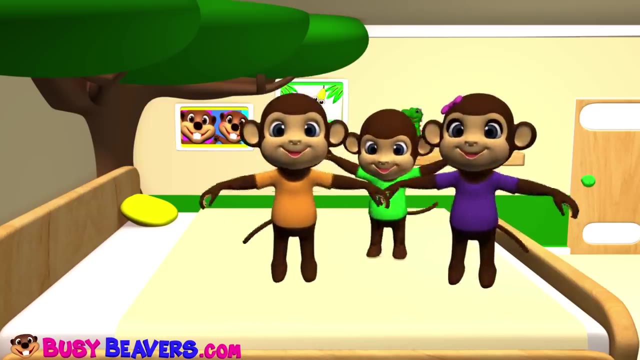 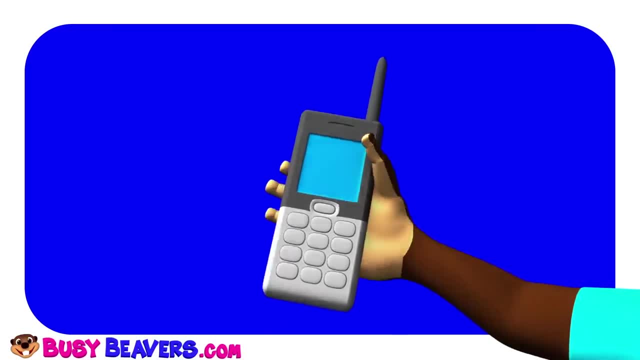 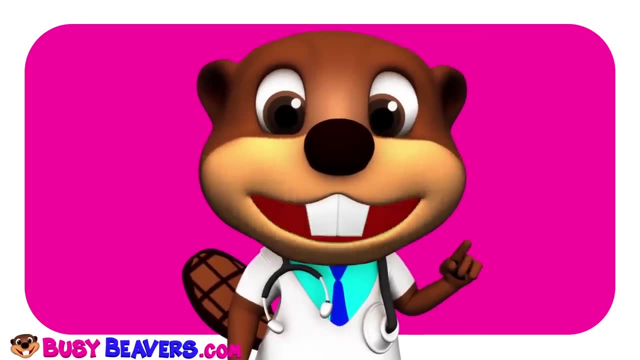 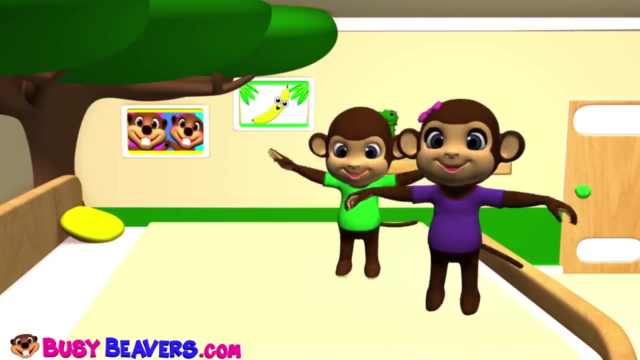 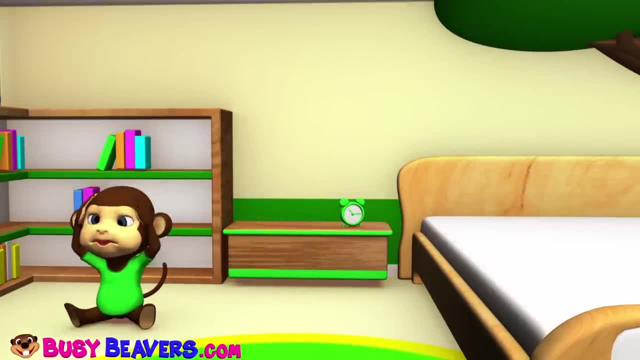 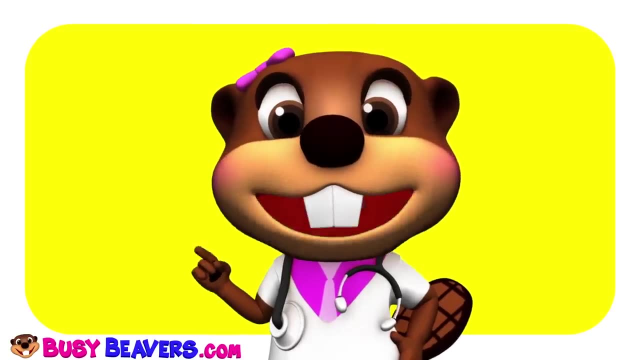 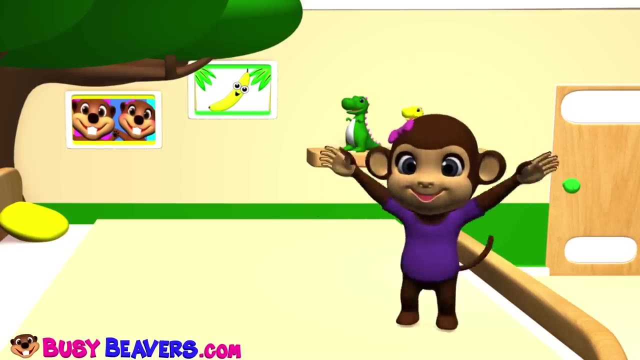 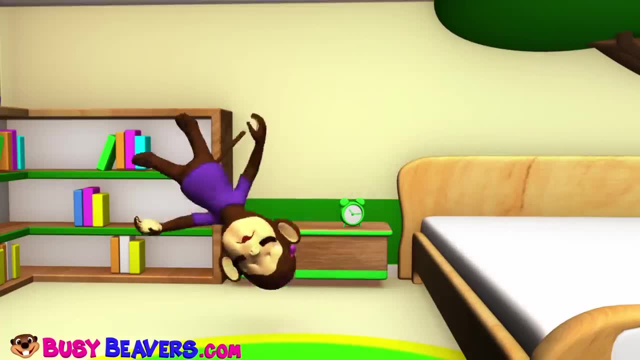 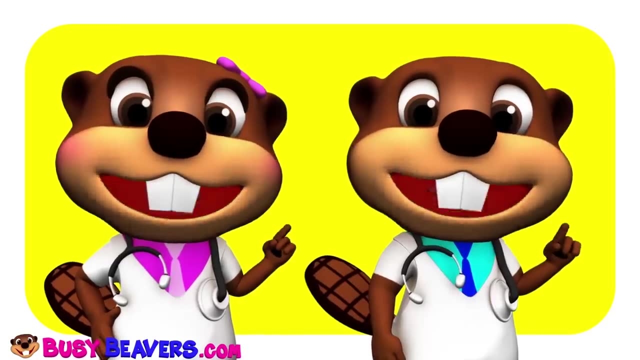 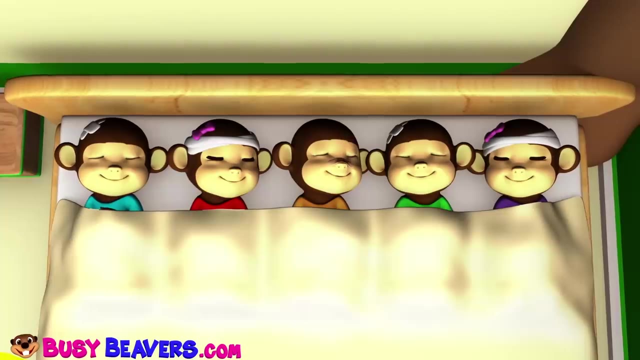 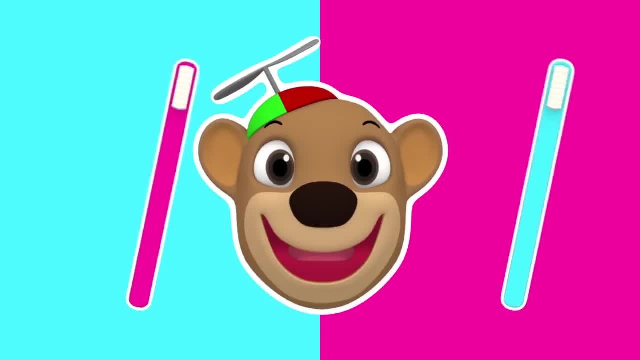 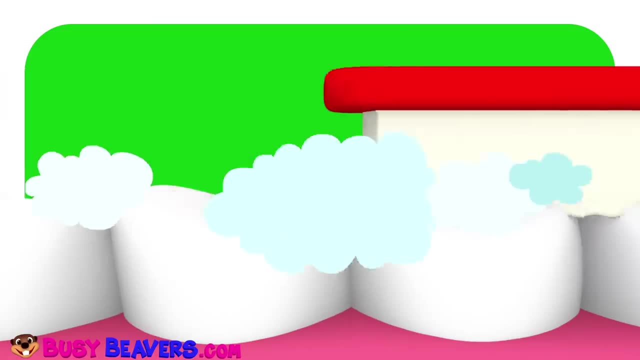 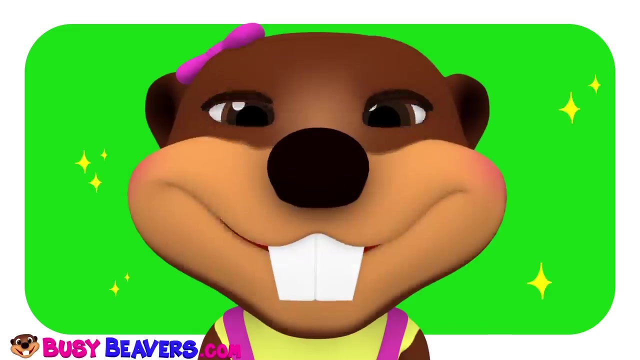 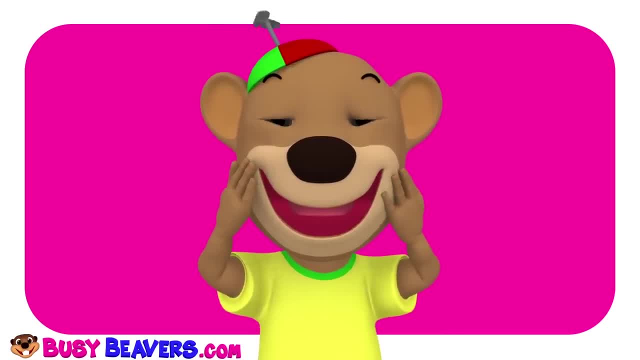 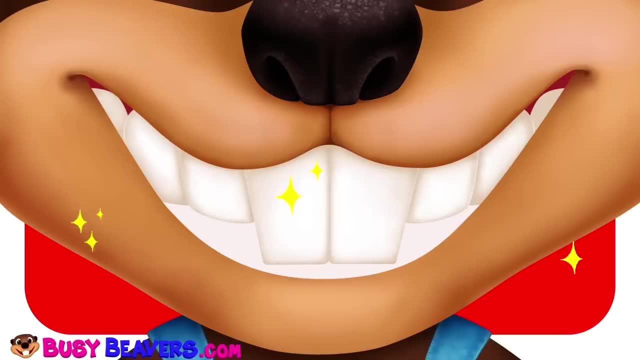 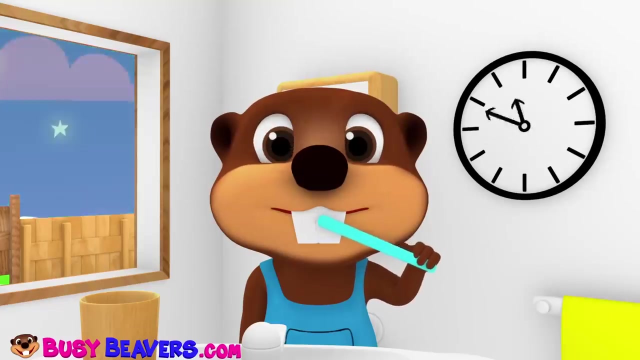 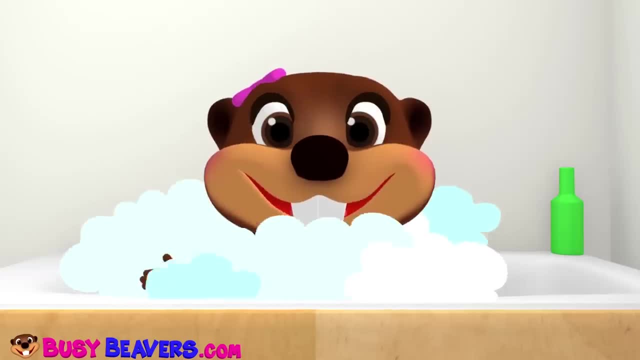 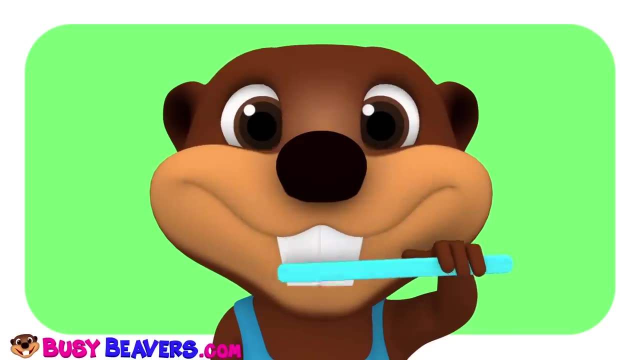 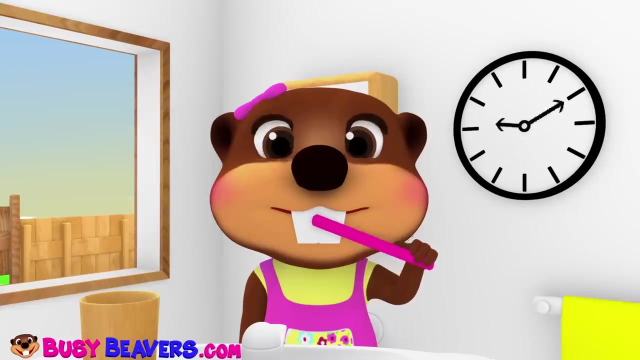 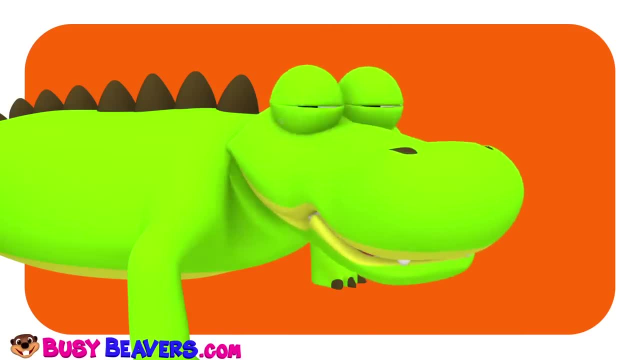 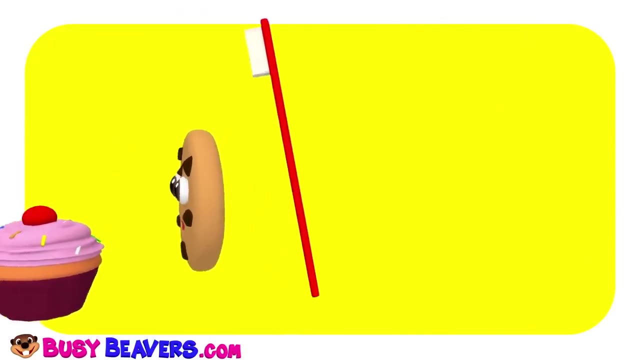 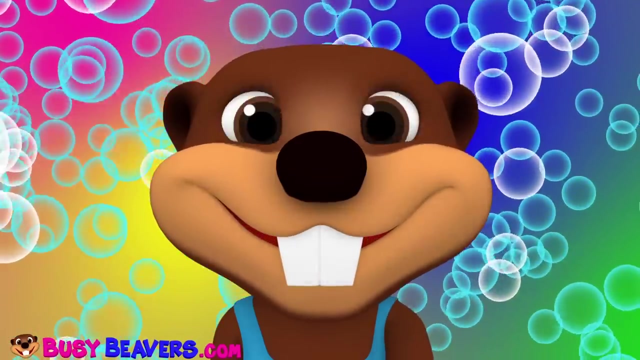 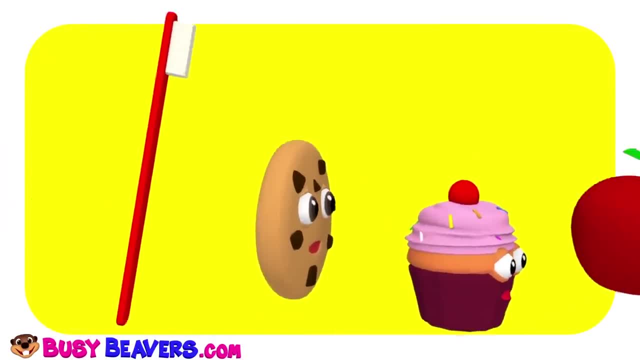 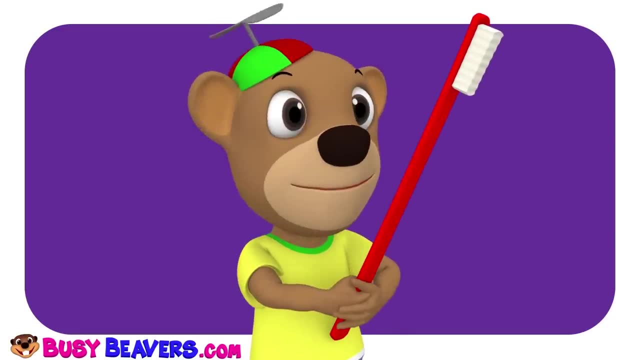 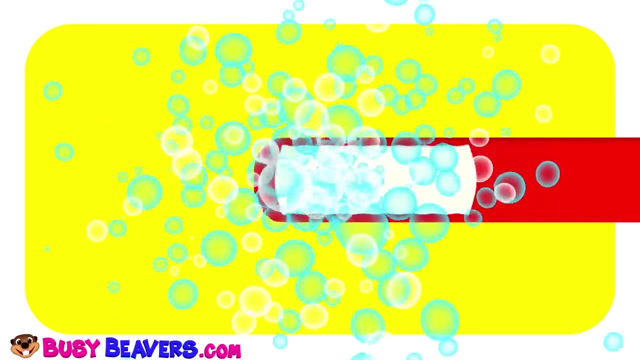 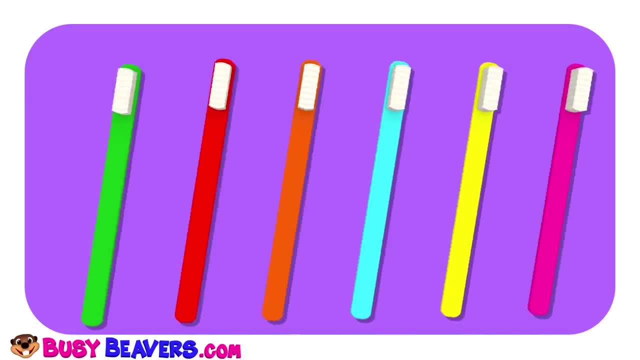 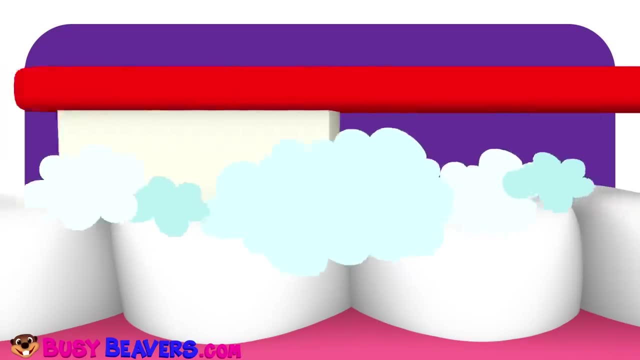 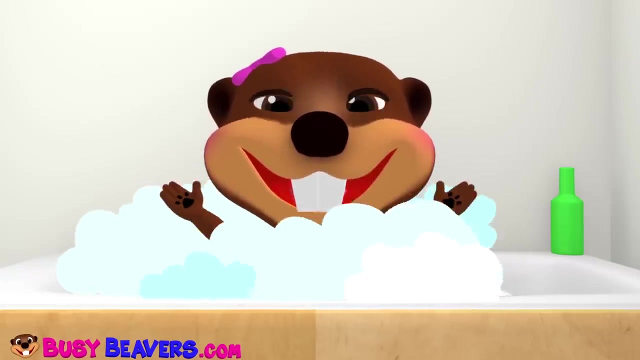 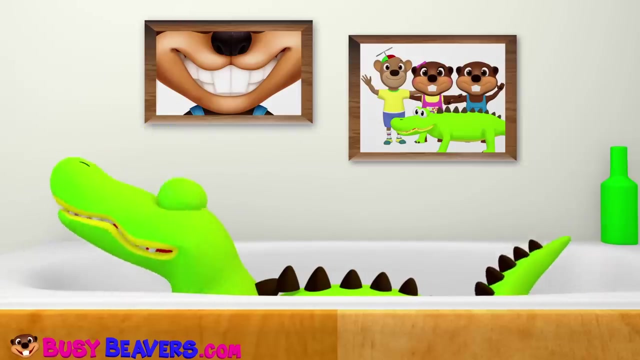 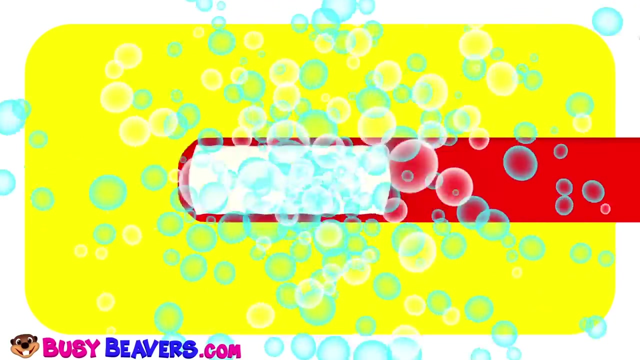 And then smile, smile, smile. Hey, yeah, my baby's got a beautiful smile, Smile, smile, smile. My baby's got a beautiful Smile, smile, smile. My baby's got a beautiful Smile, smile, smile. My baby's got a beautiful Smile, smile, smile. 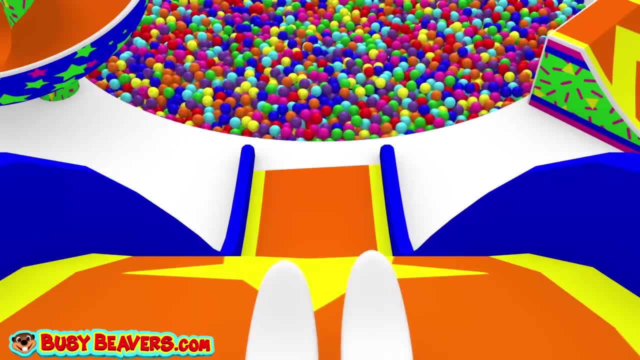 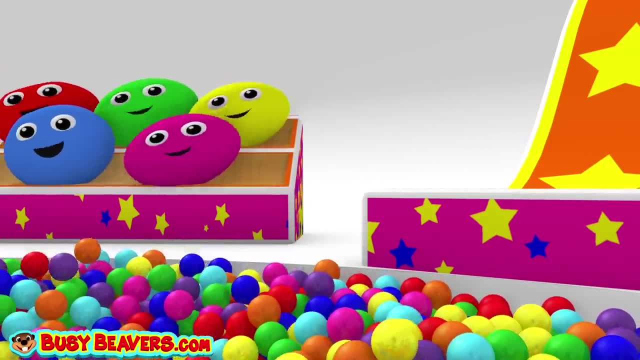 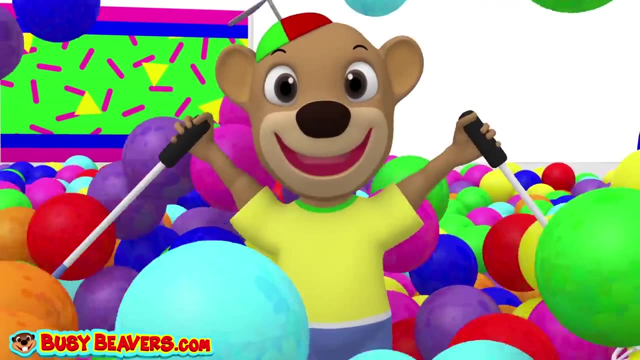 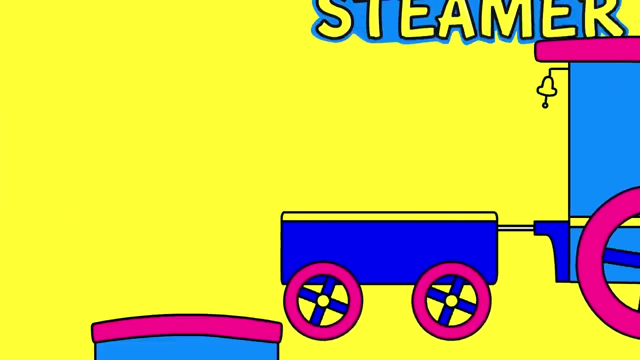 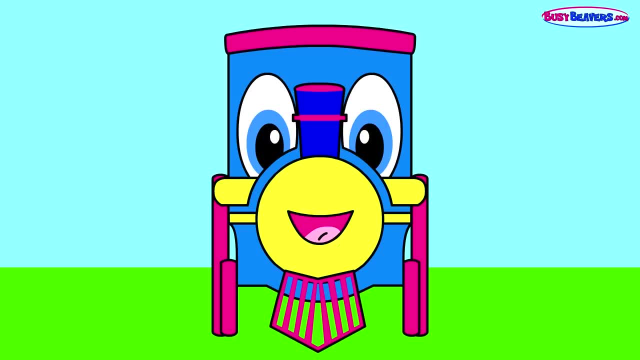 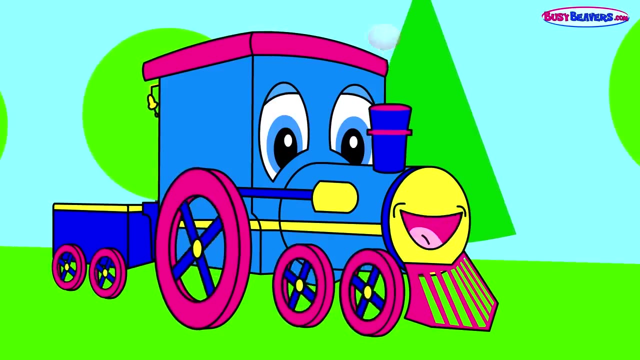 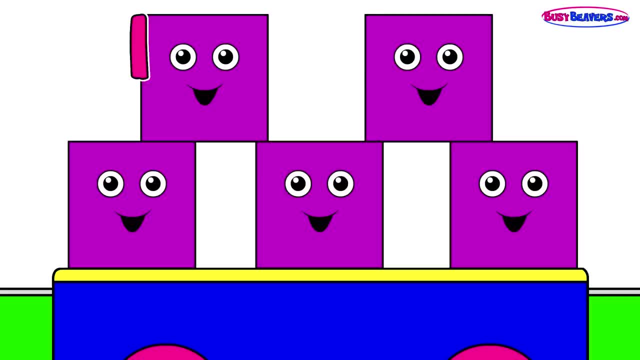 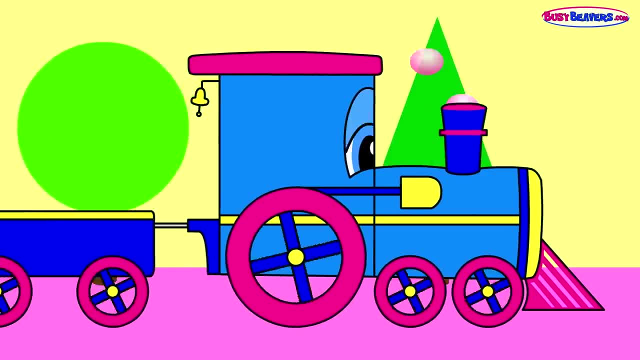 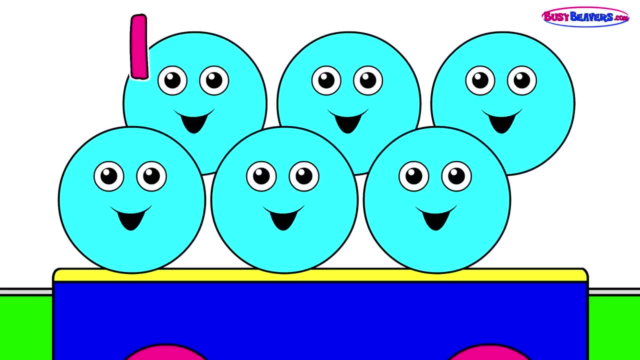 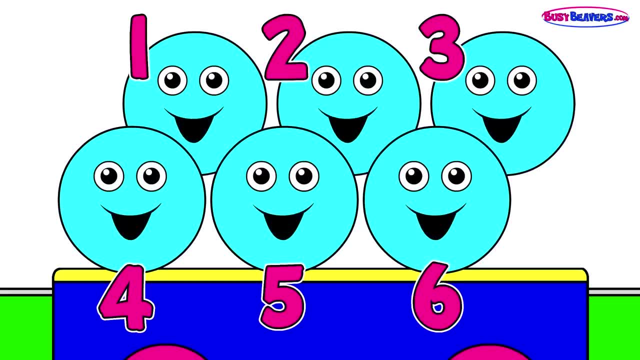 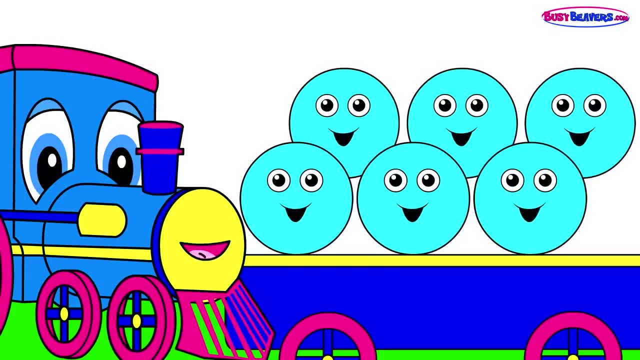 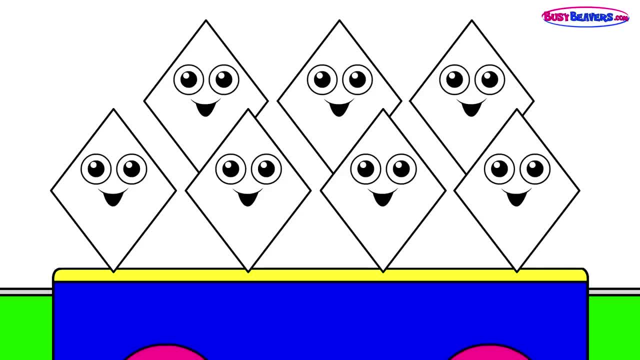 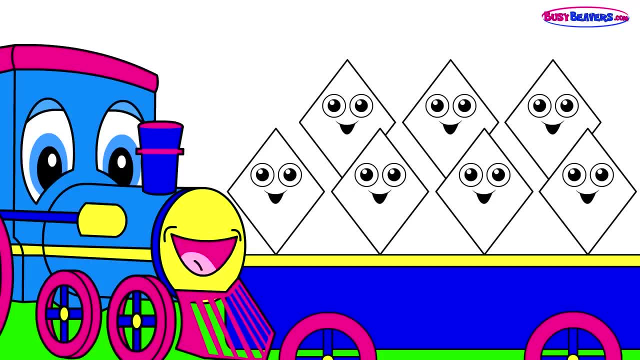 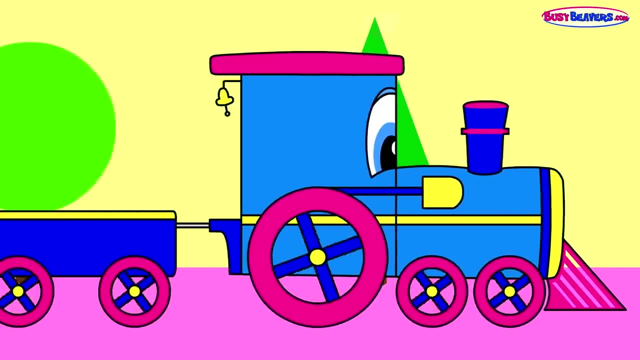 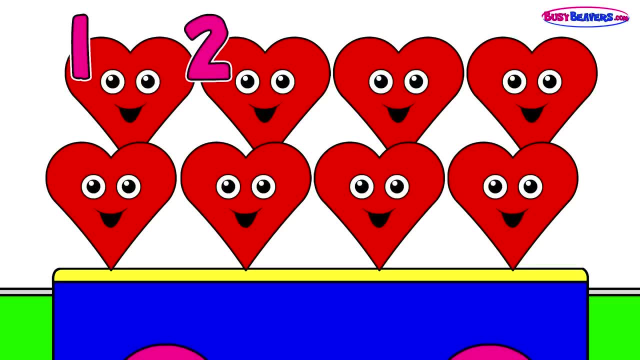 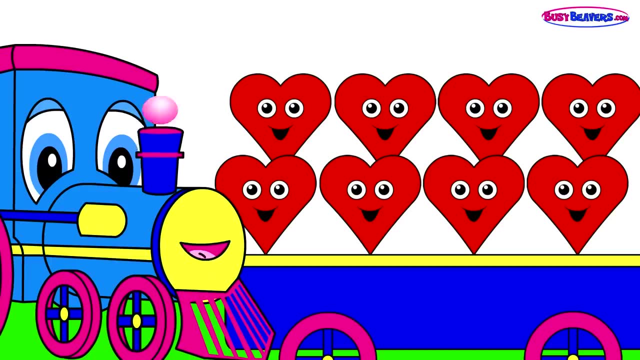 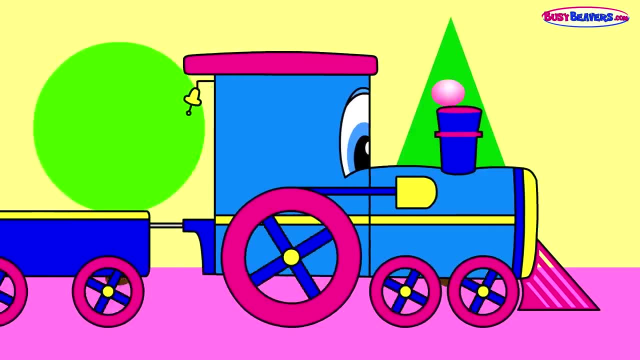 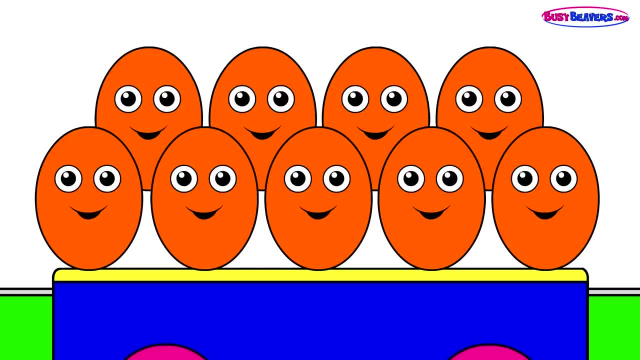 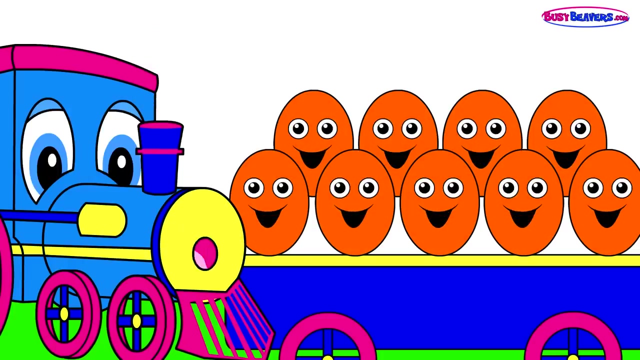 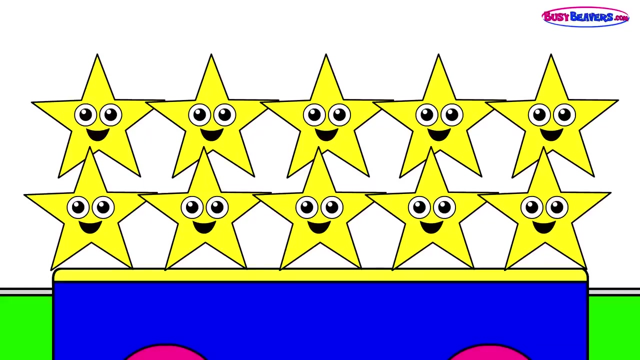 Hearts. I love them. Ovals One, two, three, four, five, six, seven, eight, nine, Nine ovals, Hi, ovals, Hi Steamy Steamer, So round Stars. One, two, three. 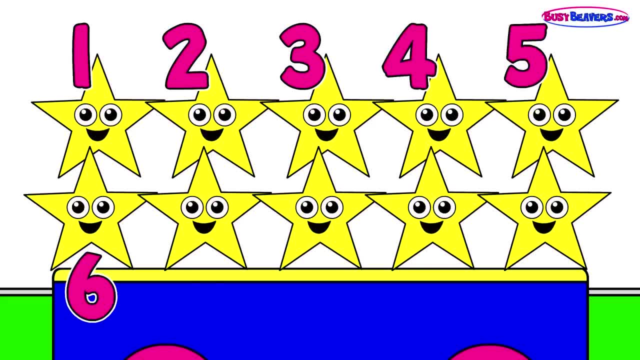 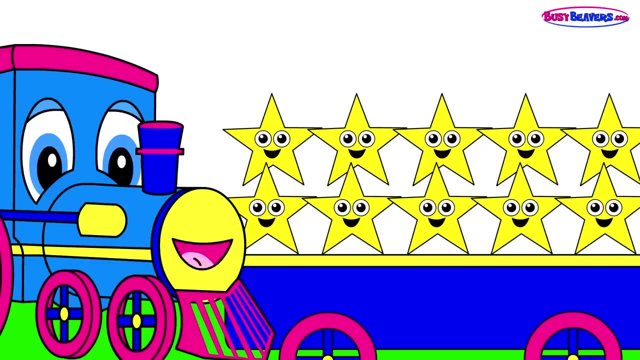 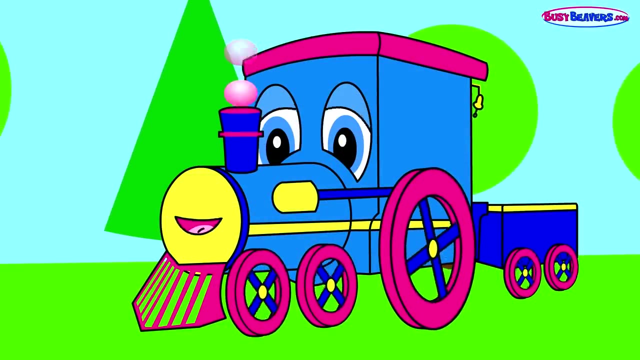 four, five, six, seven, eight, nine, ten Ten stars, Hi, stars Hi. Steamy, Very sparkly, Very twinkly. Well, that's all the shapes for today. Let's count them one more time. 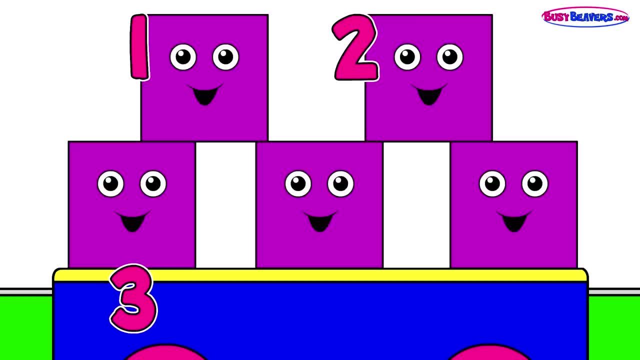 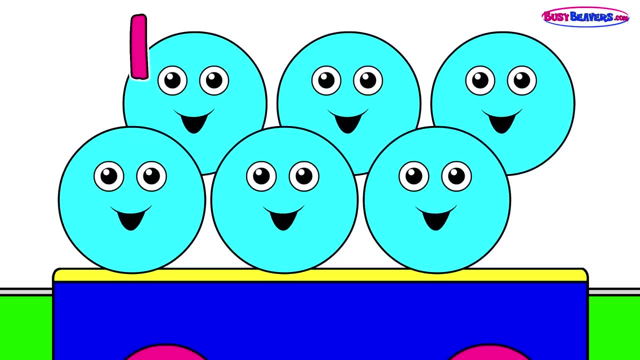 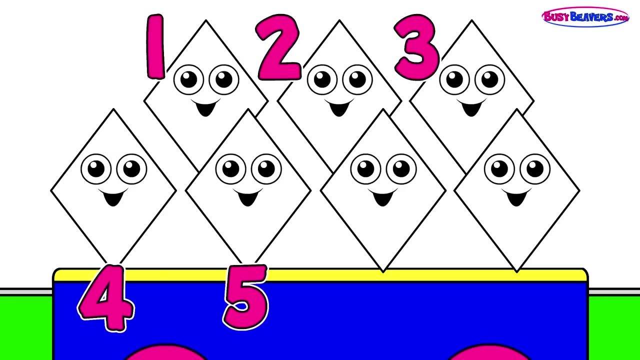 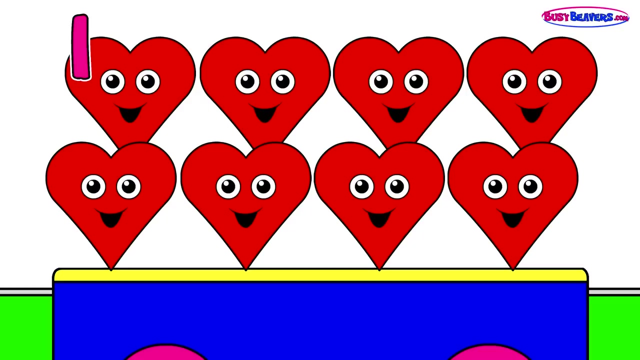 One, two, three, four, five, six, seven, Double two, three, four, five. Oh, it's just like that: Two, three, four, three, two, one, two, three, four. One, two, three, four, five, six, seven, eight hearts. 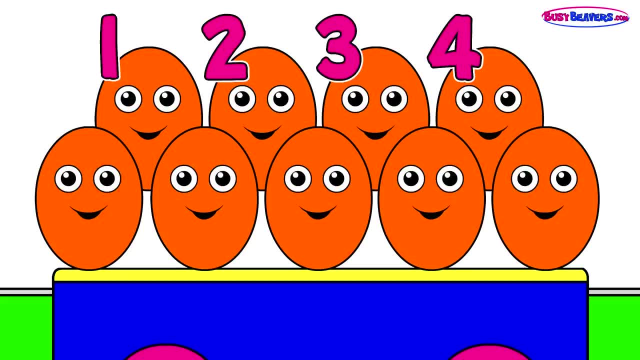 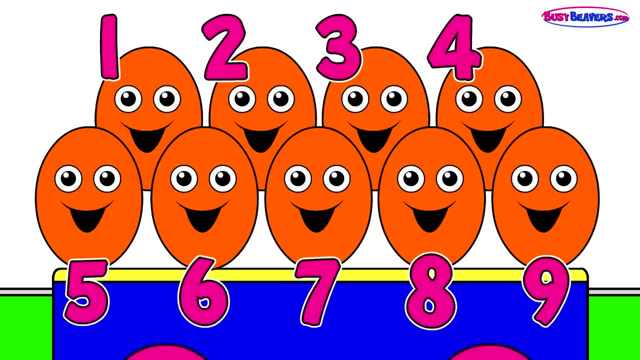 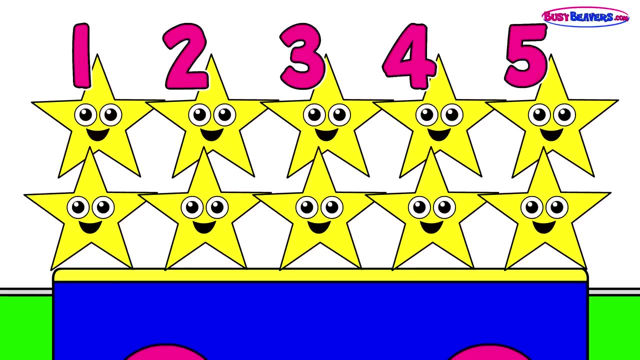 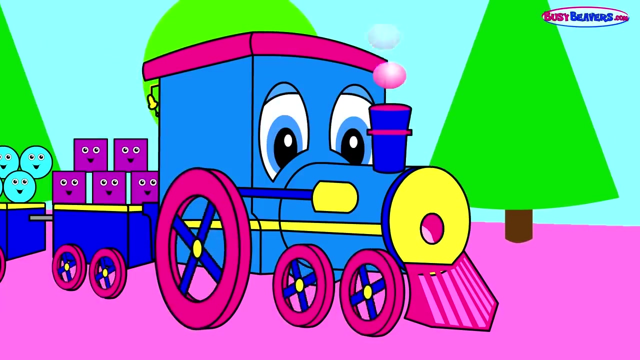 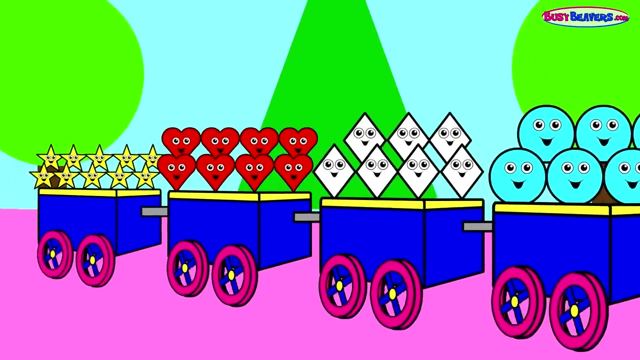 One, two, three, four, five, six, seven, eight, nine ovals. One, two, three, four, five, six, seven, eight, nine, ten stars, All aboard, Here we go. Steamy Steamer, That's my name. 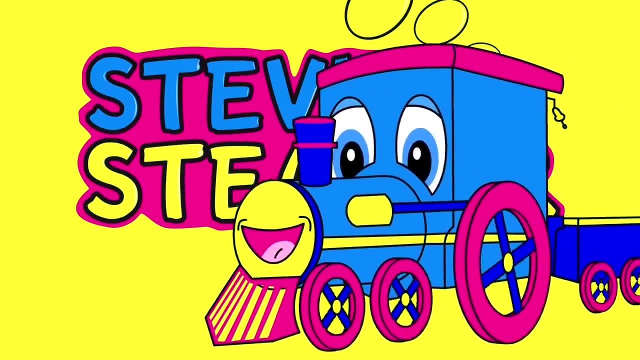 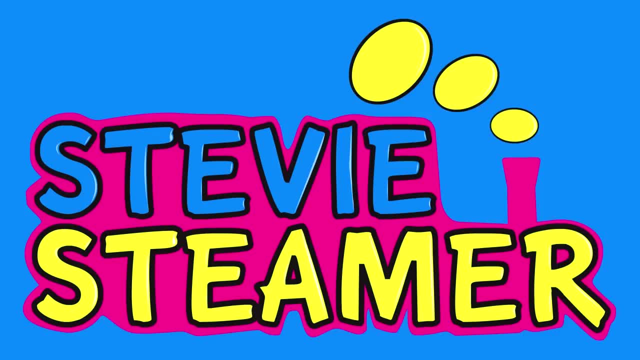 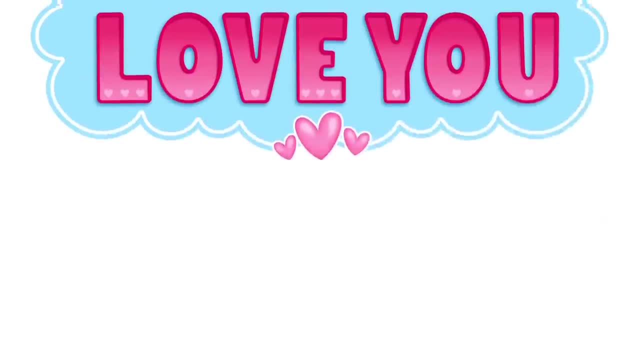 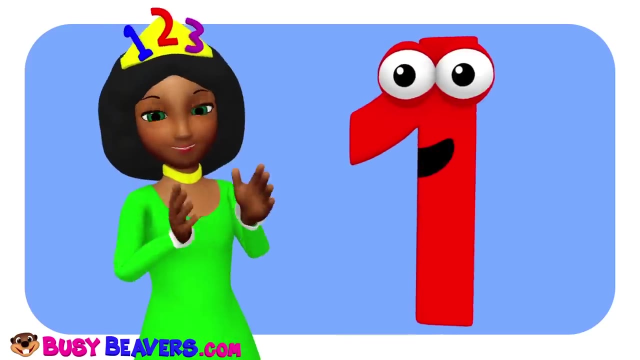 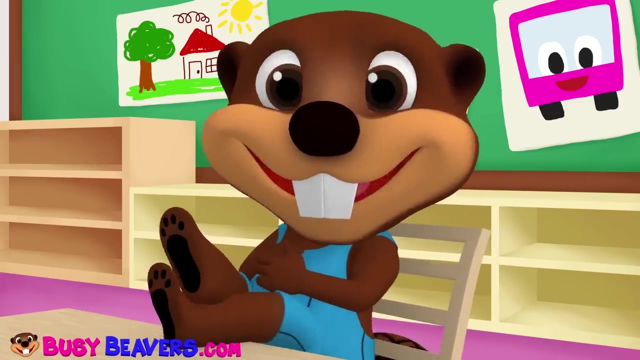 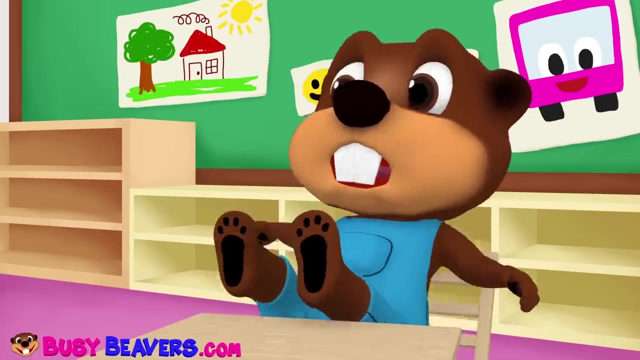 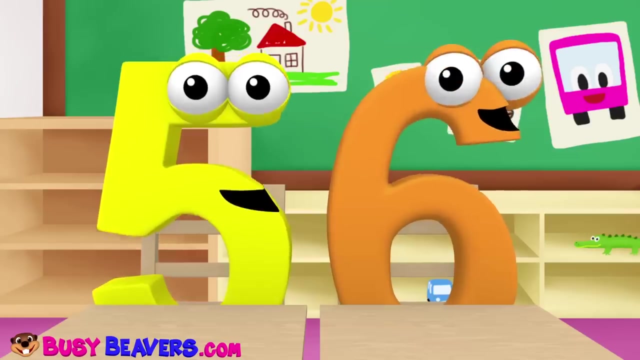 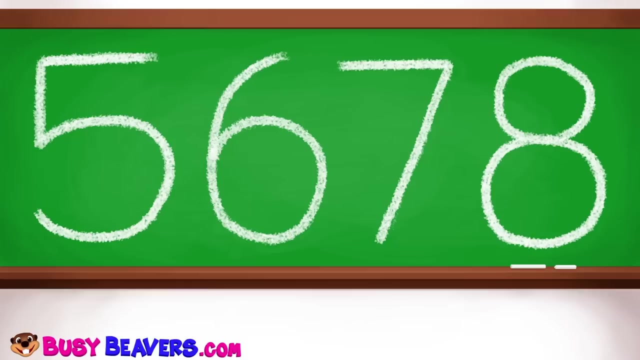 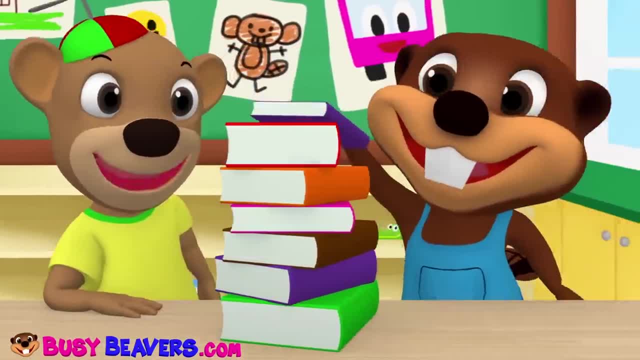 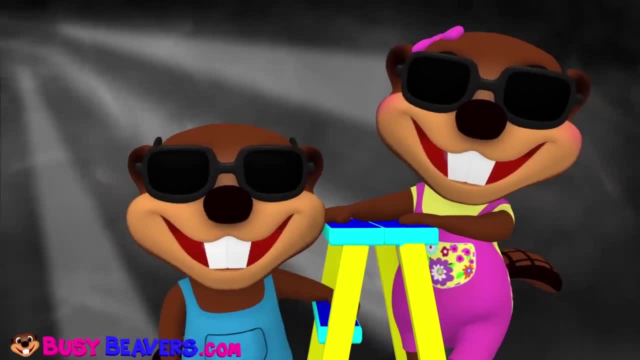 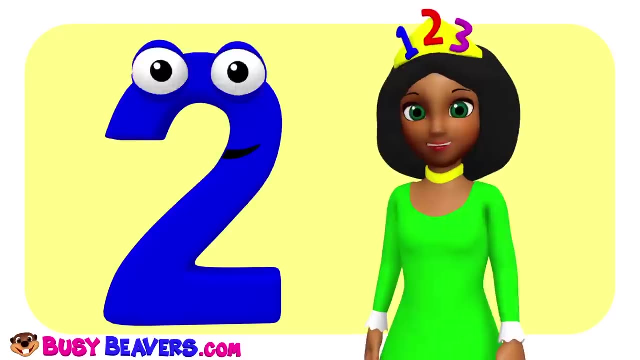 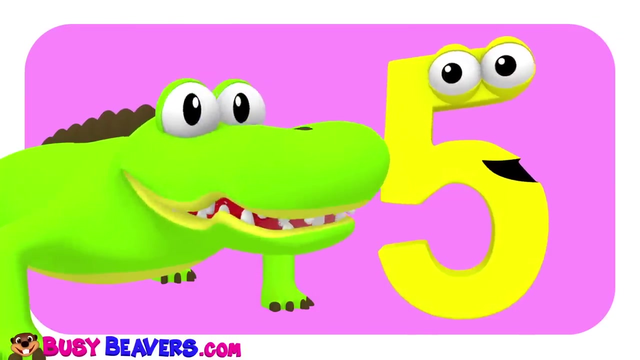 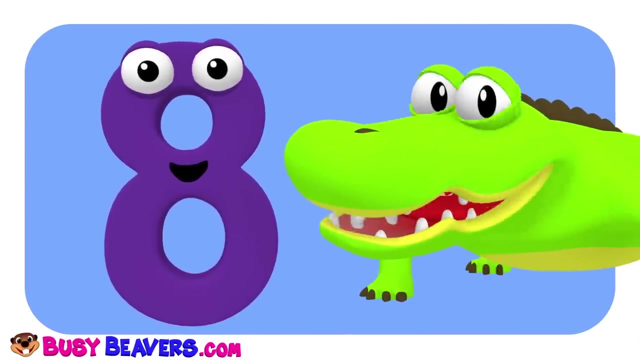 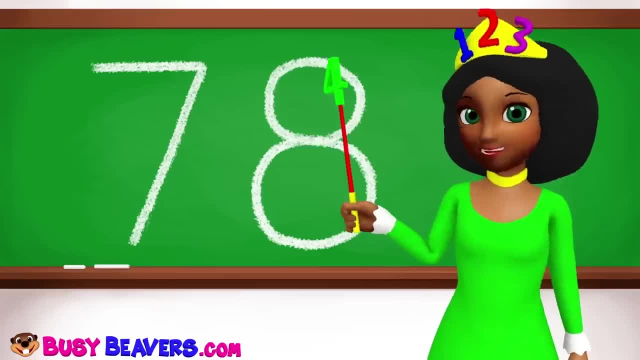 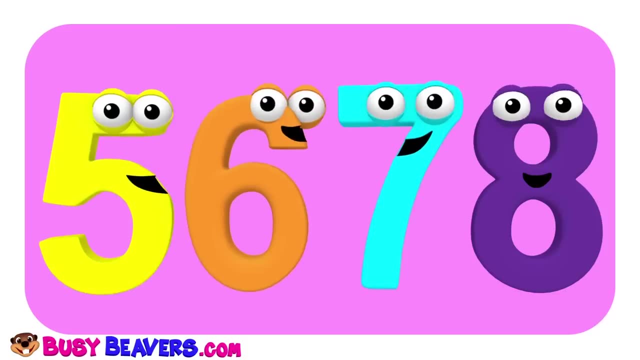 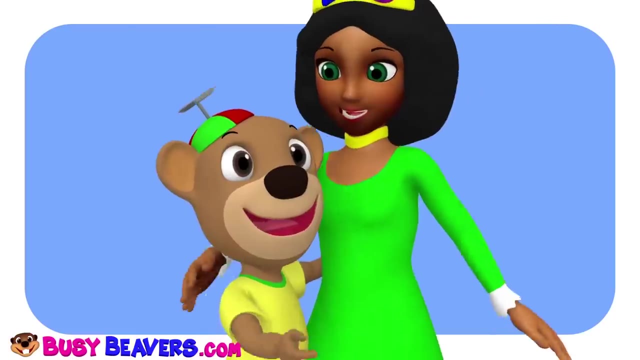 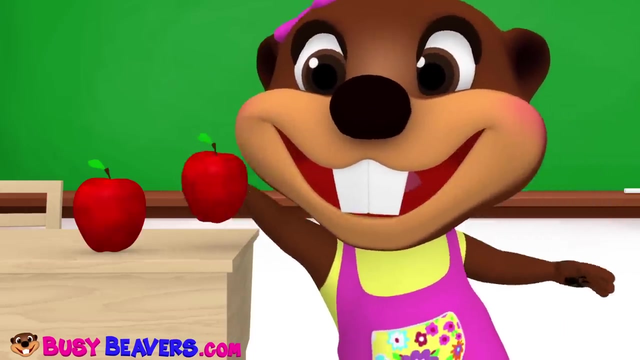 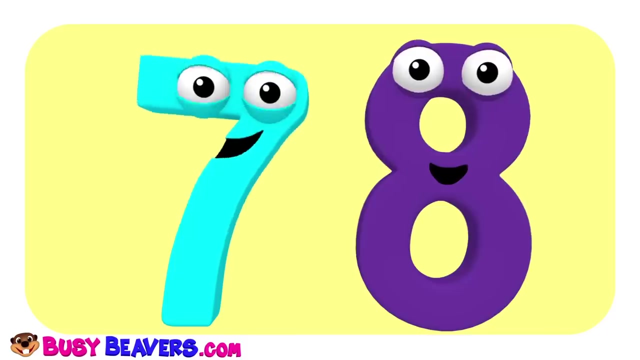 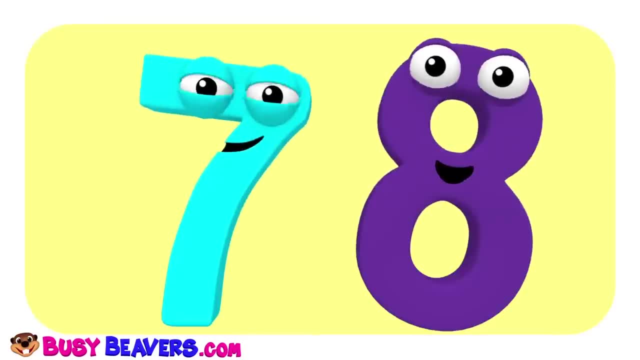 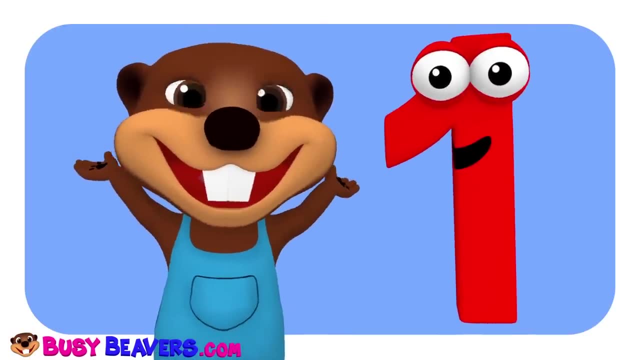 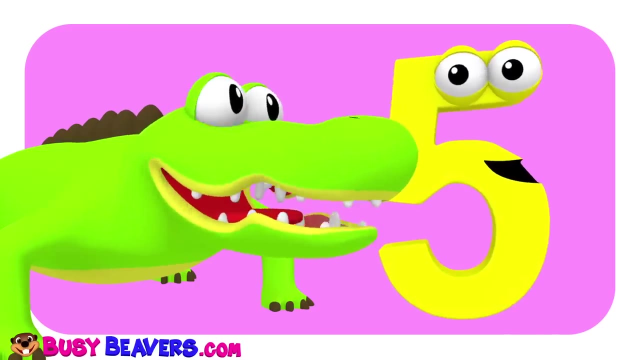 1,, 2,, 3,, 4,, 5,, 6,, 7, 8. 1,, 2,, 3,, 4,, 5,, 6,, 7, 8. 1,, 2,, 3,, 4,, 5,, 6,, 7, 8. 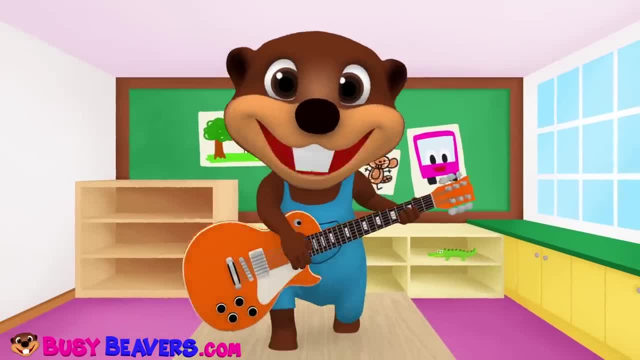 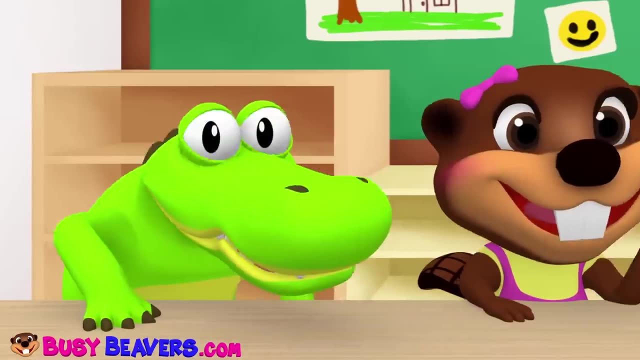 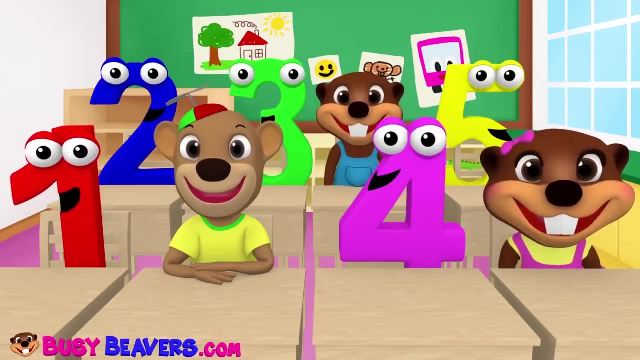 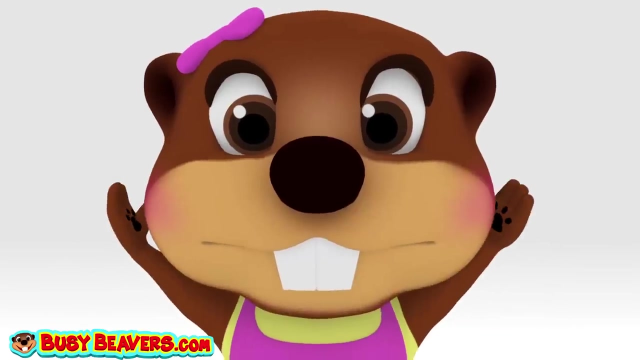 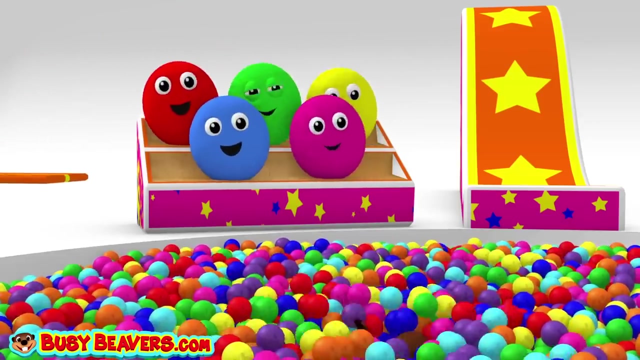 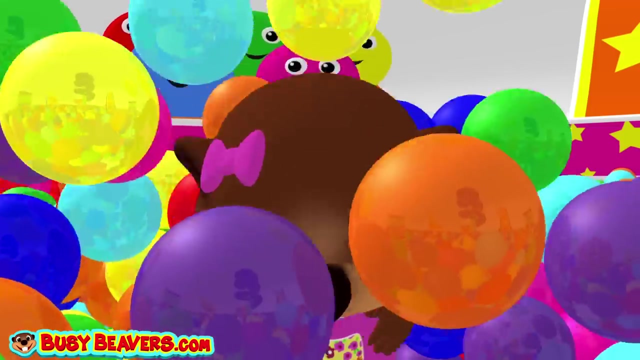 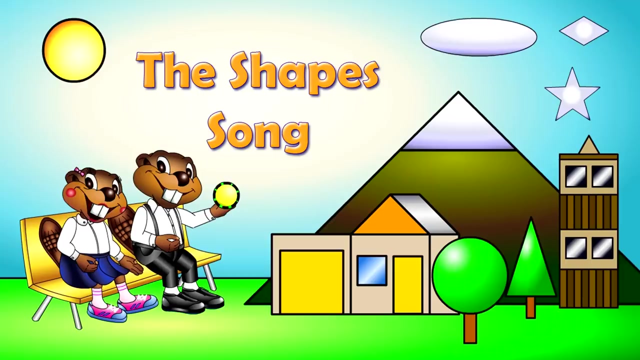 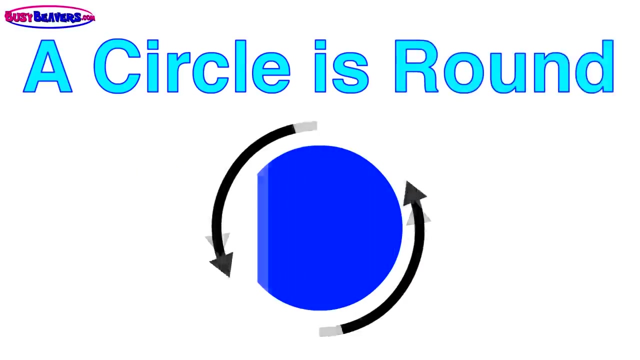 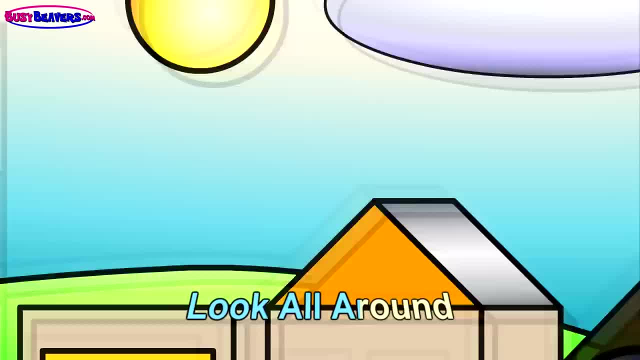 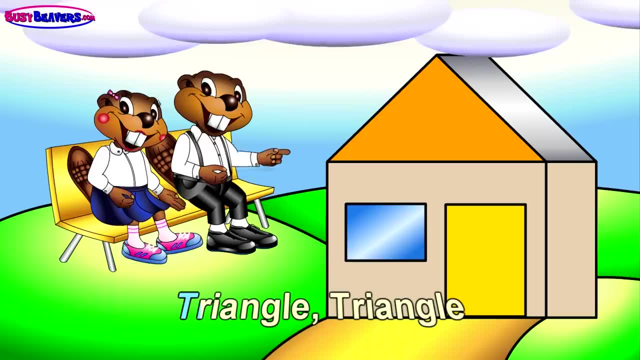 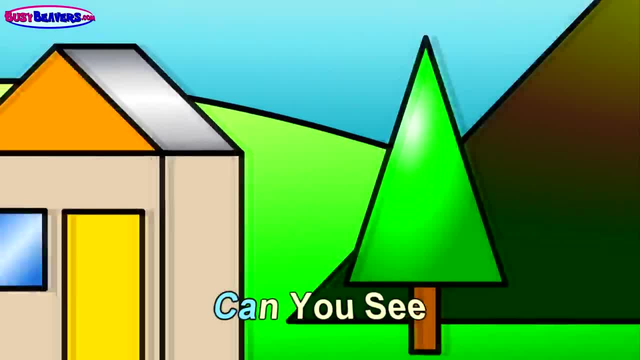 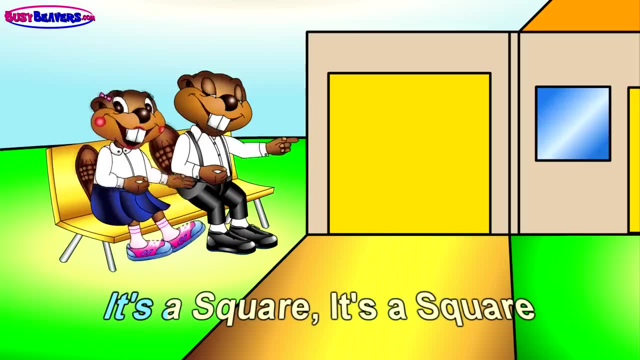 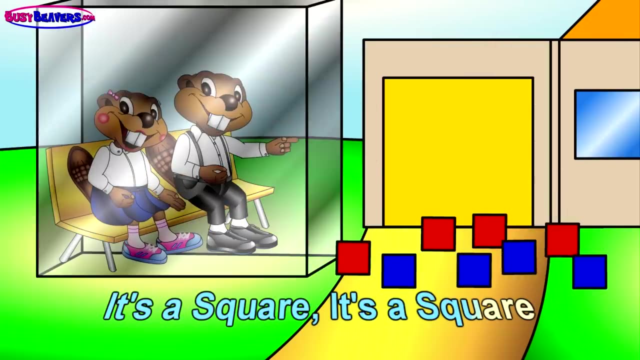 Look all around you can you see triangles. It's a square. it's a square 1,, 2,, 3,, 4. It's a square. it's a square 1,, 2,, 3,, 4. 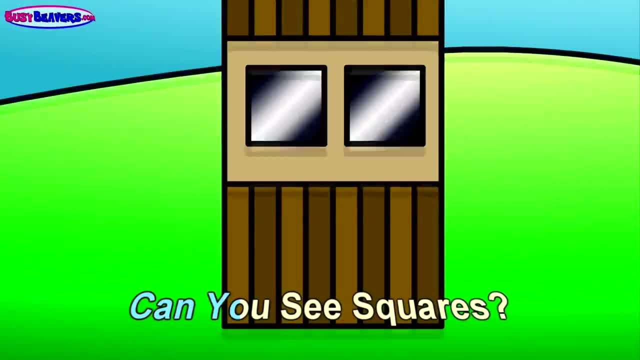 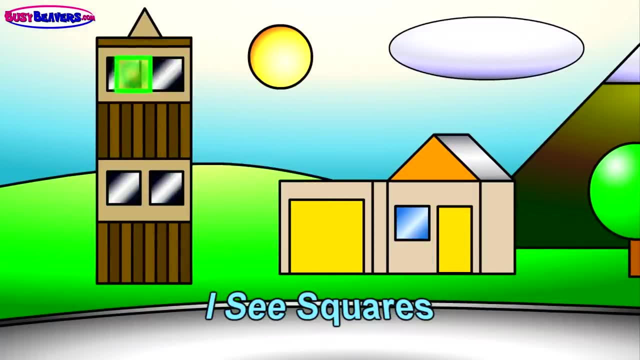 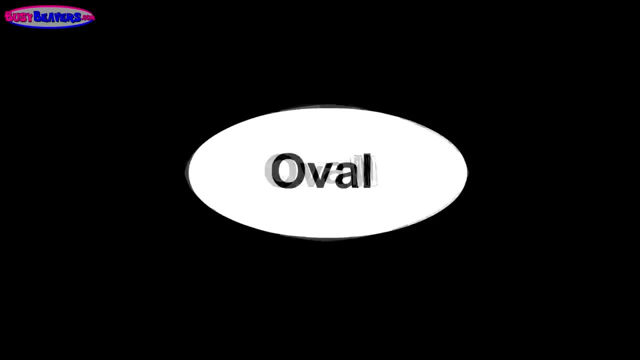 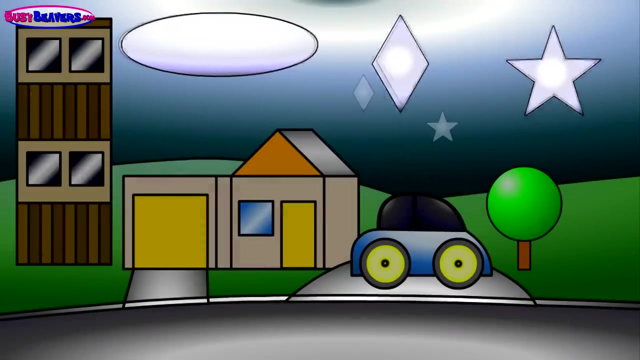 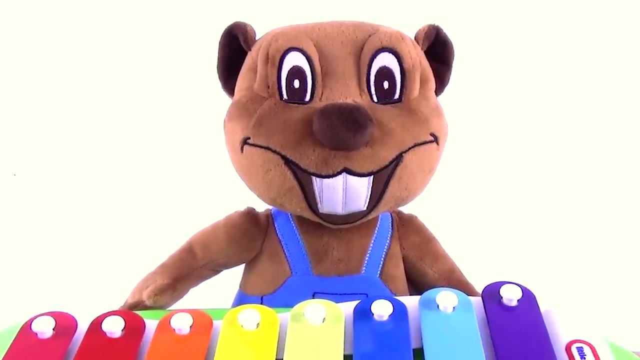 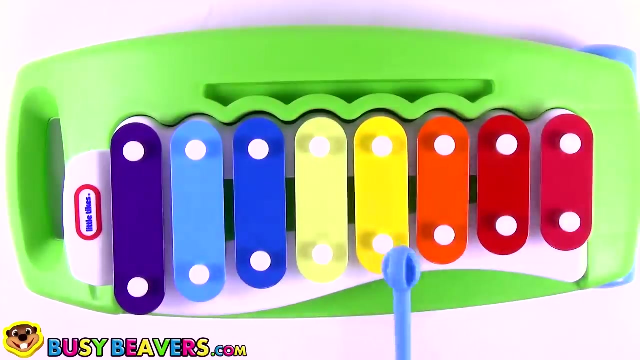 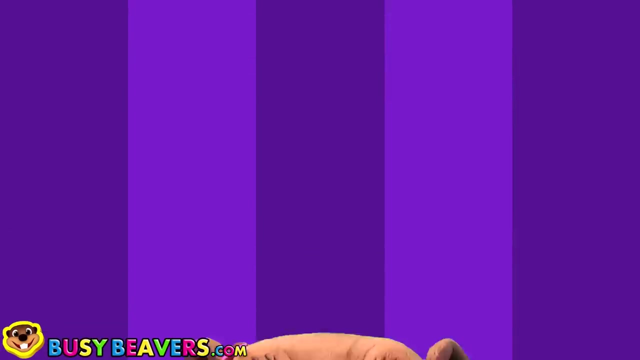 Look over there. can you see these squares? I see squares. Rectangle oval diamond star. Rectangle oval diamond star. Rectangle oval diamond star. Let's play team briefing. Rectangle oval diamond star. Rectangle oval diamond star. 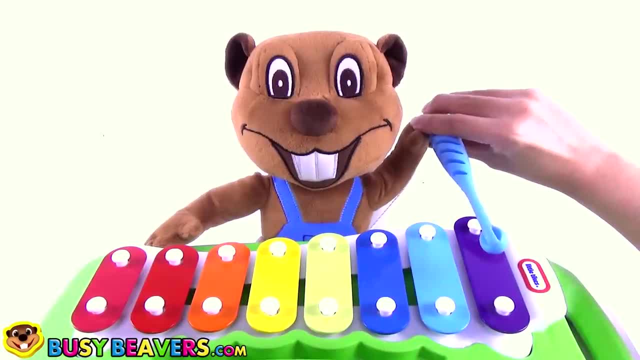 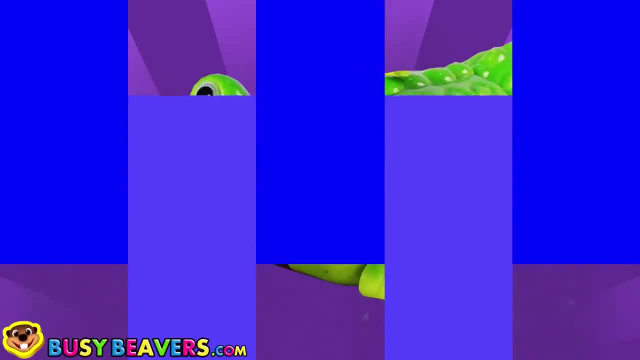 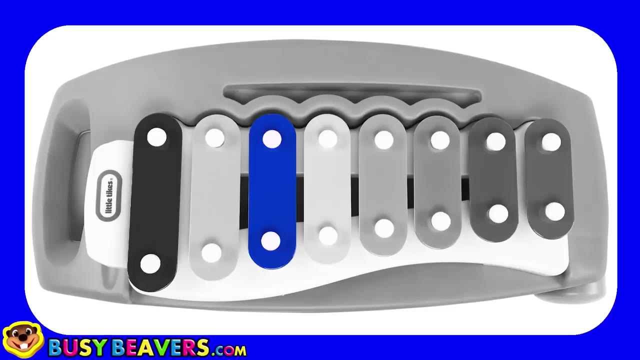 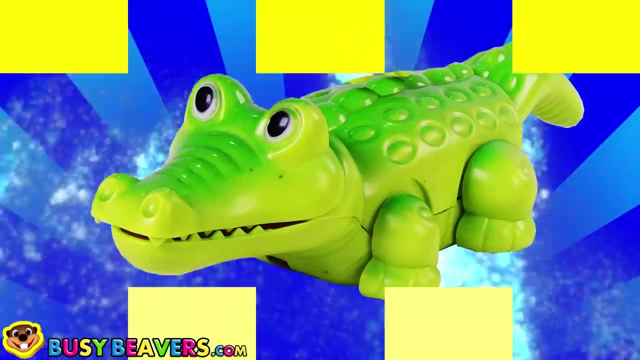 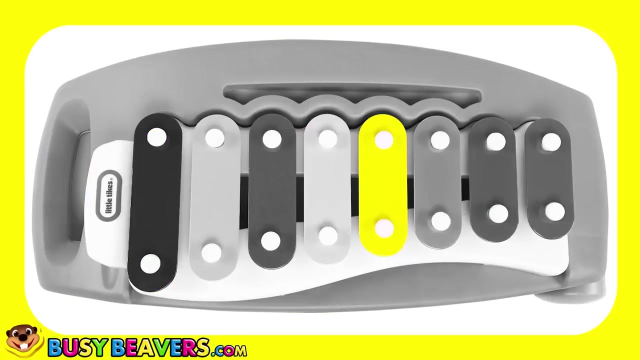 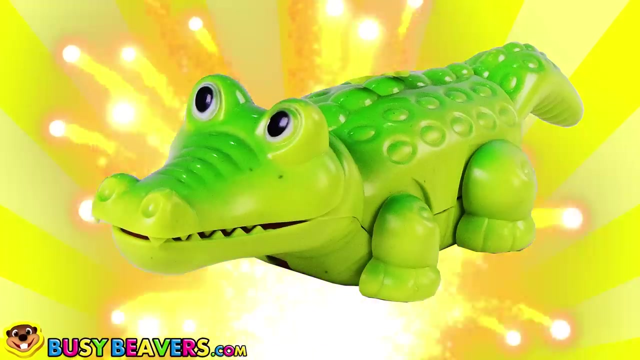 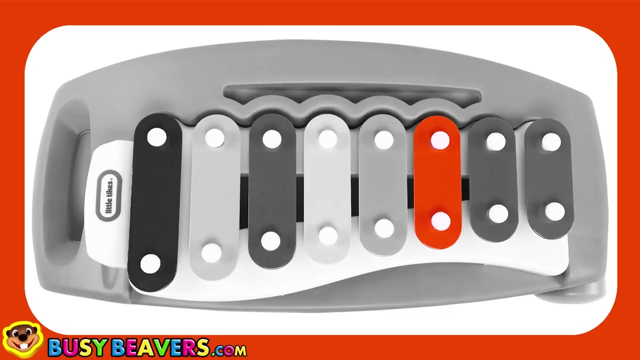 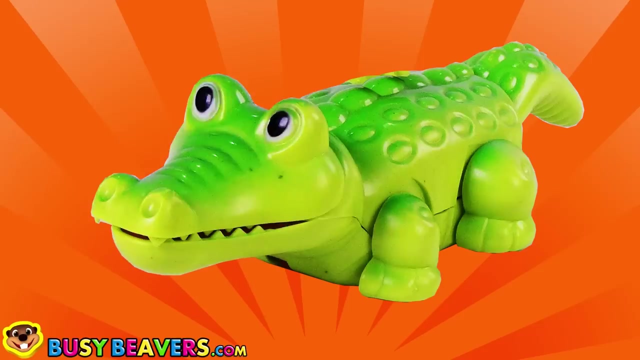 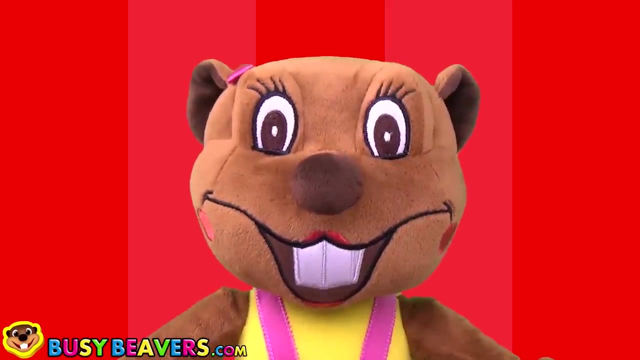 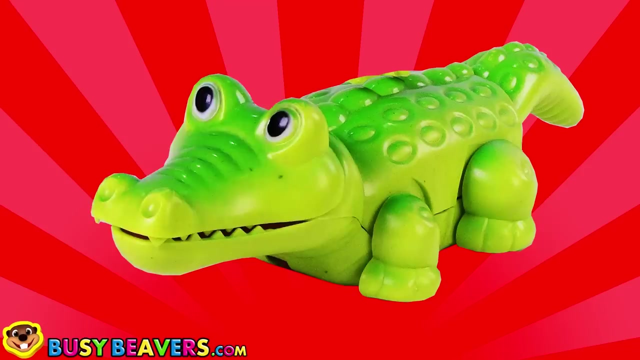 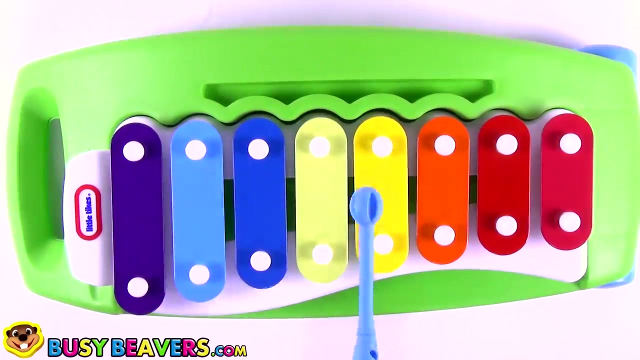 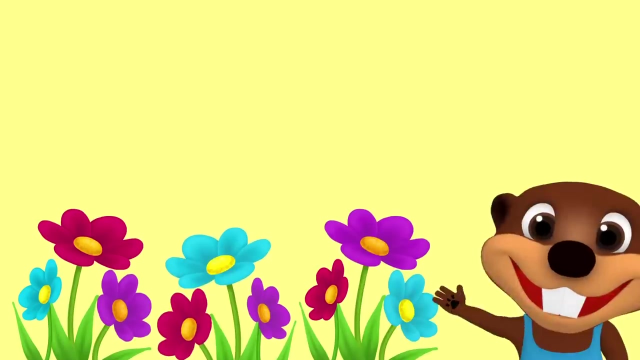 Rectangle- oval diamond star Rectangle, Rectangle, oval diamond star, Rectangle, Rectangle. seva cru asına wears 100 blue rupa rupa, blue rupa, blue, Blue, Blue, Yellow, Yellow, Yellow, Orange, Orange, Orange, Red, Red, Red, Yellow. Can you sing the alphabet backwards? 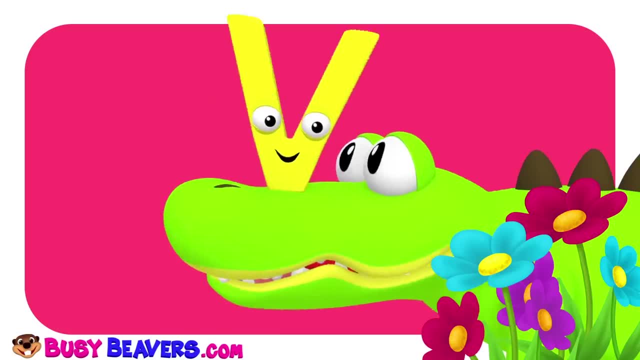 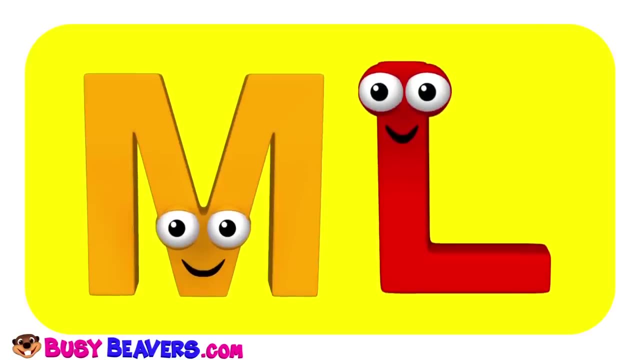 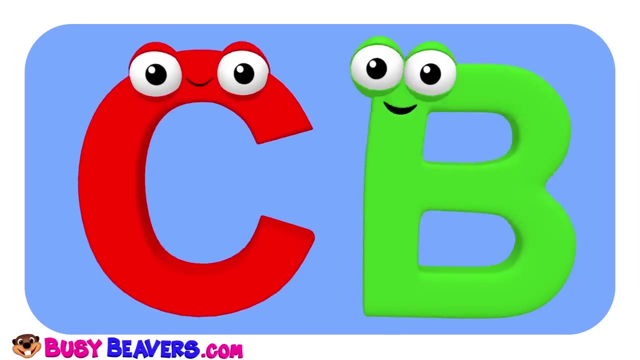 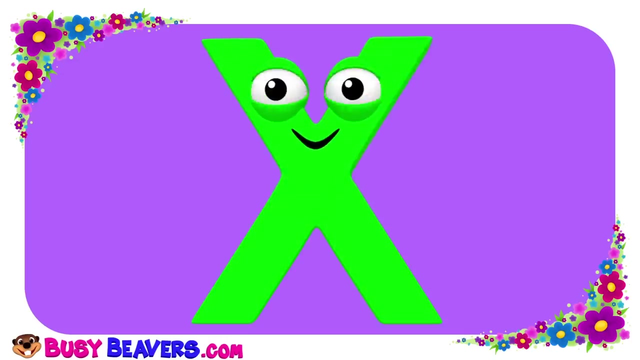 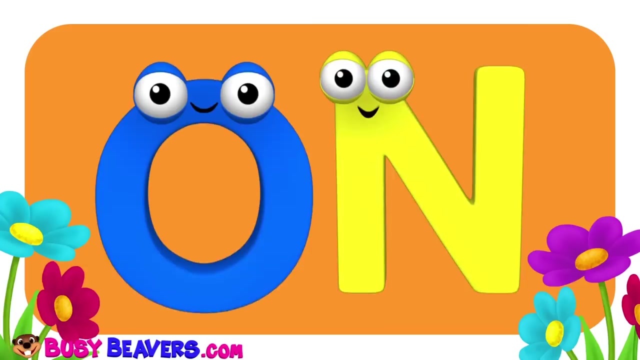 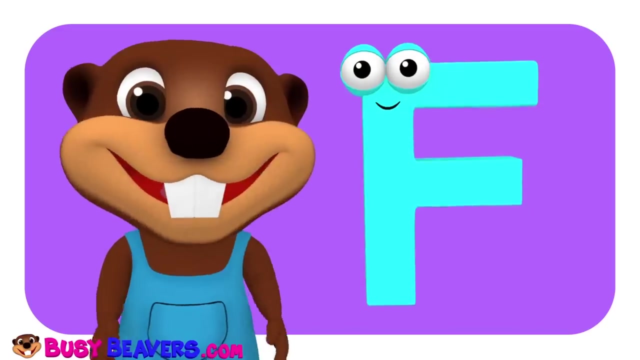 C-Y-X-W-V-U-T-S-R-Q-P-O-N-M-L-K-J-I- H-G-F-E-D-C-B-A Again. C-Y-X-W-V-U-T-S-R-Q-P-O-N-M-L-K-J-I- H-G-F-E-D-C-B-A. 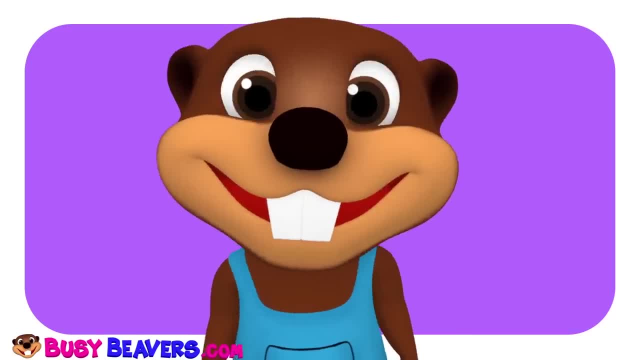 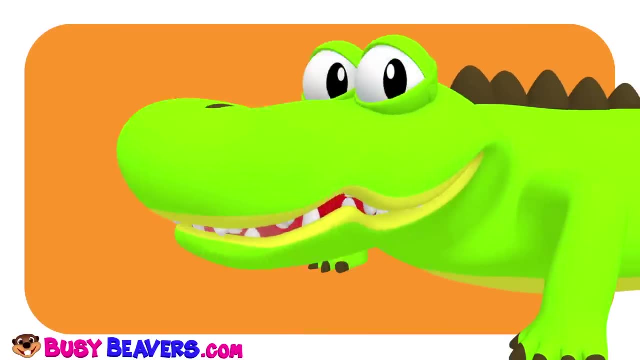 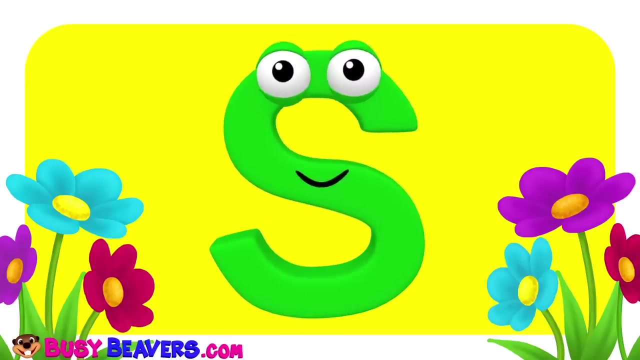 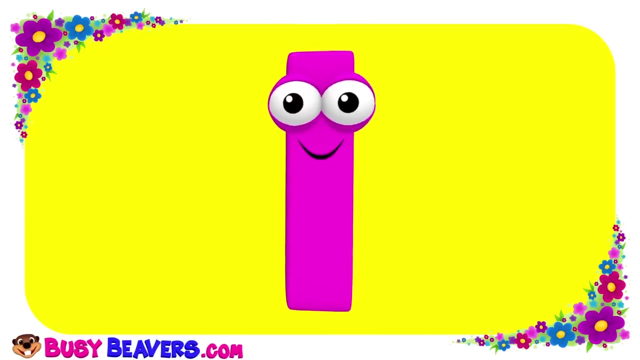 Again. C-Y-X-W-V-U-T-S-R-Q-P-O-N-M-L-K-J-I. Can you do it? It's not easy. I'm gonna do it this time. Here I go. C-Y-X-W-V-U-T-S-R-Q-P-O-N-M-L-K-J-I. 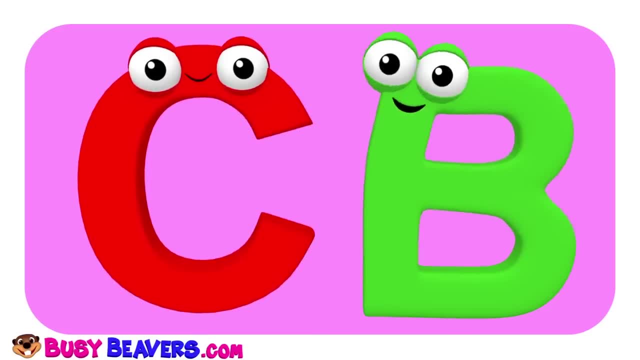 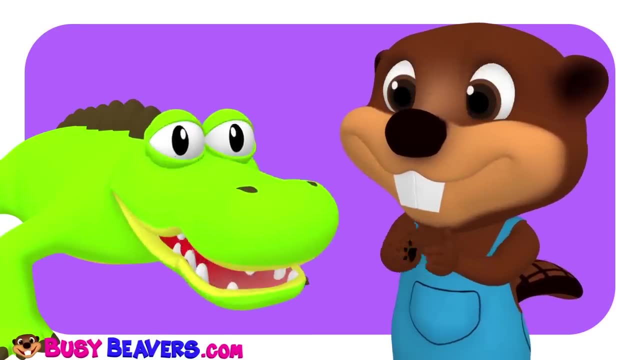 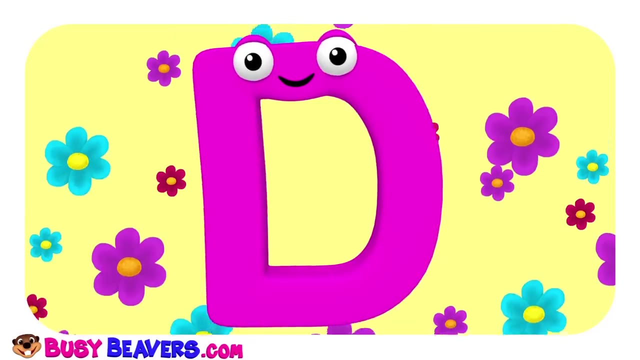 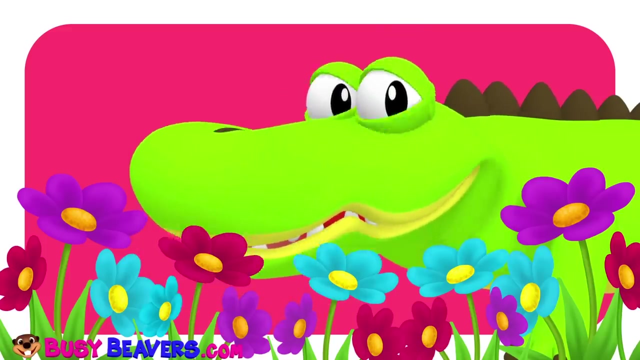 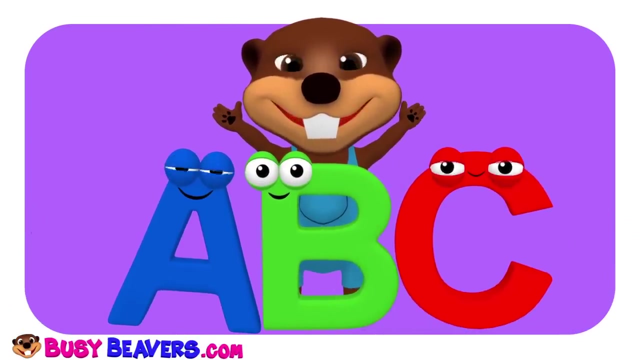 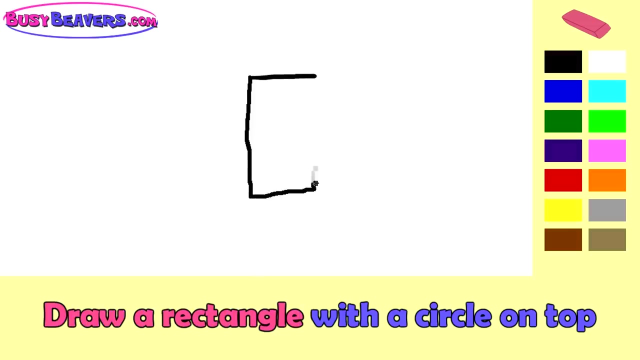 H-G-F-E-D-C-B-A, H-G-F-E-D-C-B-A, H-G-F-E-D-C-B-A. Oh, I did it. Did you hear me? I did it. I did it. good too, Draw a rectangle with a circle on top. Two arms, two legs. 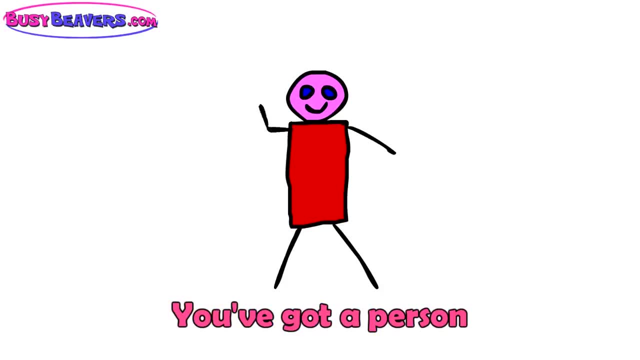 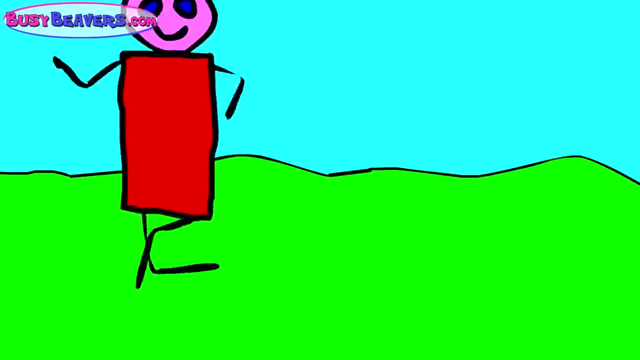 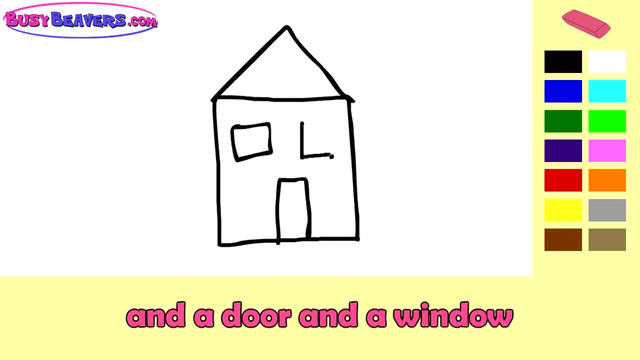 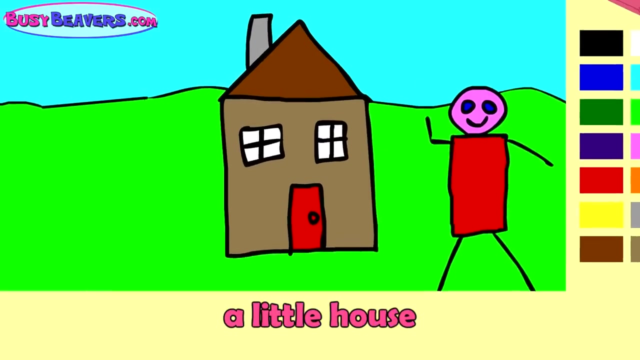 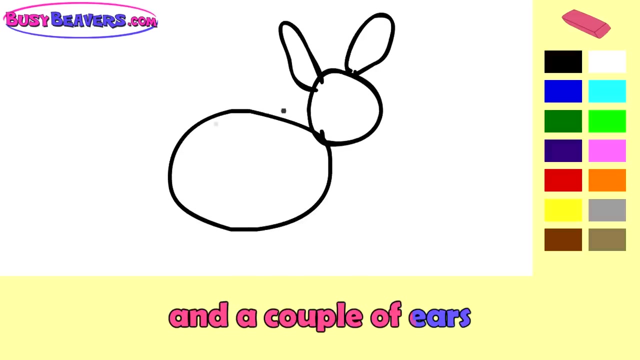 What have you got? You've got a person, A happy person. Draw a square with a triangle top And a door and a window. Hey, what have you got? You've got a house, A little house. Draw an oval and a circle and a couple of ears. 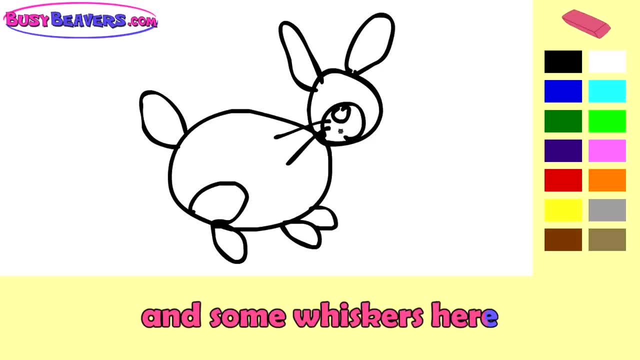 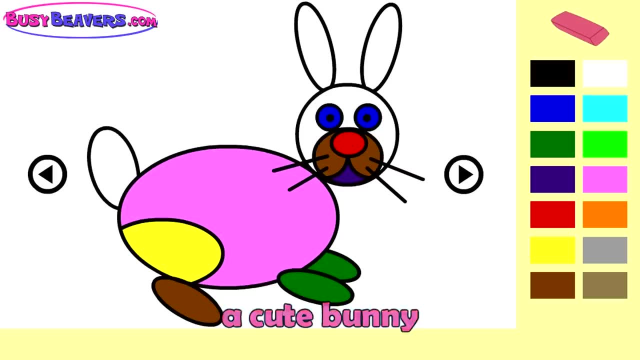 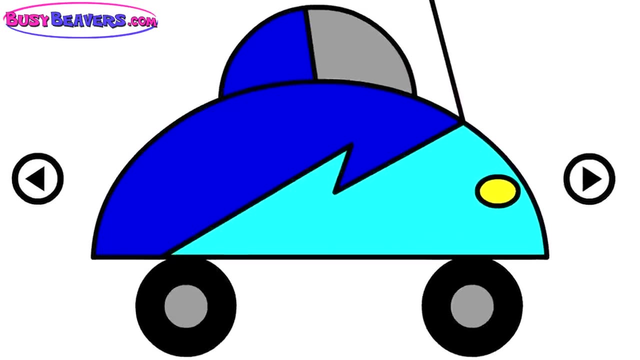 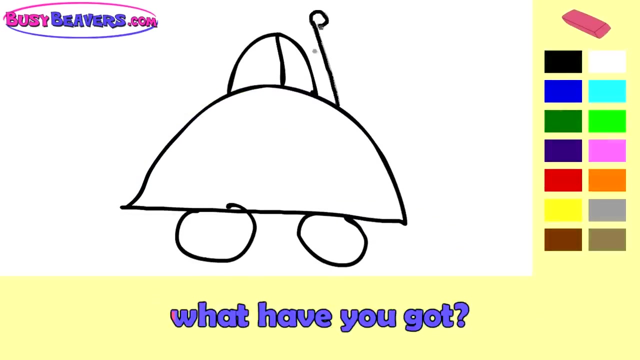 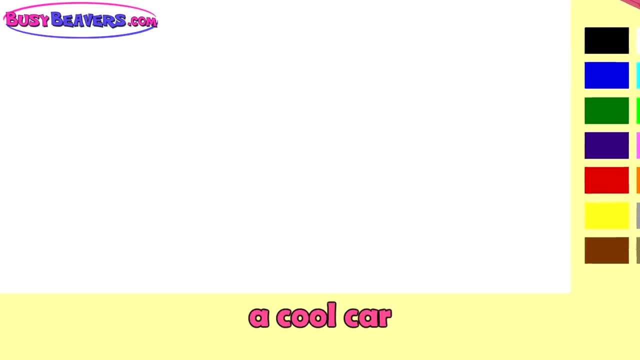 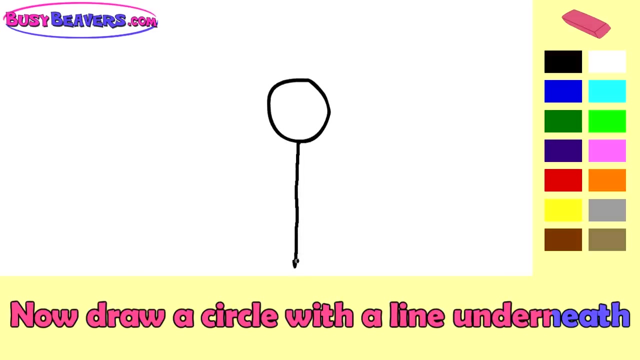 A tail, feet, a face and some whiskers. here You've got a bunny. Look at that, A cute bunny. Draw a half circle with another on top, Giving wheels and windows. Hey, what have you got? You've got a car, A cool car. Now draw a circle with a line underneath A bunch of ovals, four petals and two four leaves. 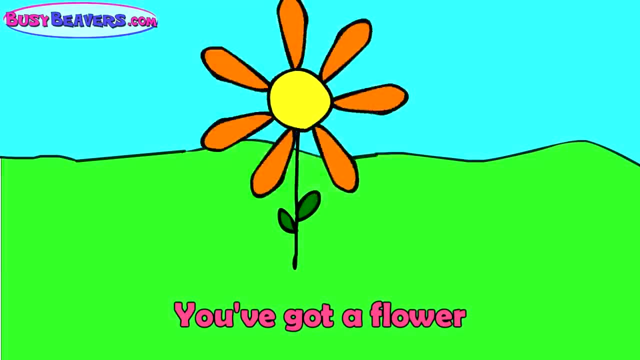 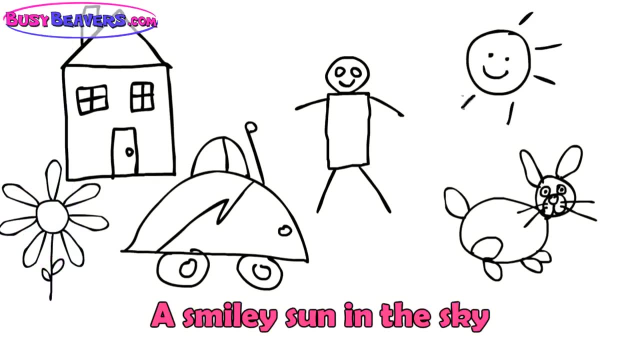 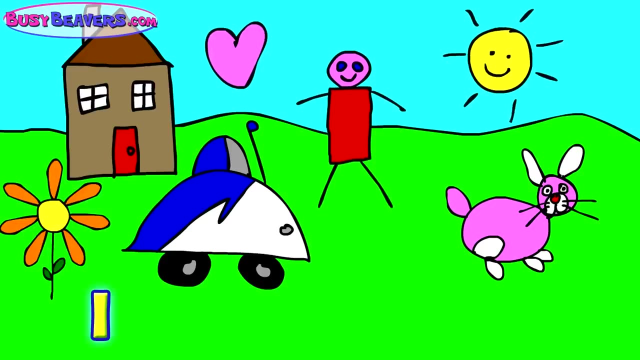 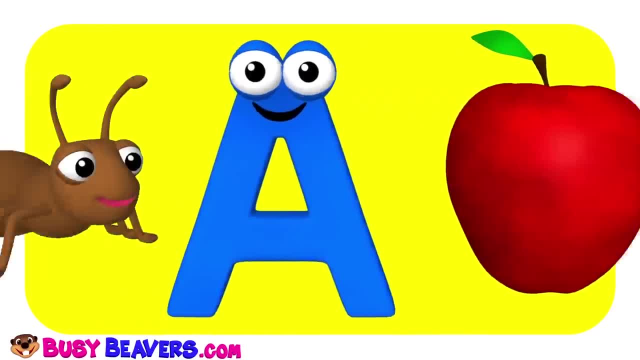 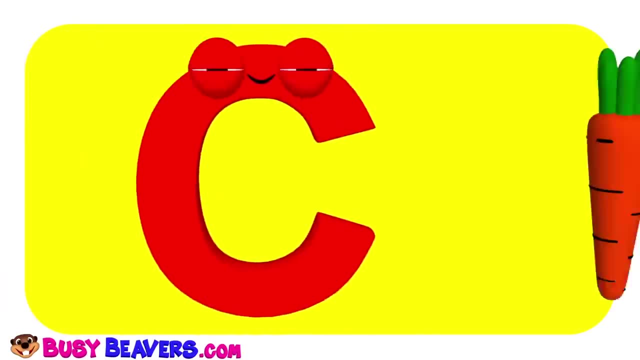 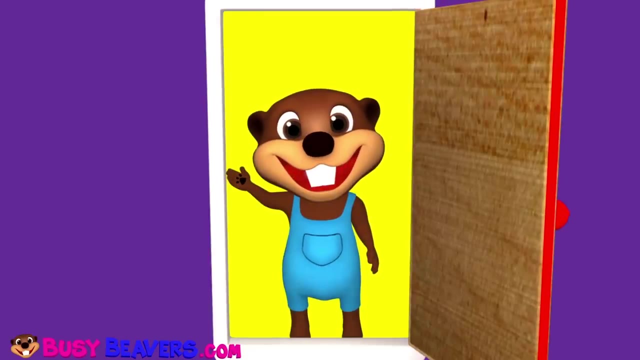 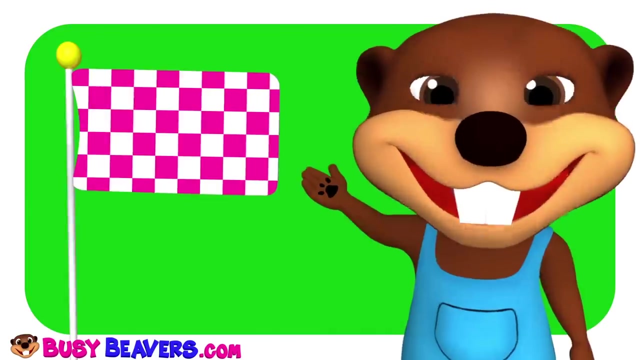 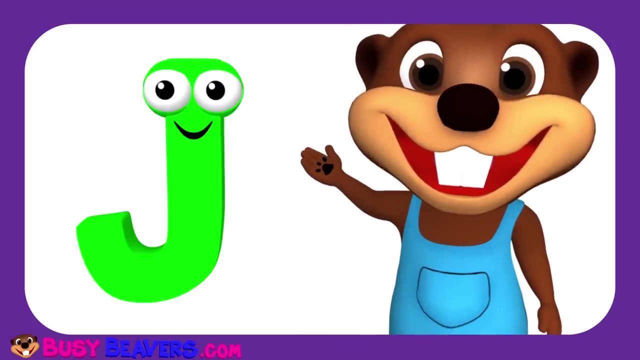 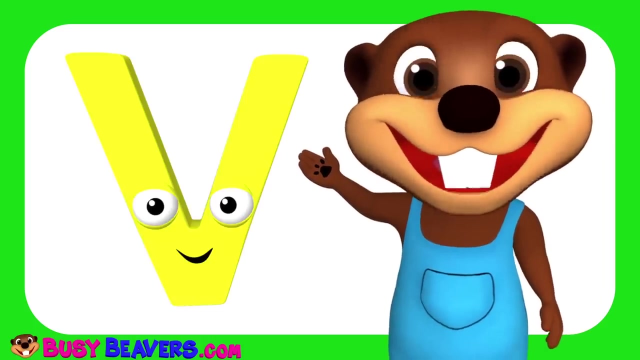 Here we go: A a apple, A a ant, B a ball, B a bat, C a carrot, C a car, D a duck, D a door, E a elevator, E a egg, F a fish, F a flag, A, B, C, D, E, F, G, H, I, J, K, L, M, N, O, P, Q, R, S, T, U, V, W, X, Y and Z. 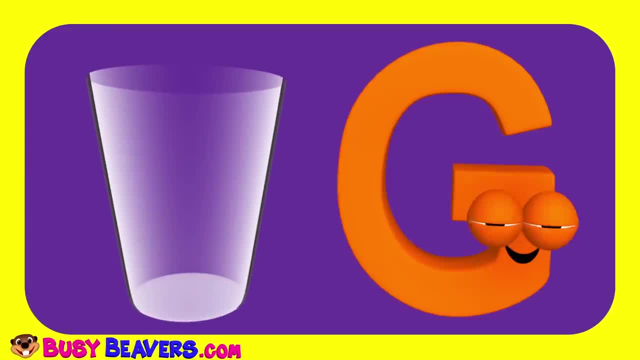 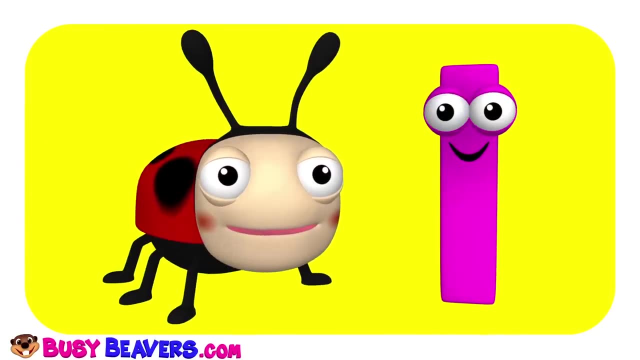 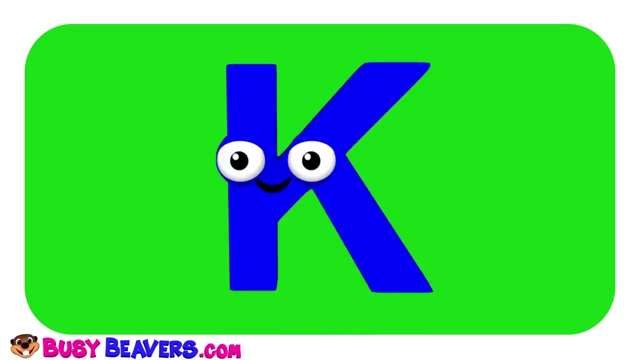 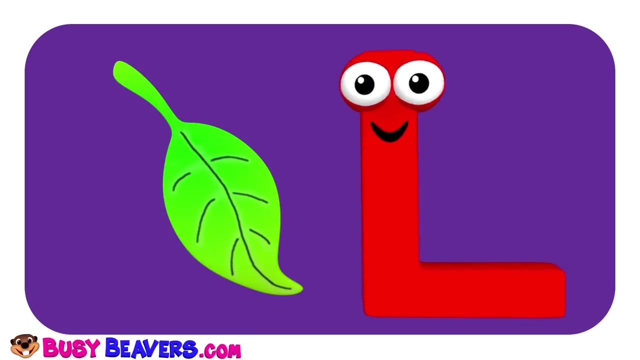 G a guitar, G a glass, H a hammer, H a hat I I insect, I I glue, J a jam, J a juice, K a kangaroo, K a key, L a ladder, L a leaf. 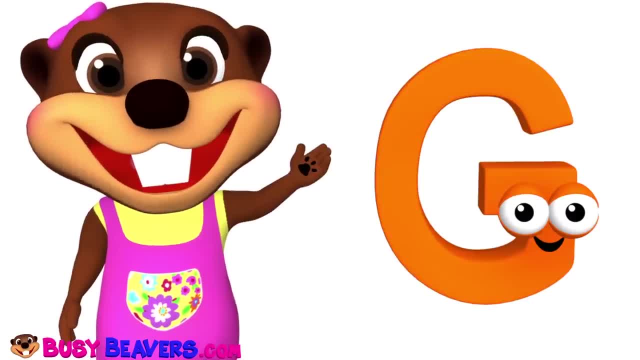 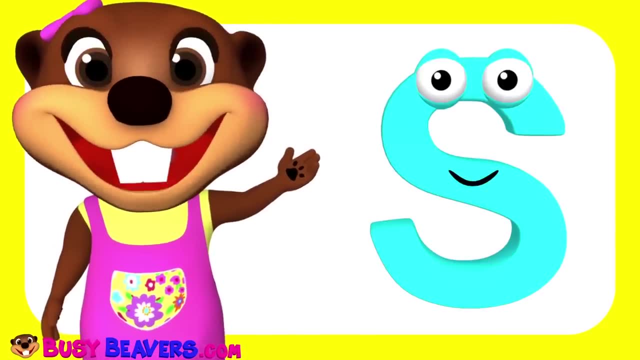 A B C D E F, G A B C D E F, G A B C D E F G H, I, J, K, L, M, N, O, P, Q, R, S, T, U, V, W, X, Y and Z. 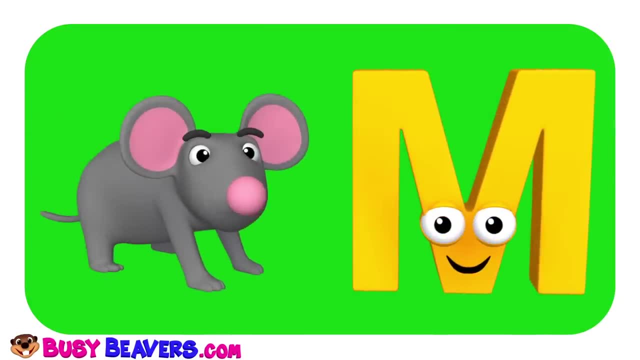 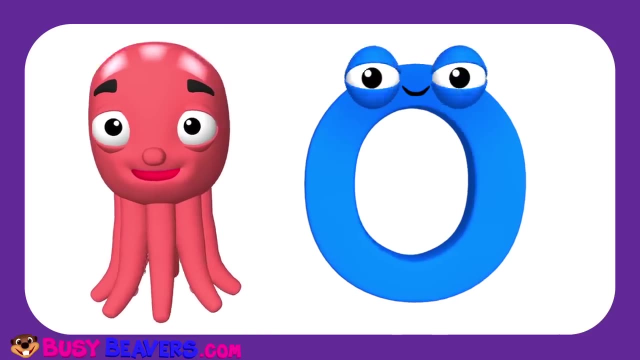 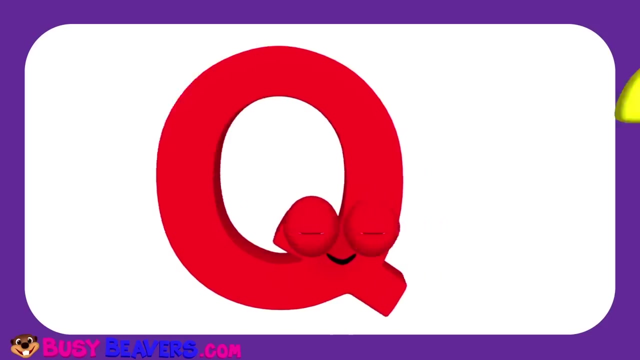 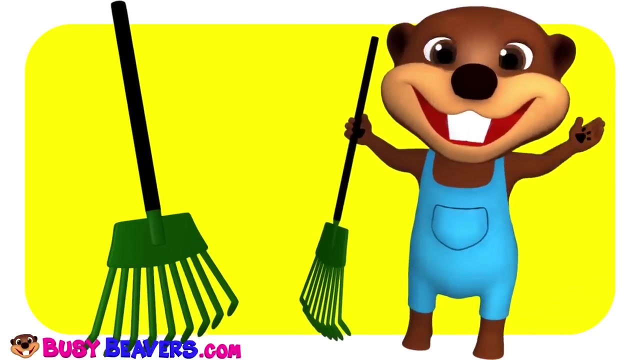 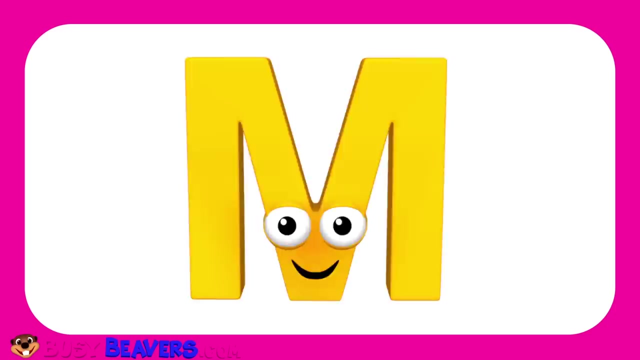 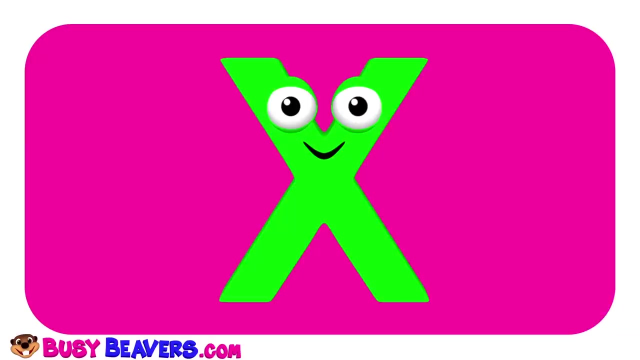 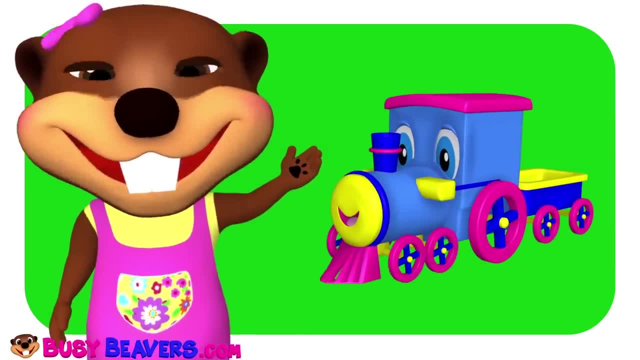 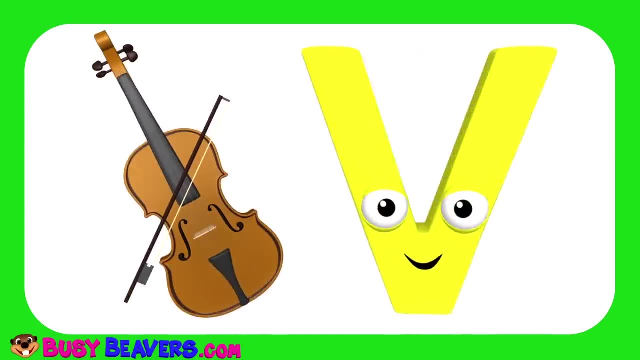 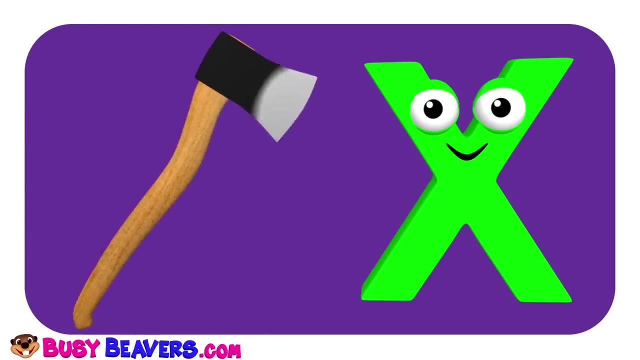 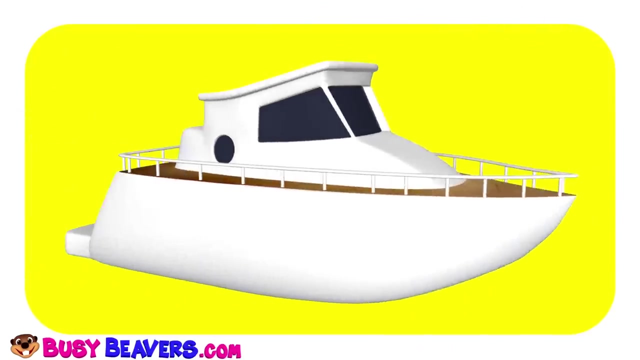 T-touch tree, T-touch train, U-a-umbrella, U-unicorn, V-a-vacuum, V-violin, W-a-whale, W-a-watch, X-axe, box, fox, Y-a-yo-yo, Y-a-yacht, Z-a-zipper, Z-zebra. 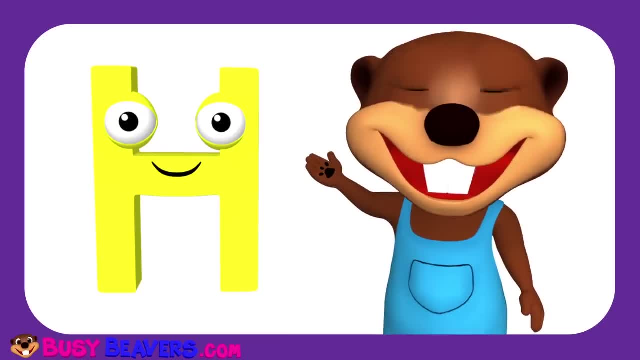 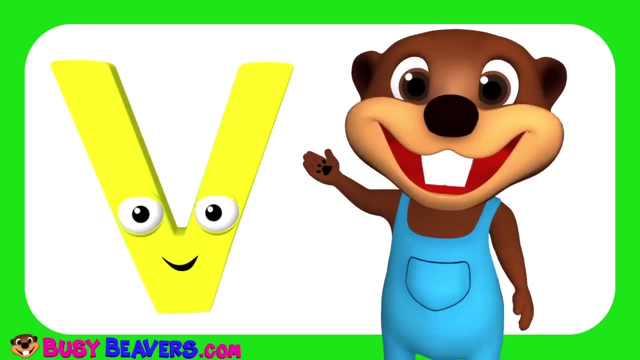 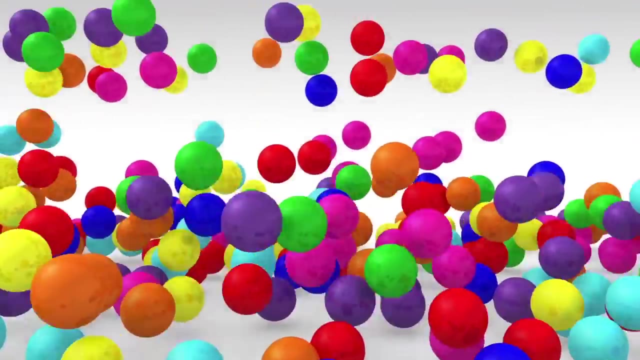 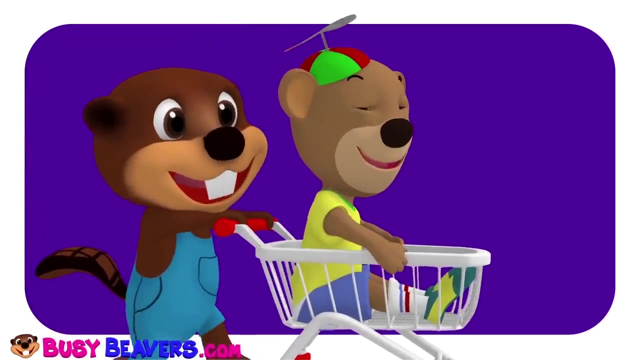 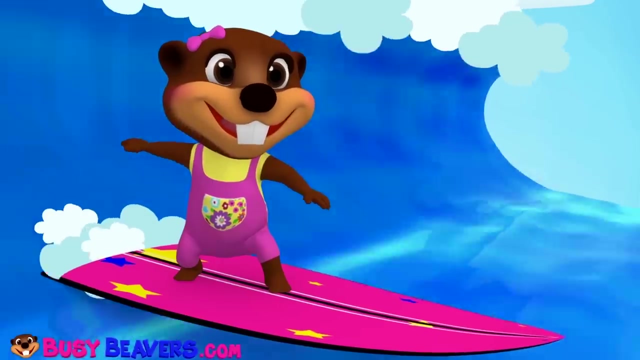 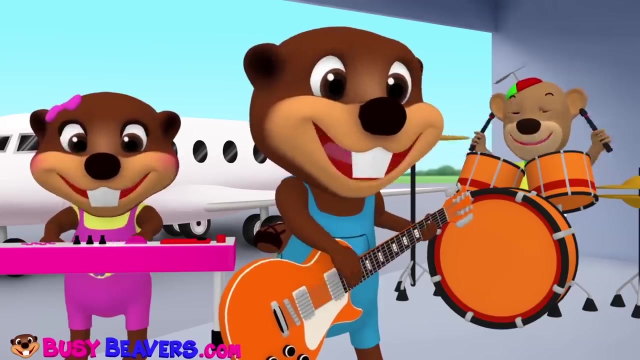 P-c-d-e-f-g, H-i-j-k-l-m-n-o-p, U-r-s-t-u-v, W-x-y-n-t. I love the Busy Beavers TV show. I love the Busy Beavers TV show. One, two, three, four. here we go. 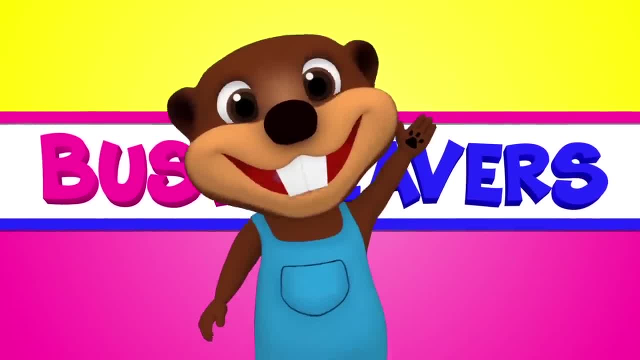 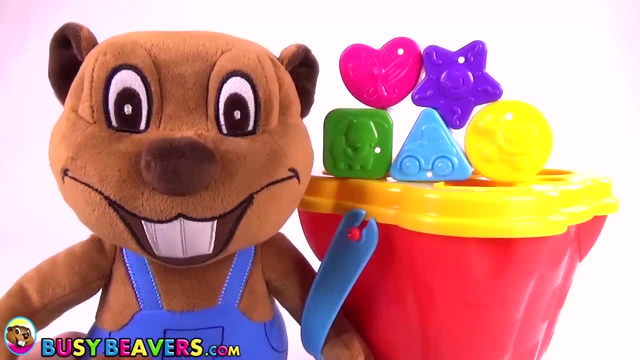 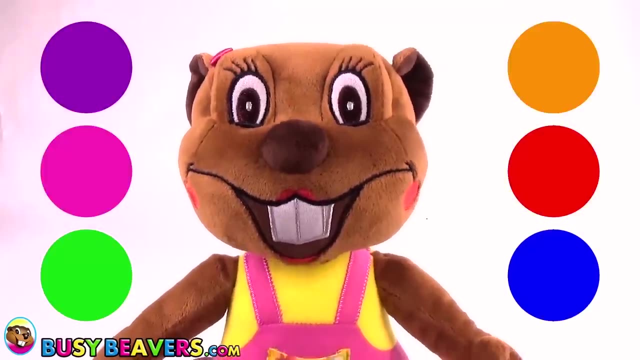 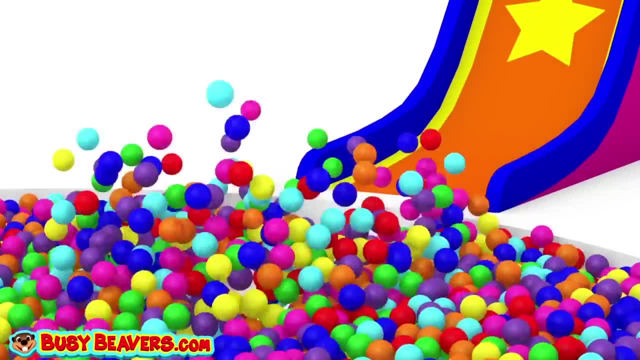 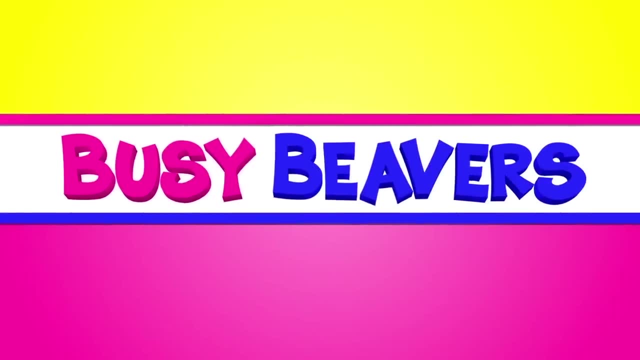 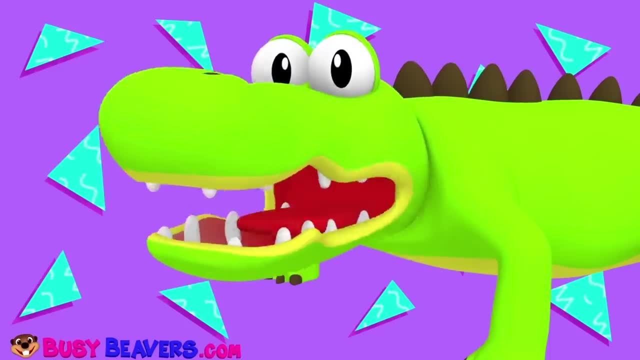 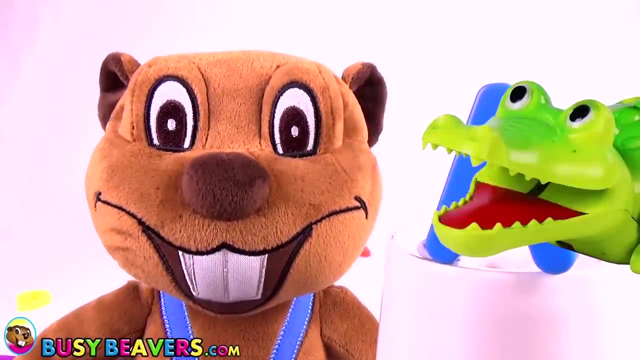 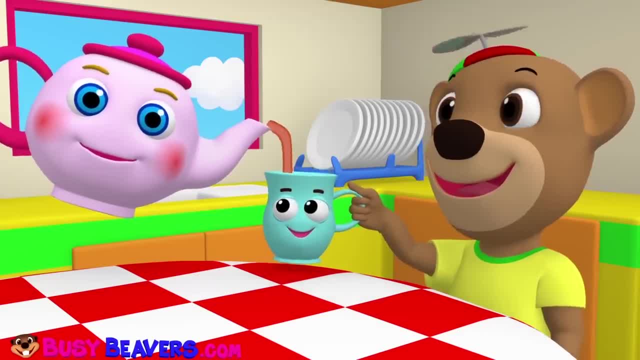 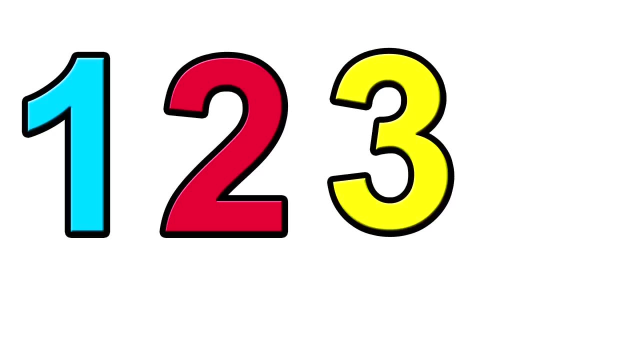 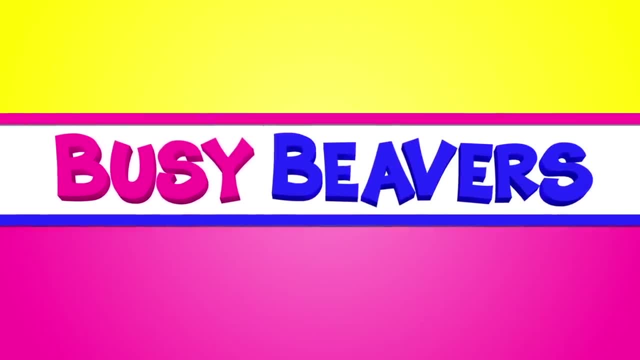 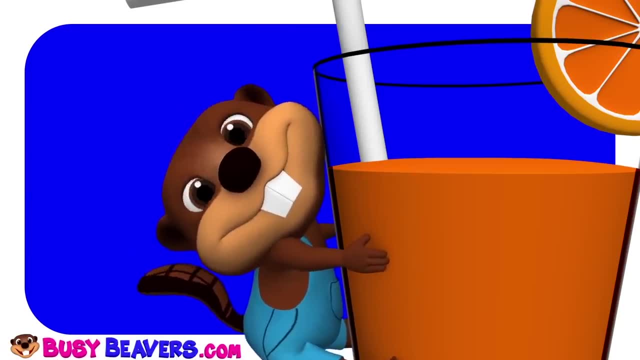